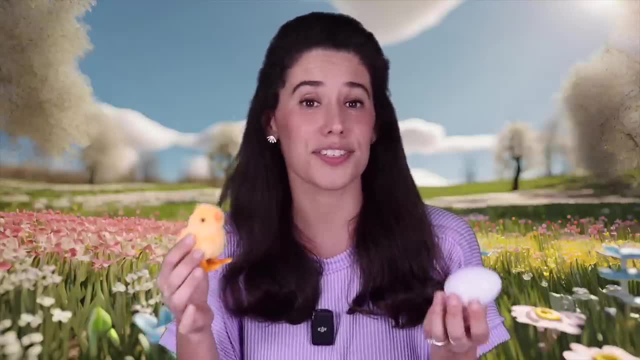 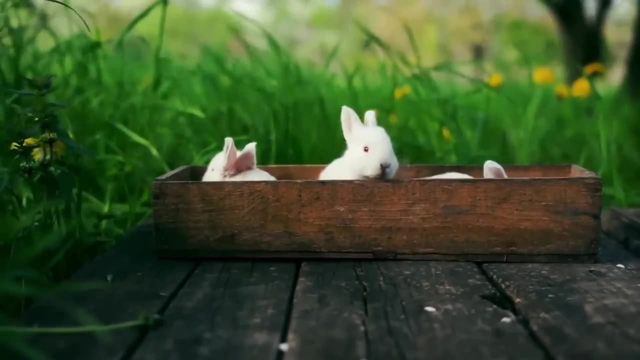 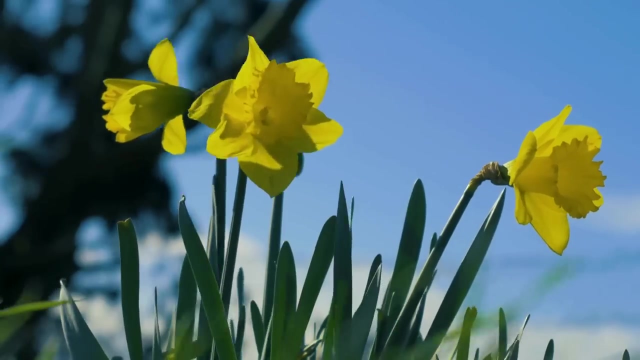 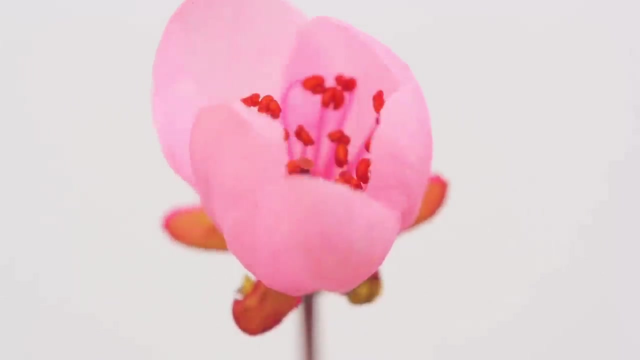 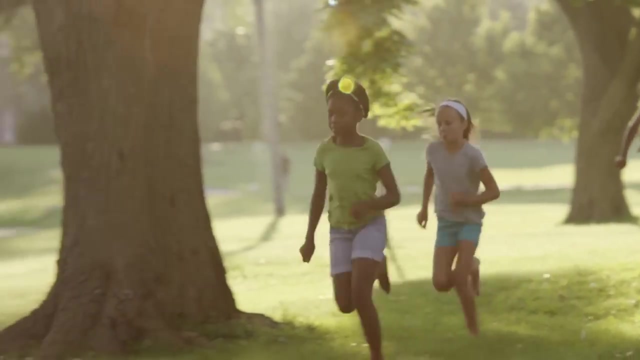 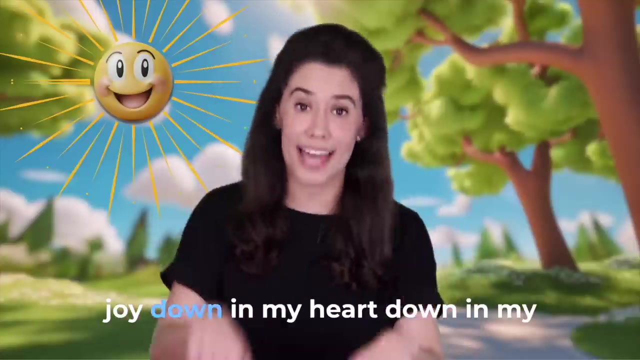 all about the different things about celebrating Easter and the different things that come to life, and about Jesus being alive. Let's watch next. I got the joy, joy, joy, joy down in my heart, down in my heart, down in in my heart. 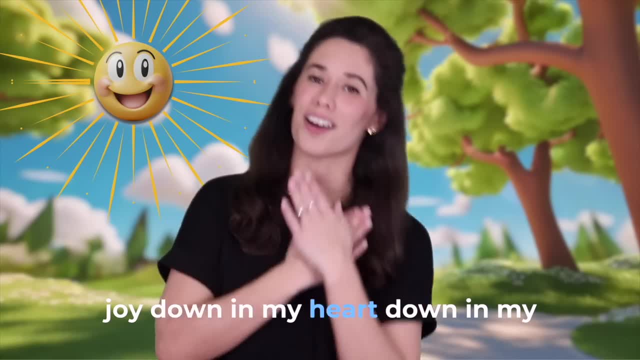 I got the joy, joy, joy, joy, the joy, joy, joy down in my heart. Down in my heart to stay, and I'm so happy that you came out here to play. Stay esteemed, so blessed, come every man that is held high and Ginsburg. 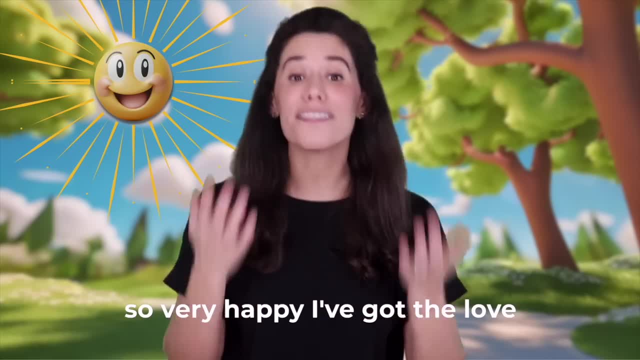 I will welcome you with grace. Start what you say by saying: oh praise God. Look, that's what God was going to say. so very happy. I've got the love of Jesus in my heart And I'm so happy, so very happy. 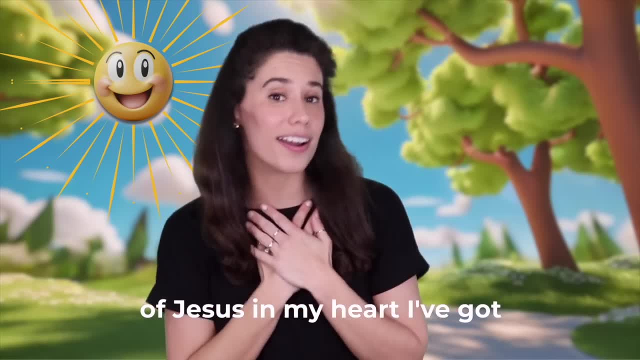 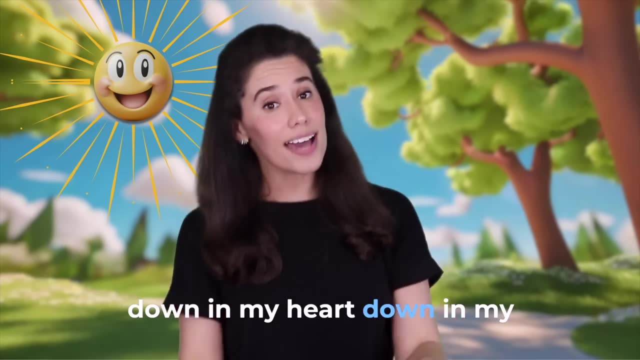 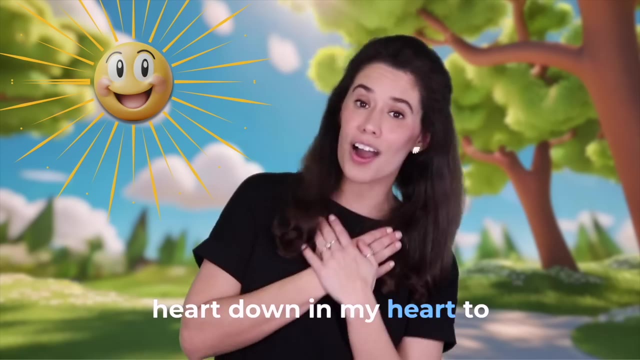 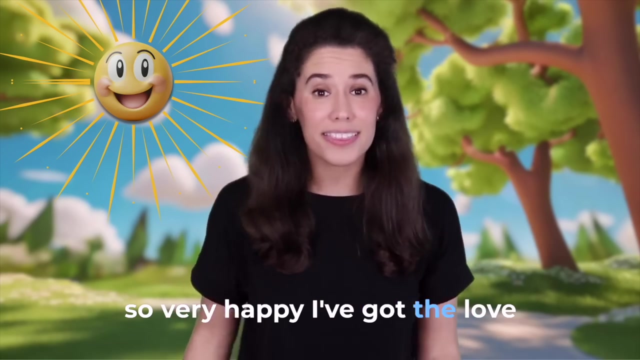 I've got the love of Jesus in my heart. I've got the peace that passes understanding down in my heart, down in my heart, down in my heart. I've got the peace that passes understanding down in my heart, down in my heart to stay, And I'm so happy, so very happy. I've got the love of Jesus. 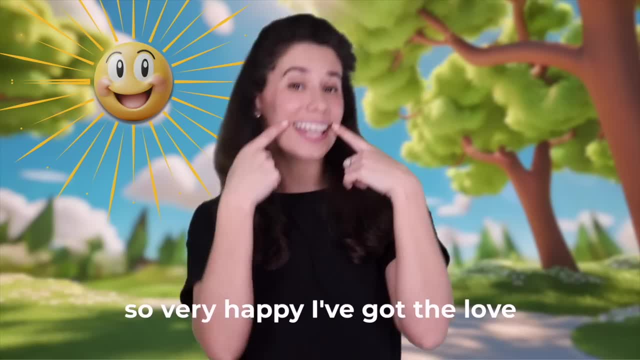 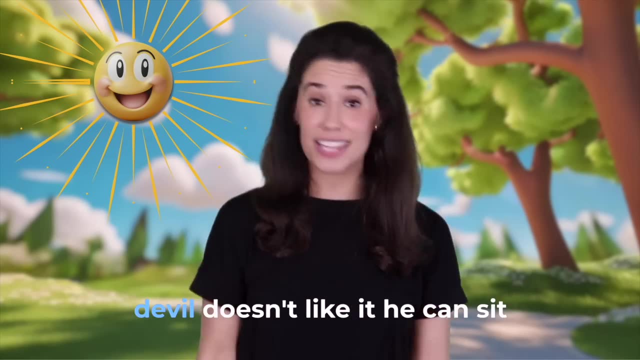 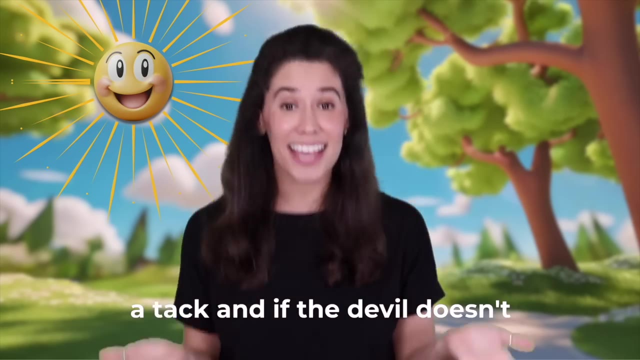 in my heart And I'm so happy, so very happy. I've got the love of Jesus in my heart And if the devil doesn't like it, he can sit on a tack. Ouch, Sit on a tack, Ouch, Sit on a tack. And if 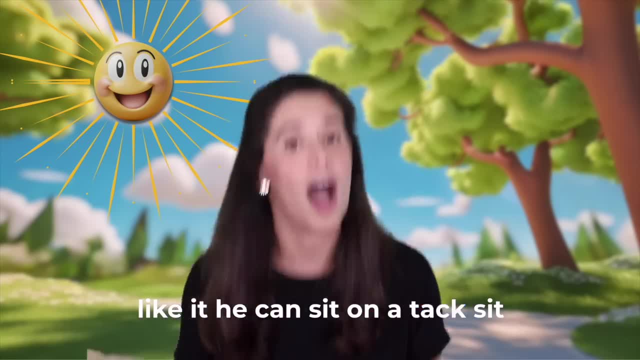 the devil doesn't like it, he can sit on a tack. Ouch, Sit on a tack, Ouch, Sit on a tack. And if the devil doesn't like it, he can sit on a tack, Sit on a tack to stay, And I'm so happy, so very. 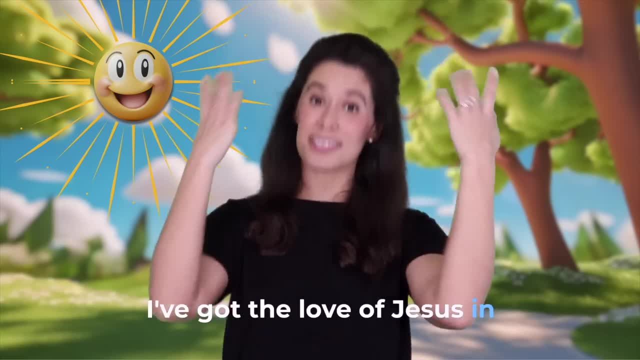 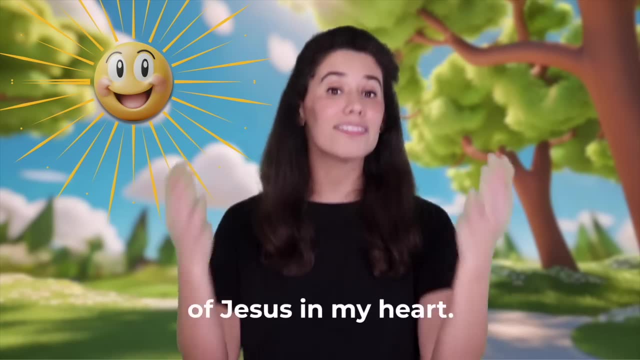 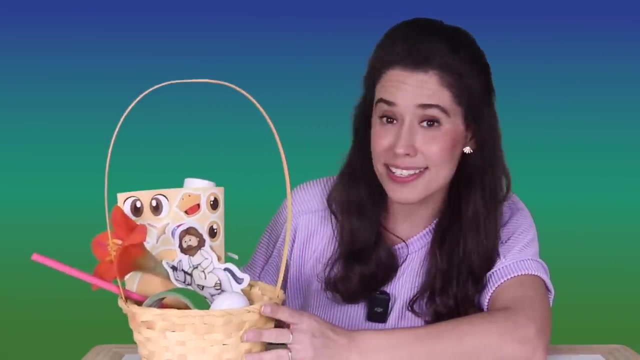 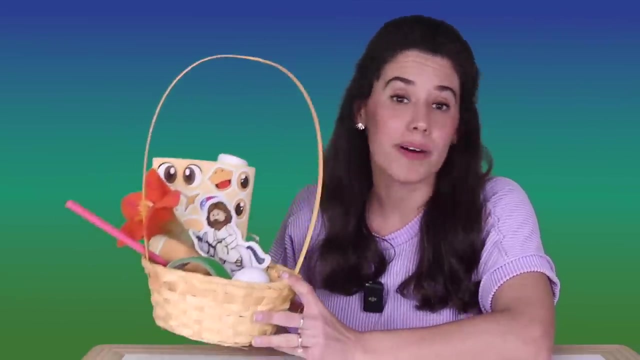 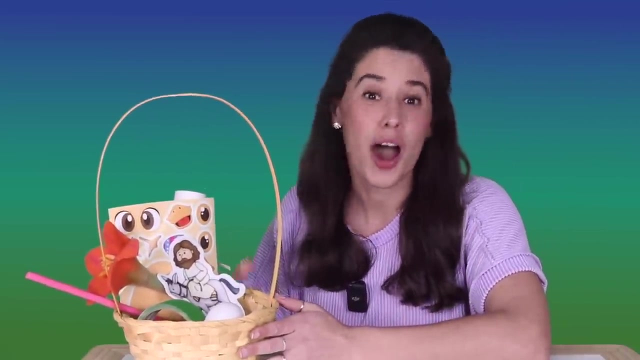 happy. I've got the love of Jesus in my heart And I'm so happy, so very happy. I've got the love of Jesus in my heart. Do you know what this is? This is my activity basket. Yes, it's going to help us know what activities we need to do today. Yes, it is What's in the basket. 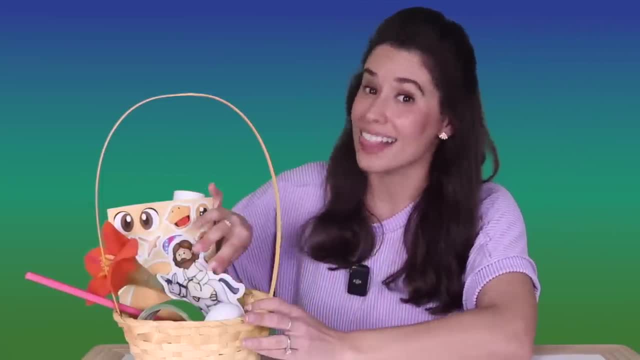 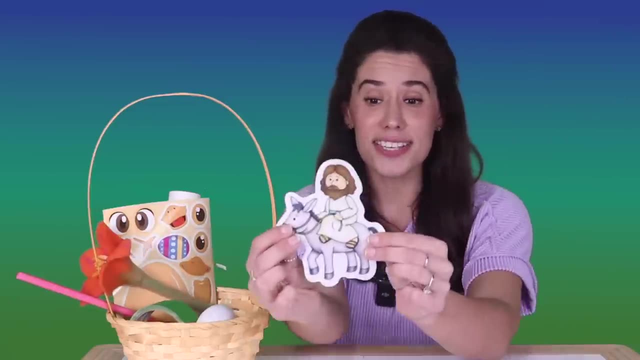 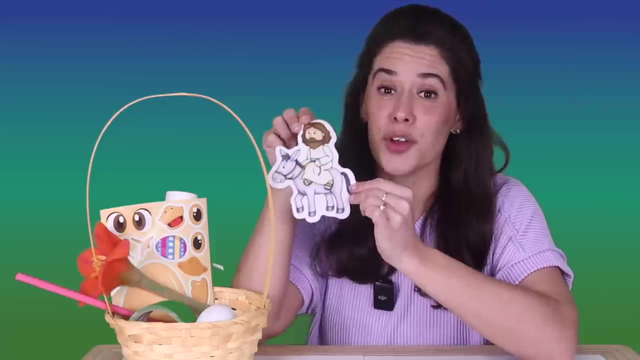 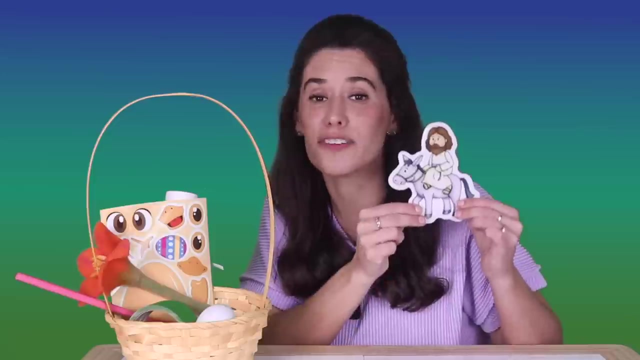 What could it be? What's in the basket? Let's look and see. Let's see what's in our basket. I see Jesus riding on a donkey. Yes, Jesus riding on a donkey. And you know what? That is part of the Easter story, Yes, And so I think our first activity is to go and learn about. 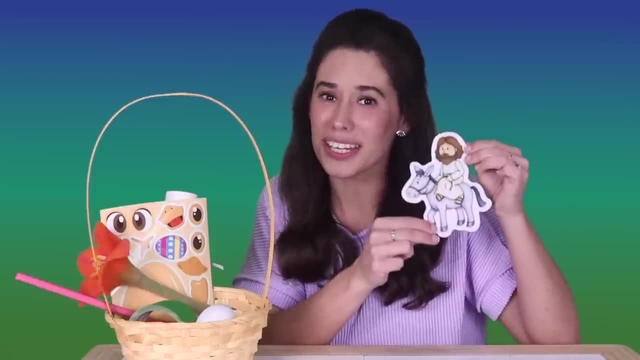 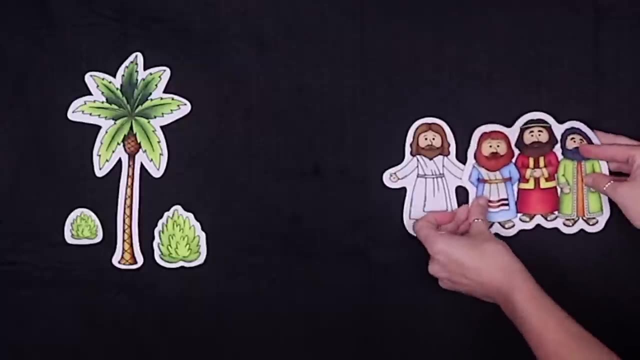 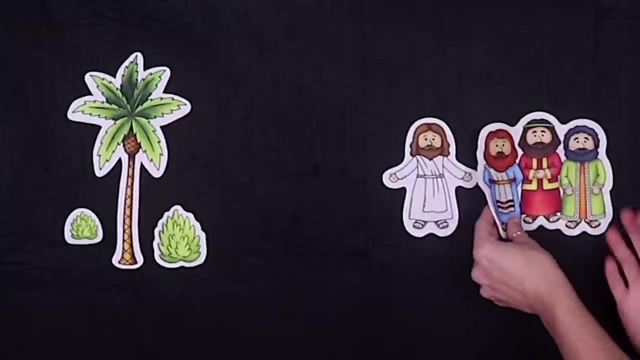 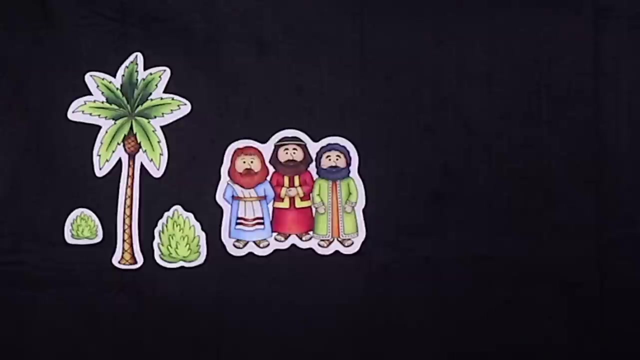 the Easter story. All right, let's go hear the Easter story. Jesus was traveling to Jerusalem with some of his disciples who were like his friends, And he asked them to go ahead and find him a donkey. And so his disciples went ahead of him and they brought him back. 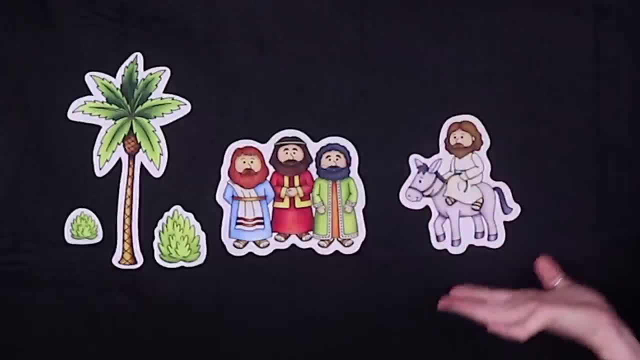 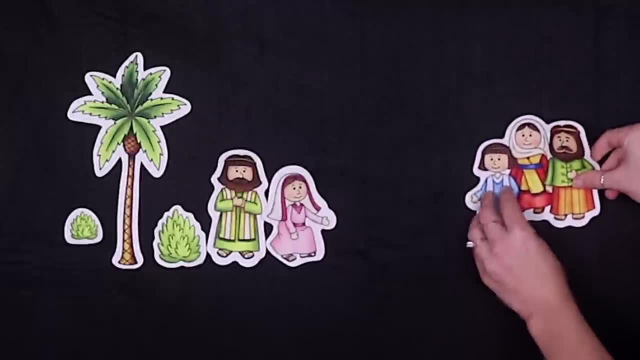 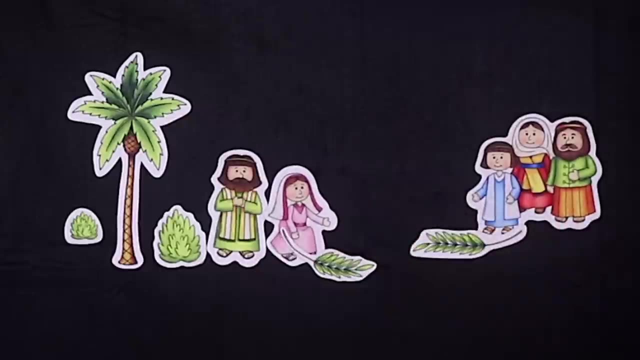 a donkey to ride on. Then Jesus rode into the city of Jerusalem on a donkey. Many people were excited to see Jesus and they laid down palm branches and cloaks to celebrate his arrival. They were so excited to see him and they shouted. 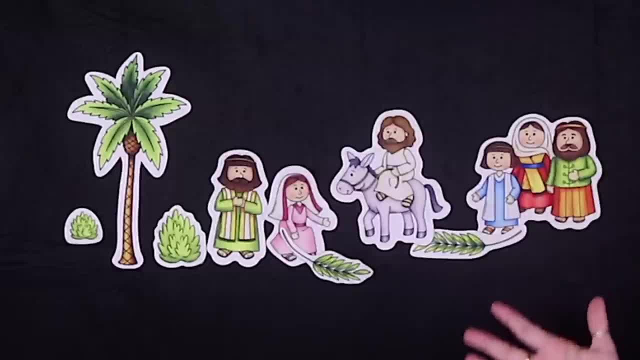 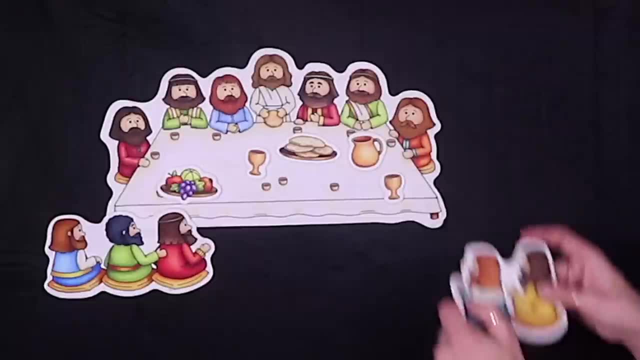 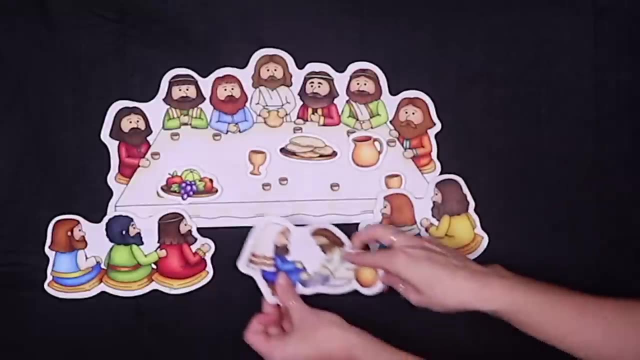 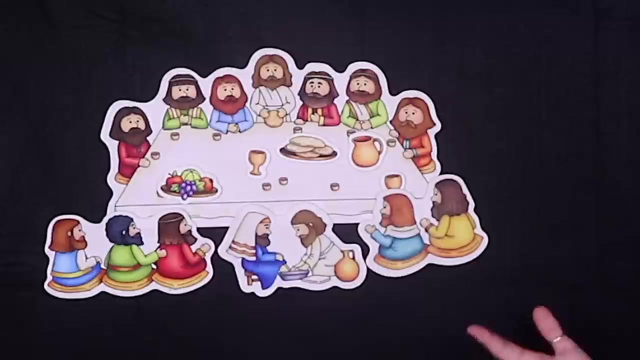 Hosanna to the Son of David. Blessed is he who comes in the name of the Lord. One night, Jesus was having dinner with his disciples. They were talking and eating And while they were there, Jesus even washed their feet. But he told them that one of them Named Judas. 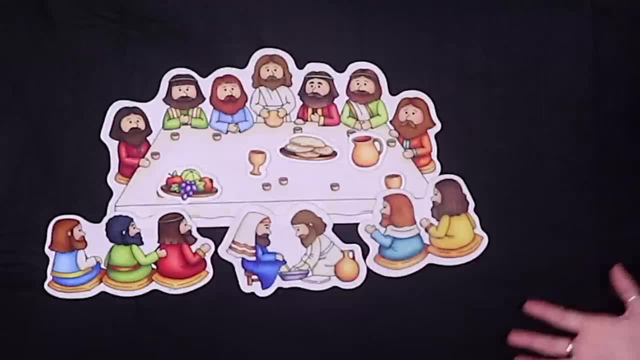 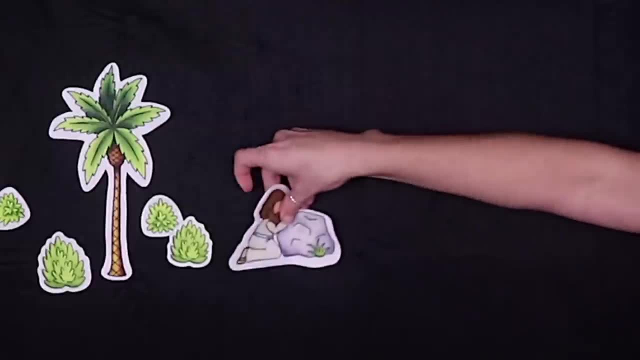 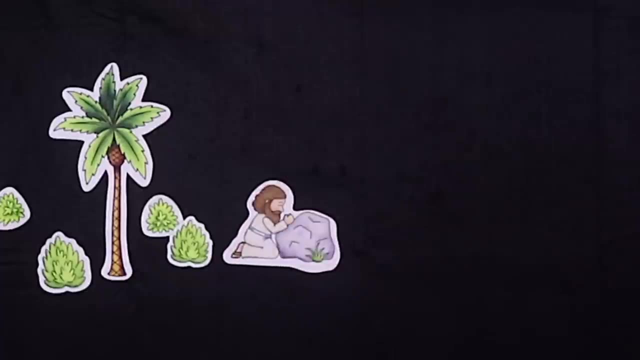 Was going to betray him, And that means that he was going to give Jesus to the people Who didn't like him. After dinner, Jesus went to a garden to pray to God, And while he was praying, The people who didn't like him Sent soldiers to come and take him away. 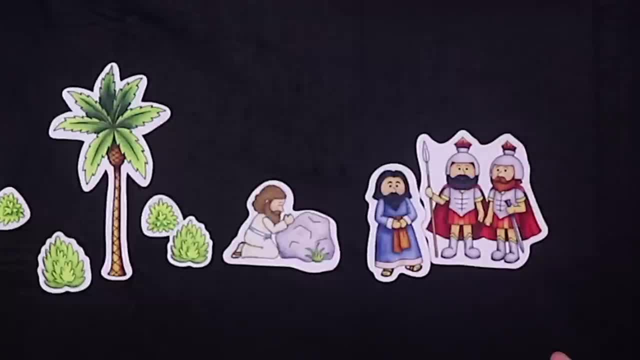 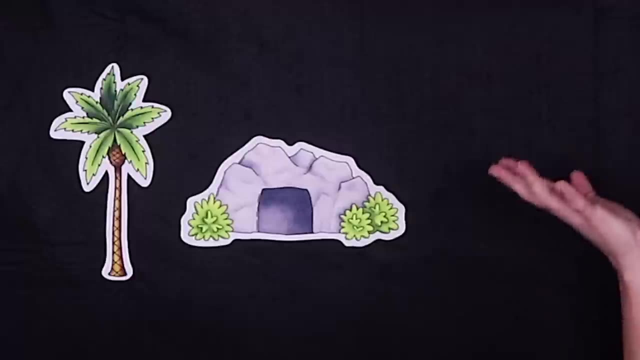 Judas was the one who told them where Jesus was, And they were not nice to Jesus. They sent Jesus to die on a cross, And they were not nice to Jesus. And they were not nice to Jesus. After Jesus died, they placed him in a dark cave called a tomb and they put a large, heavy 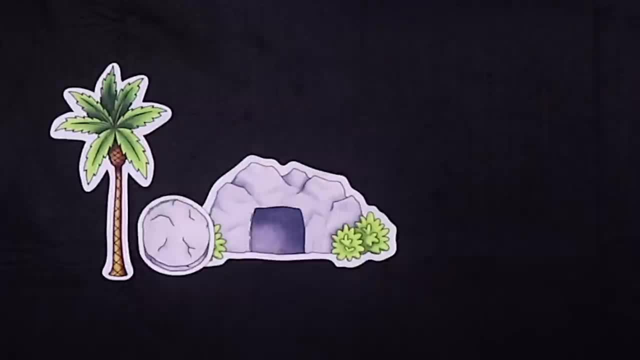 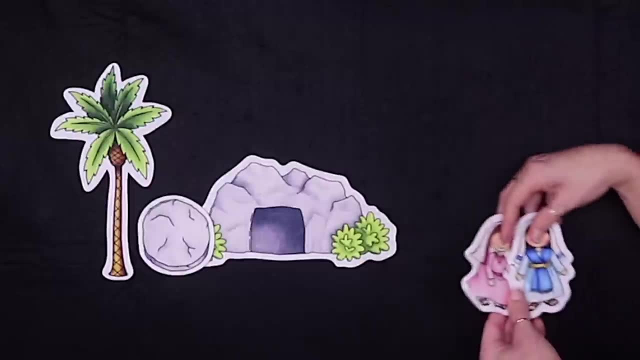 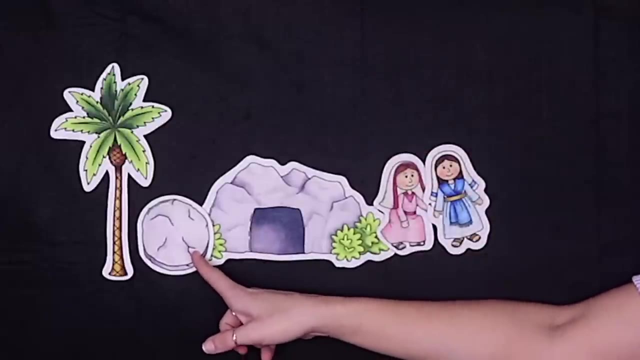 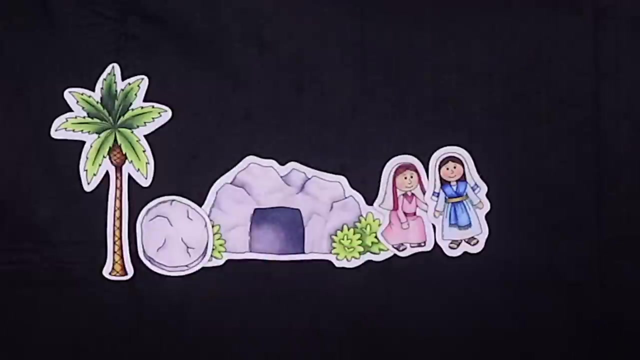 stone over the entrance. After Jesus had been dead for three days, some of his friends went to the tomb, but they were shocked to find that the stone was not there anymore. It had been rolled away and the dark cave was empty. But then an angel appeared to them, and the angel told them that Jesus had risen and that 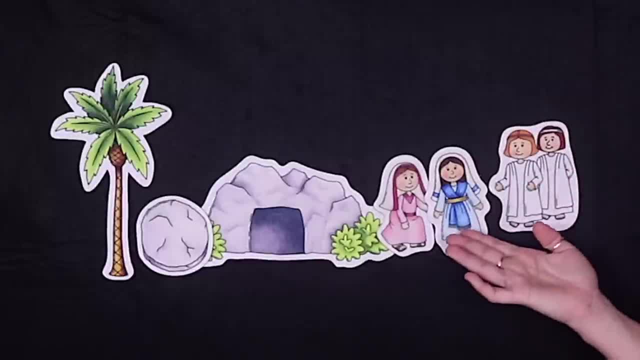 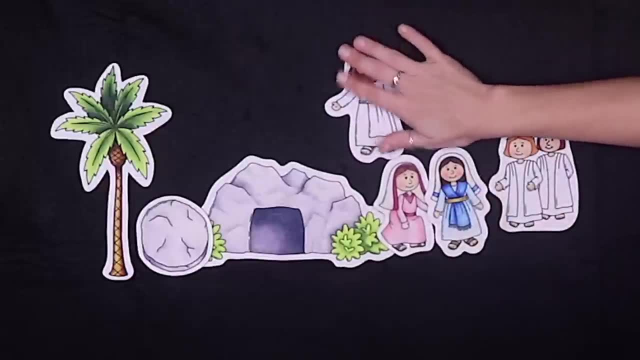 he was not dead anymore. Jesus' friends were so happy and excited because Jesus was alive. Jesus was alive and he never died again. He went back up to heaven. Jesus was alive and he never died again. He went back up to heaven. 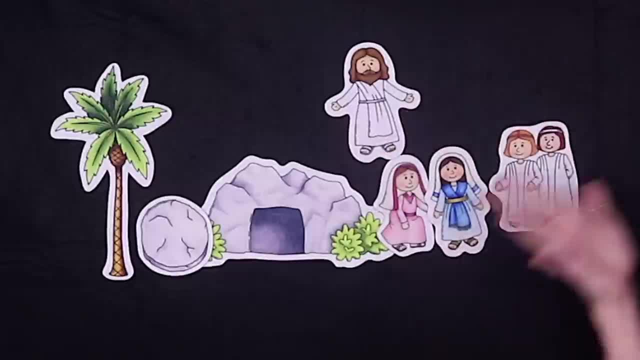 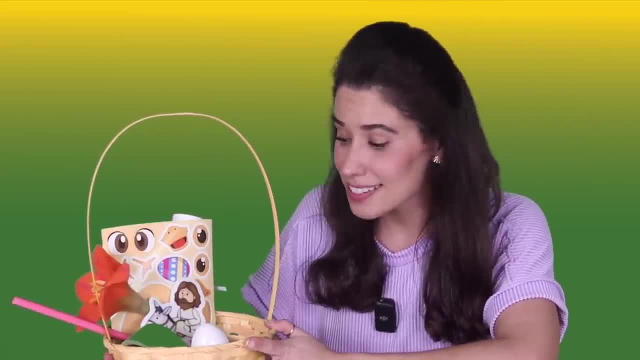 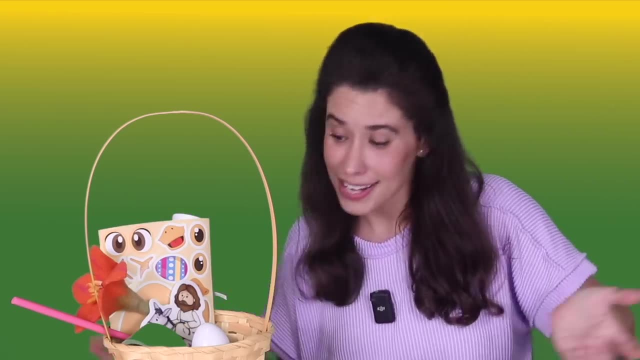 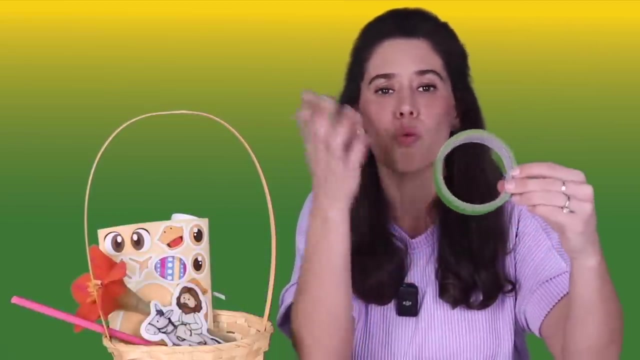 Which means that we get to be friends with Jesus. What else is in our activity basket? What's in the basket? What could it be? What's in the basket? Let's look and see. I see some green tape. I wonder what we could be doing with this green tape. 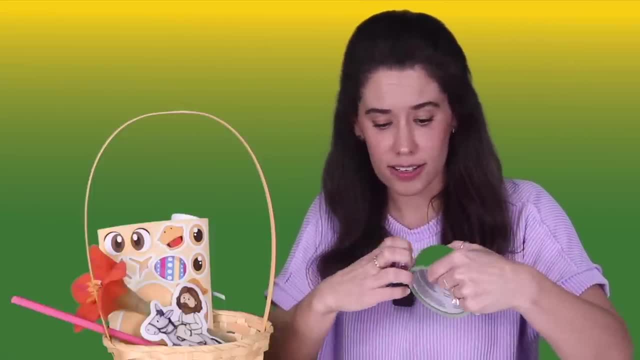 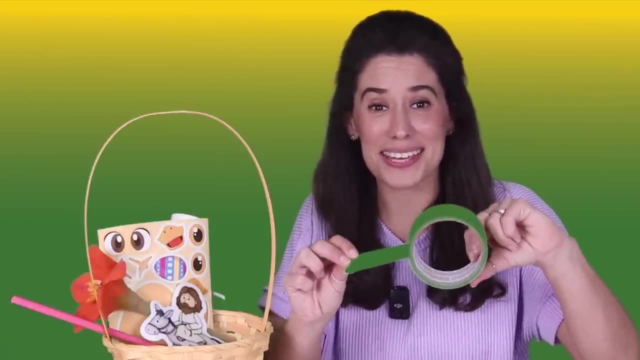 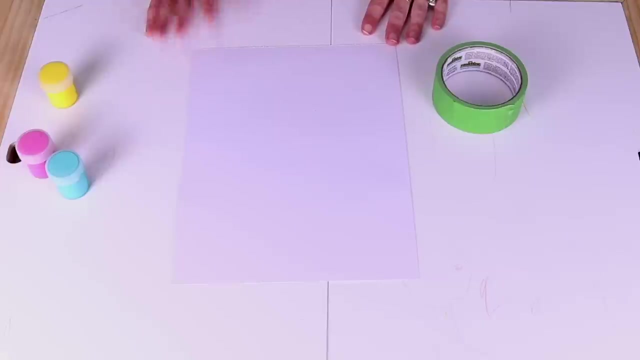 Hmm, I'm sure it's a green tape, something fun, Let's see. All right, let's go and do our next activity with some green tape. All right, this activity is a little bit messy, So you might want to put on an apron, All. 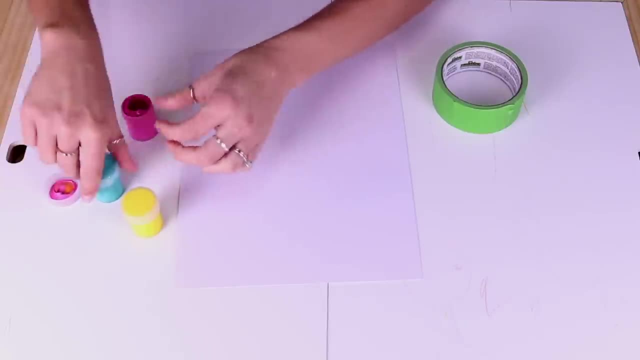 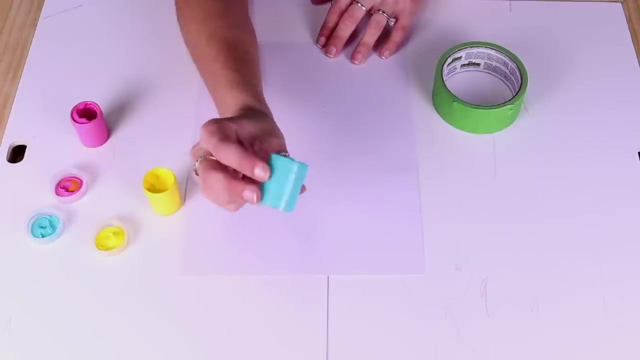 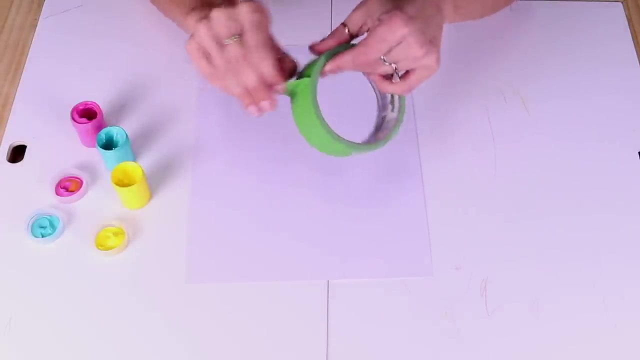 right, here are my paints. Gonna open them, open them and open this one. All right, there are my paints. I have pink, right here, pink, And I have teal or mint, And I have yellow. All right, and I've got my tape. So what we're gonna do is we're. 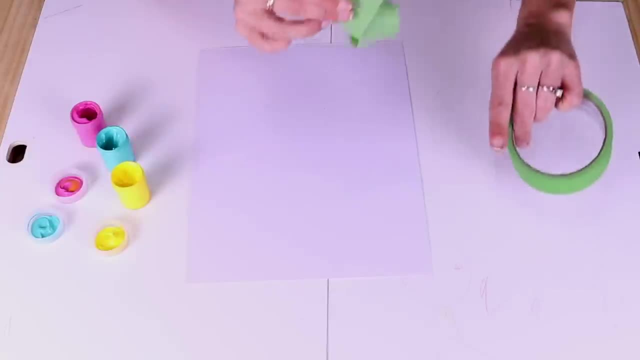 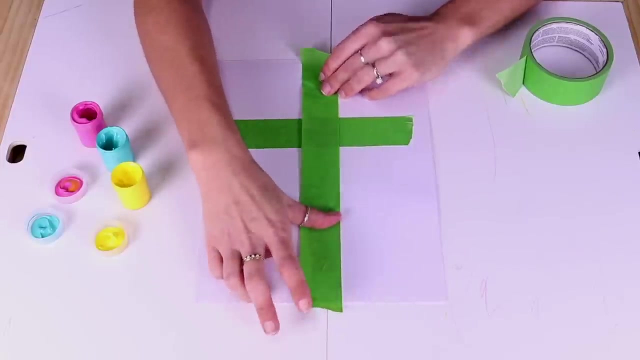 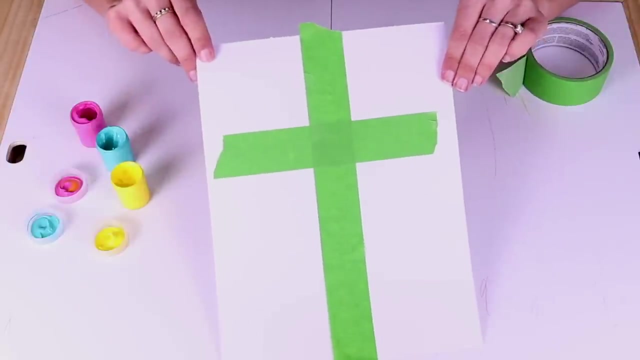 gonna take a piece of tape and we are gonna put it across our page, just like this: We go And then we're gonna take a longer piece- What? And we are gonna tape that piece this way. All right, and you know what we've made? A cross, Just like Jesus died on. 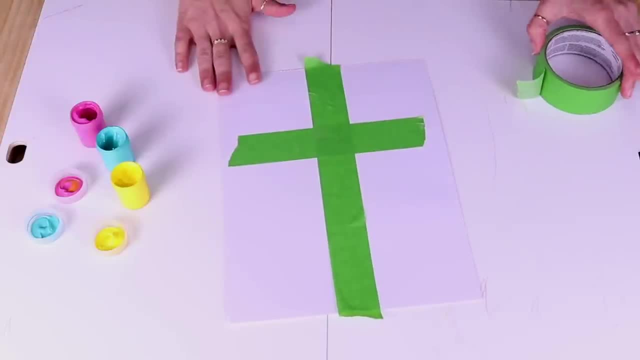 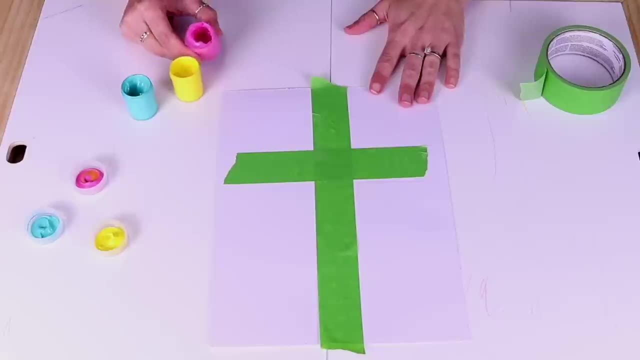 the cross. We're gonna make a cross, Okay. so now we've got our paints And we're going to use our fingers to paint All around the cross. Okay, we can paint over it a little bit and all around it in the different colors. So first I'm 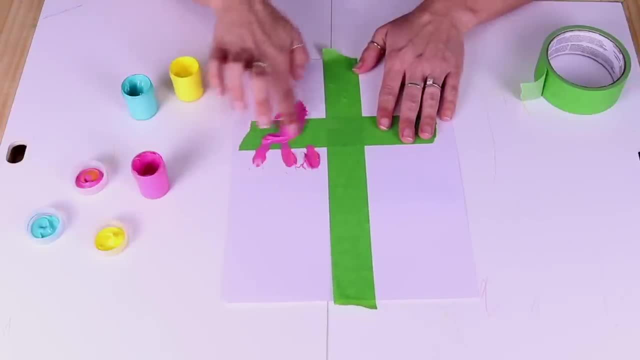 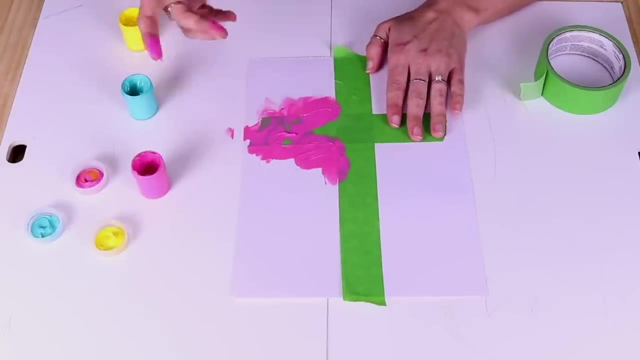 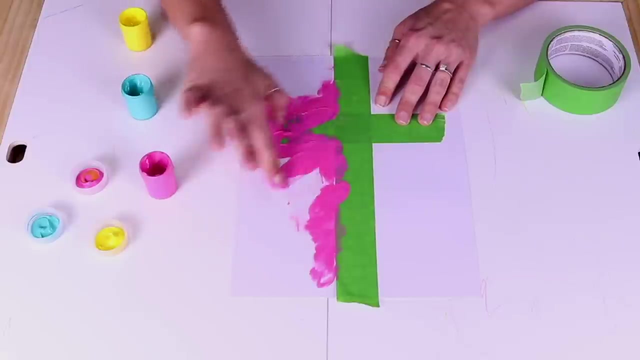 gonna start with pink And do some pink paint Right around the edges. You can try to keep it on the page, but sometimes it might come off. All right, let's do some pink. It's looking pretty. Got some pink. 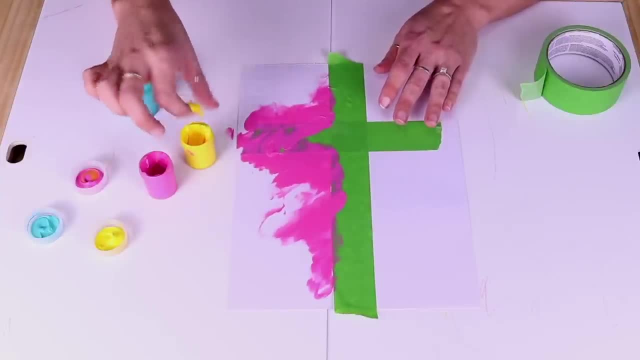 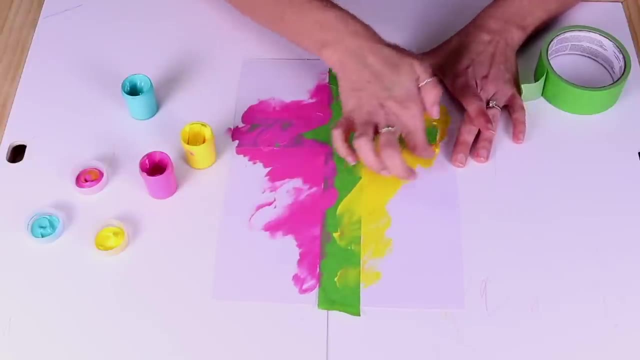 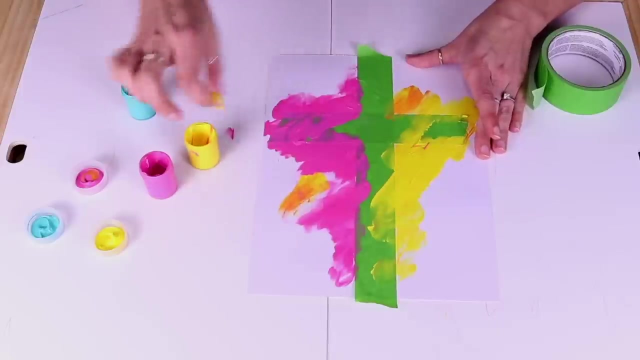 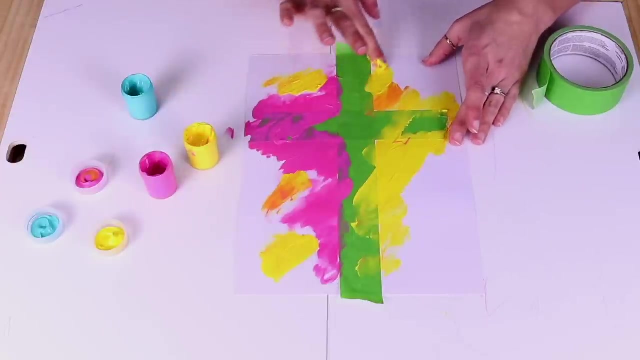 There we go. All right, now I'm gonna use some yellow Yellow over here. Some pretty yellow on my picture. Yellow is such a bright and pretty color. Let's put some yellow down here. There we go. That's looking beautiful, I like yellow. Okay, now let's. 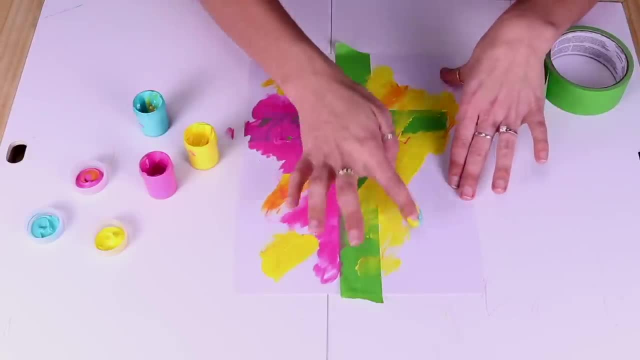 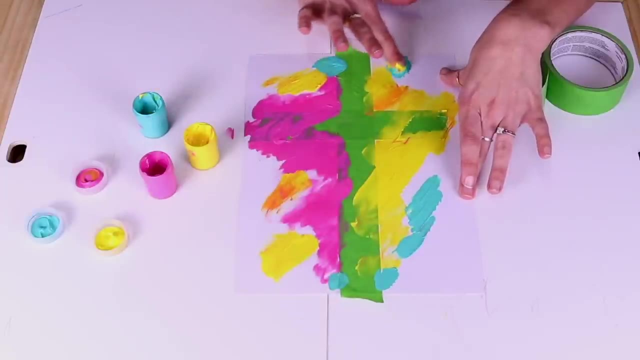 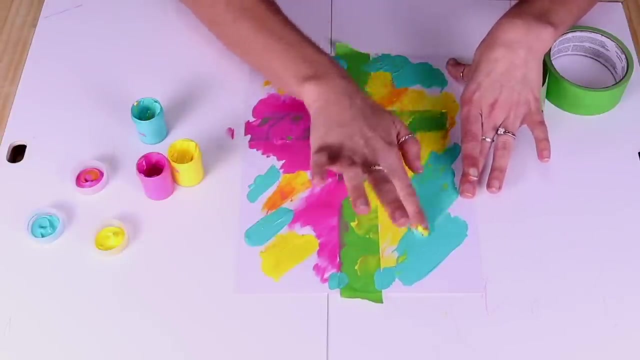 take this color, The turquoise color, Add some of that Right. Here we go. This is also a pretty color. Love this one. Some right there, Some right here. Oh, that's looking so pretty. Okay, Now, now that. 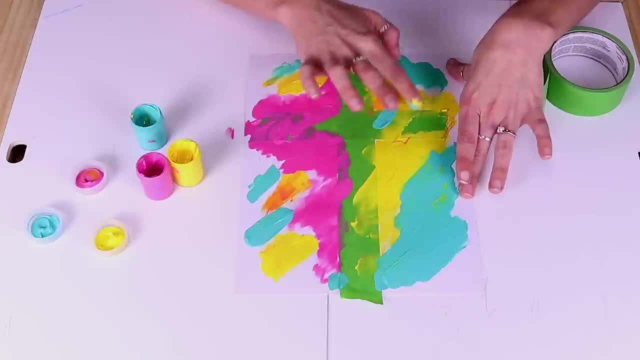 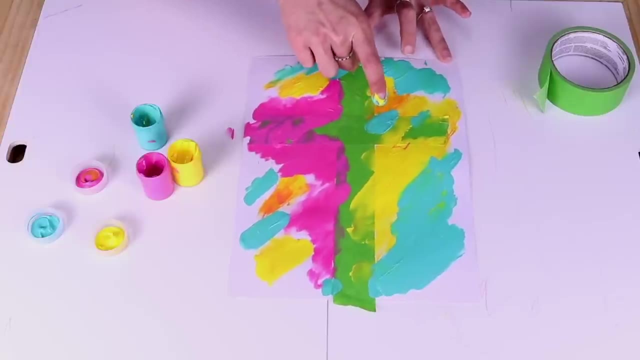 we're all done Adding on our colors. What we're going to do is take off our tape. All right, we're gonna pull it from one side and just take it off. There we go. There's one piece, And now let's take off our other piece. 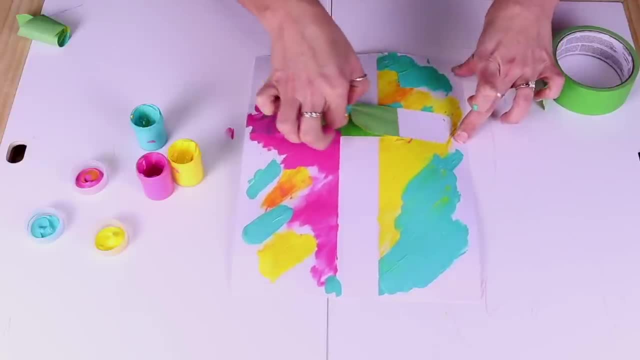 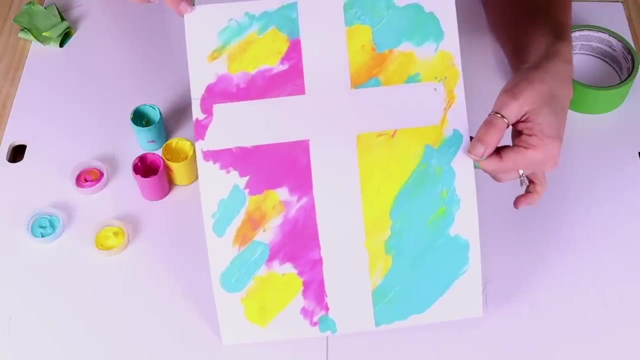 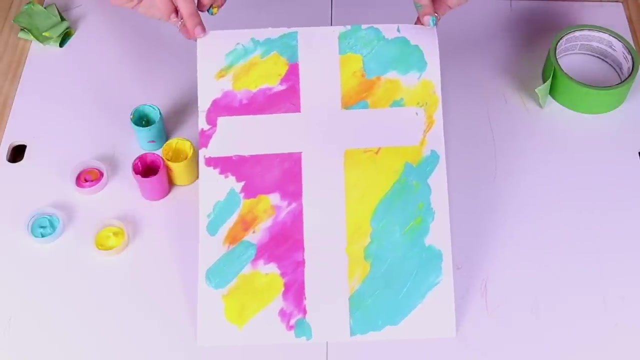 Try and grab the corner and pull it off. Wow, look at that, We have a beautiful cross left. We made a beautiful cross, We painted around it and we took off the tape and we're left with a beautiful cross. And if you make 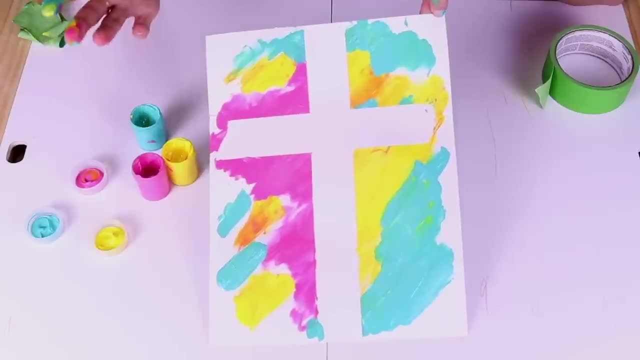 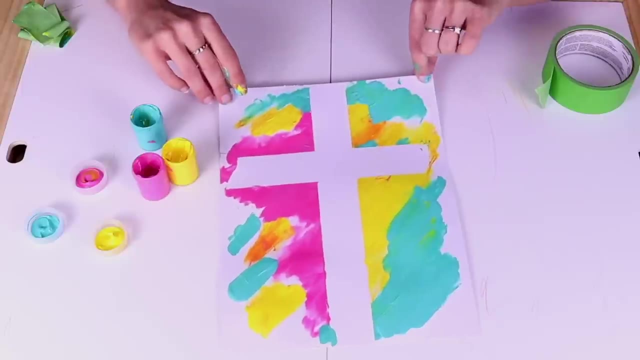 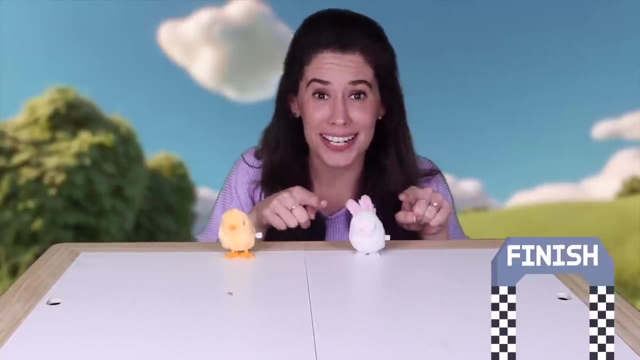 one too. you can hang this in your room to remind you that Jesus died on the cross for us because he loved us. Thank you for doing this fun activity with me. Look what I have here. I have a little bunny that hops around and I have a little chick. 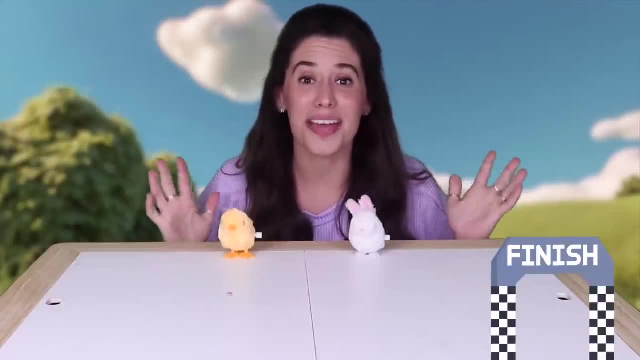 that says peep, peep, peep, peep, peep. And you know what? They were just telling me? that they want to race each other. All right, so let's watch them race. We're going to count to three. 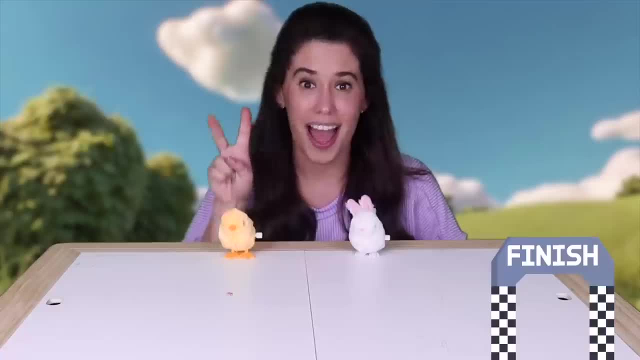 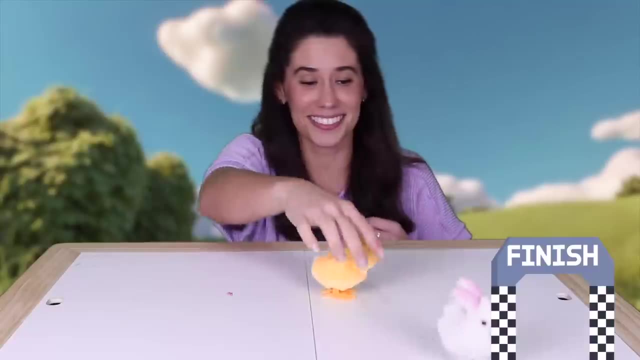 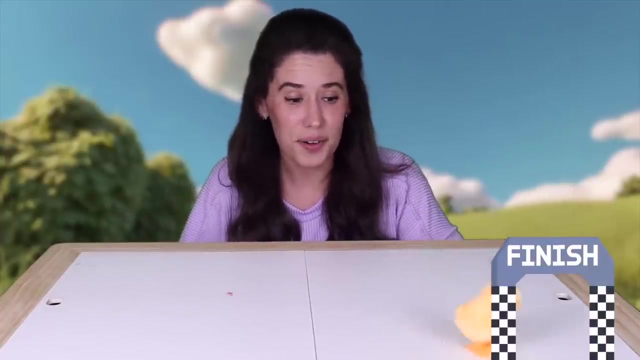 Okay, you can count with me One, two, three, Go, go, go go. What happened? Our little chick stopped running. Go, go, go. Good job, little chick. Our bunny won. Our little chick got a. 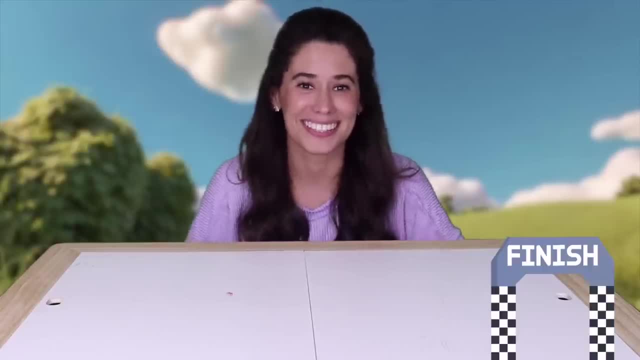 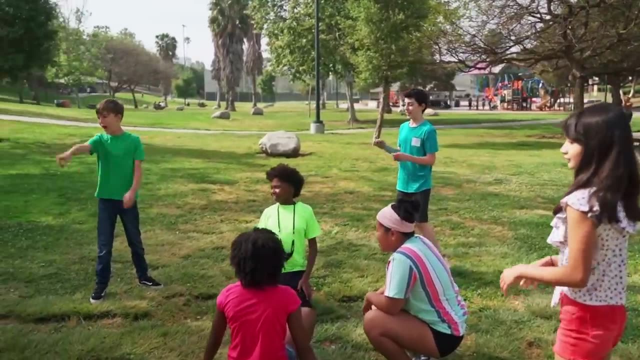 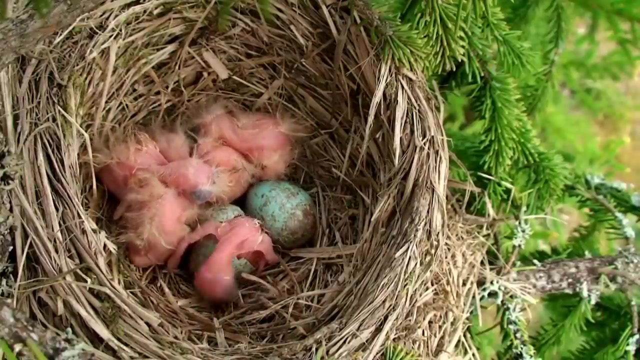 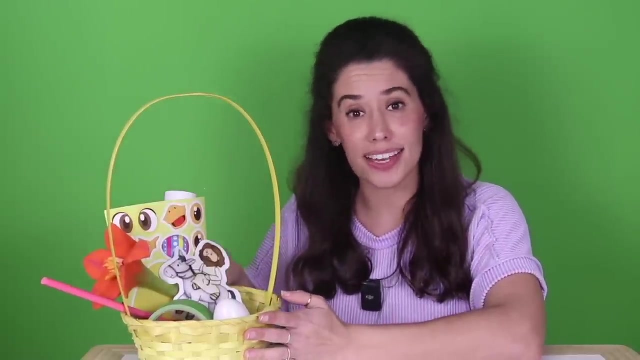 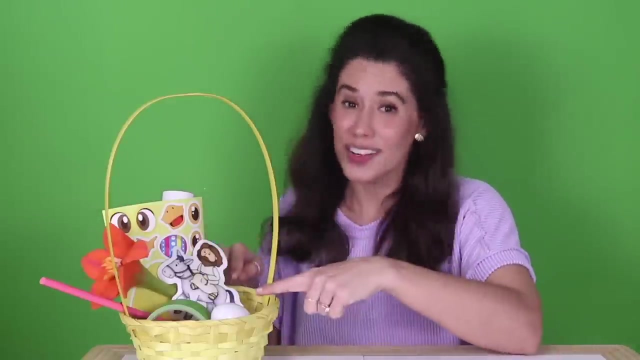 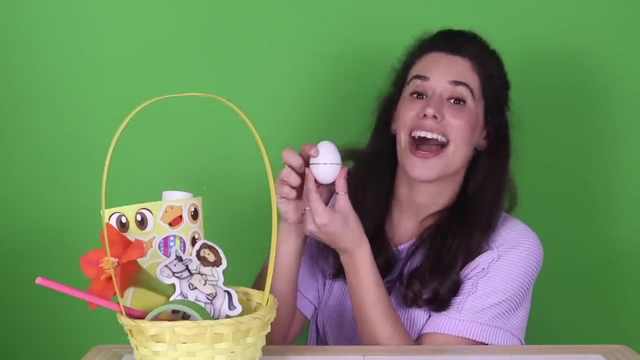 little bit stuck. Good job, bunny. All right, let's see what else is in our activity basket. What's in the basket? What could it be? What's in the basket? Let's look and see. I see an egg. Yes, an egg. I think our. 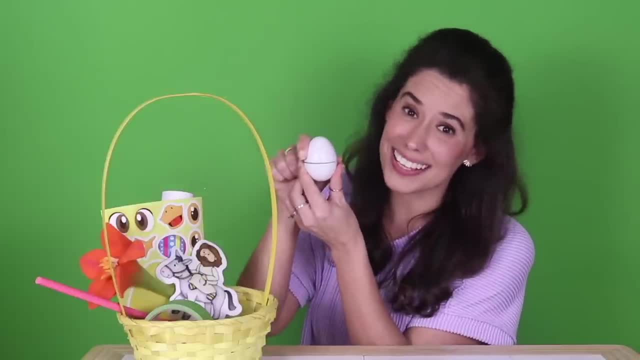 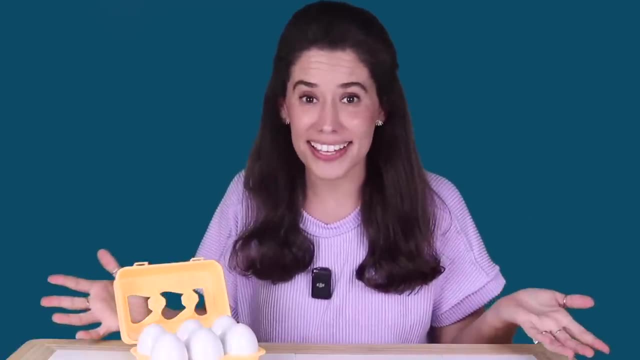 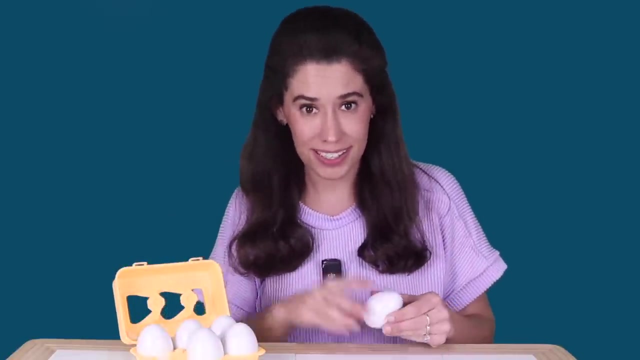 next activity is going to be something with eggs. Let's go and do our next activity. have my carton of eggs. Why don't we see what's inside these eggs? Do you want to open them with me? Yes, Alright, let's say. 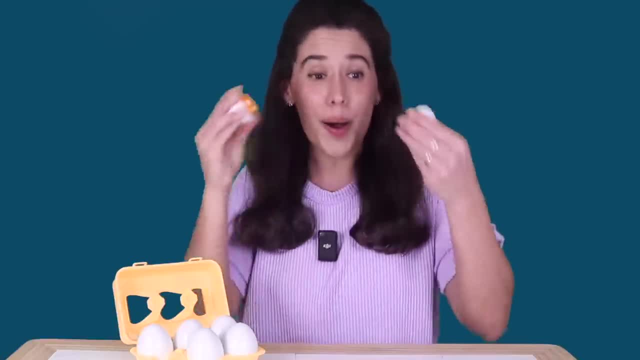 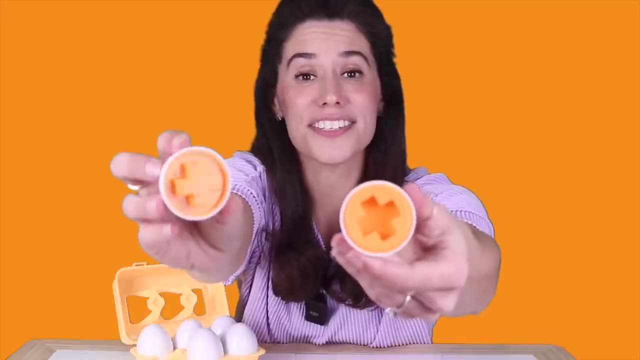 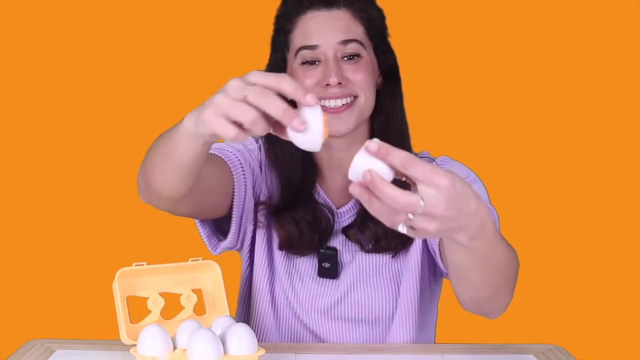 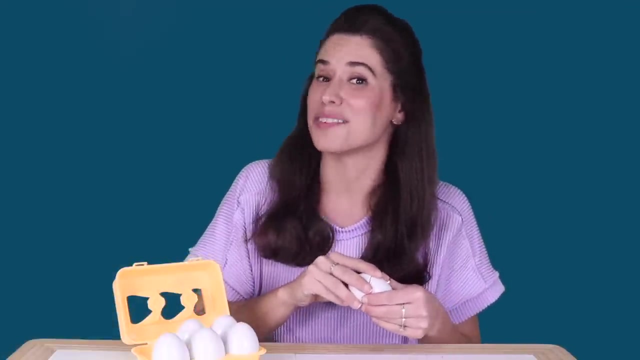 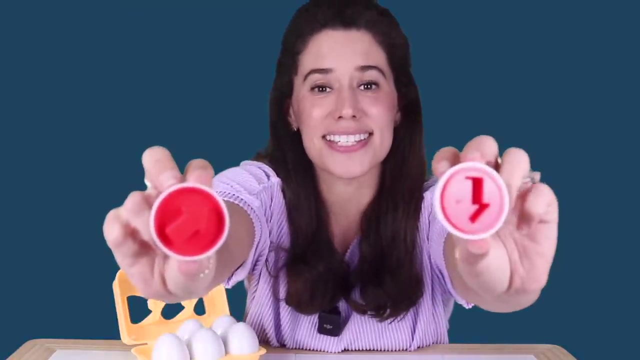 open together. Open, open, open, Wow. look, this egg is orange. The color inside this egg is orange, Orange, An orange egg. What do we have next? Say open and we'll open it together. Open, open, open, Wow. This is a red egg On the inside of this. 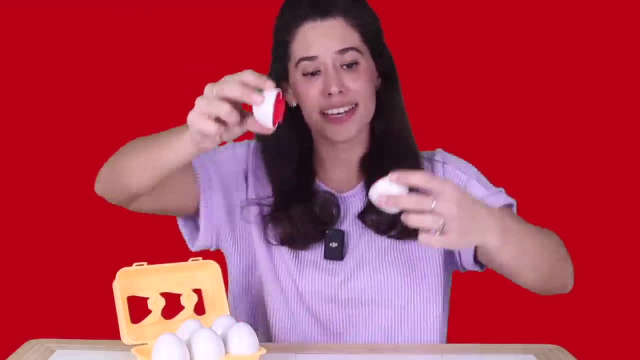 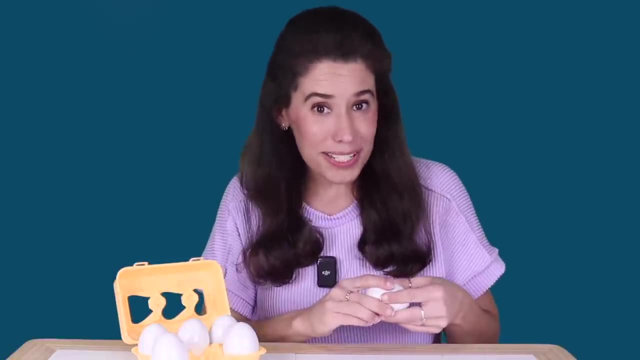 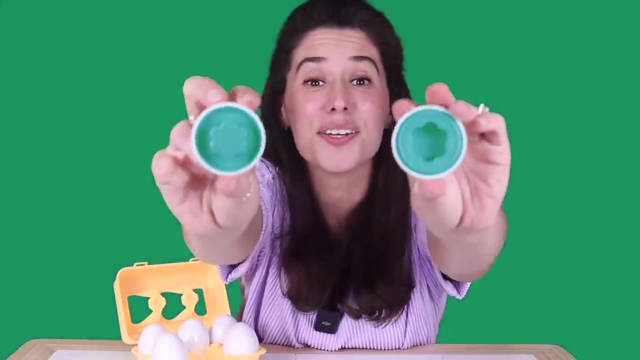 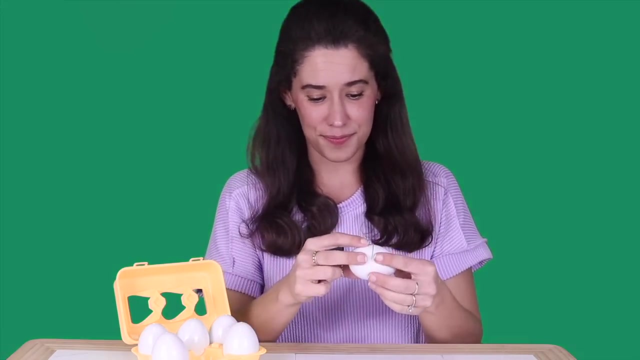 egg. it is red, Red, A red egg. Alright, what's next? Let's say: open together, Open, open, open. This egg is green. The inside of this egg is green Green. Alright, what else do we have? We have a few more eggs. Let's 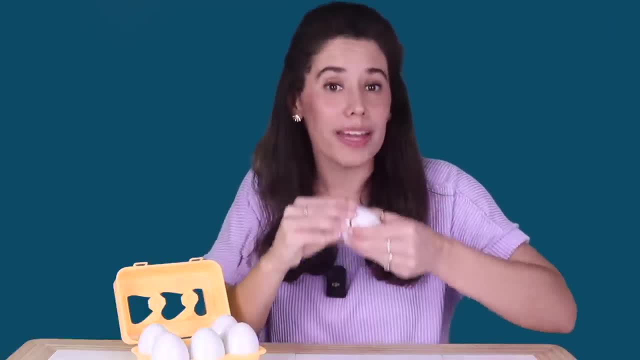 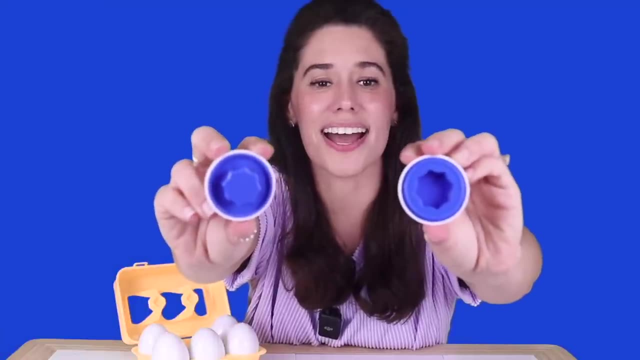 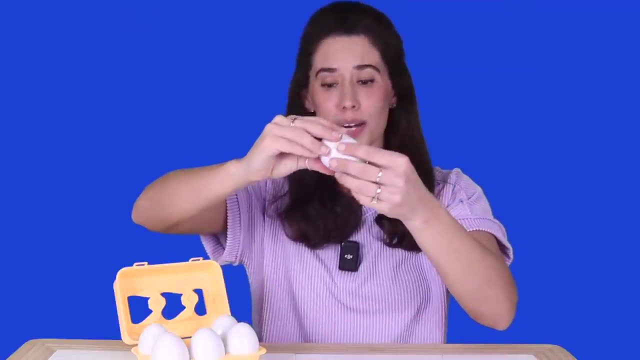 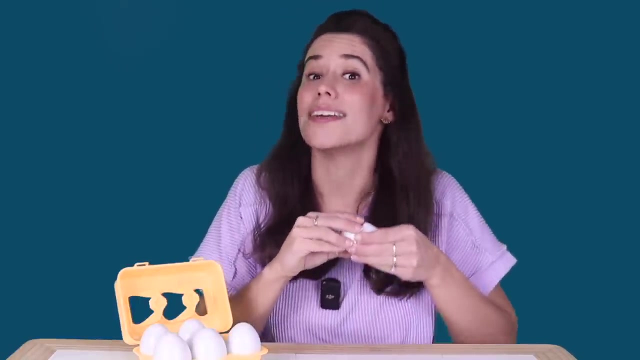 say: open together, Open, open, open, Open. This is a pretty egg. It's blue inside. Look at that beautiful blue. This egg is blue. What a pretty egg. OK, What's next Say: open with me, Open, open, open. This is a. 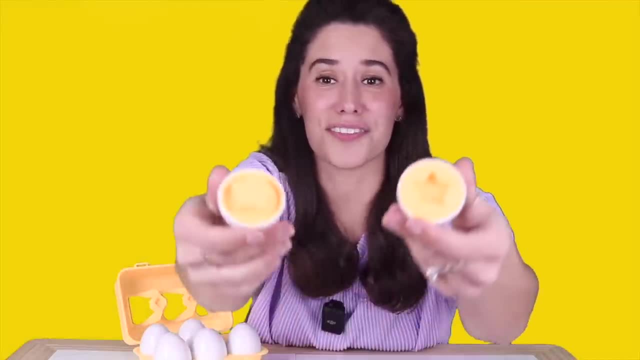 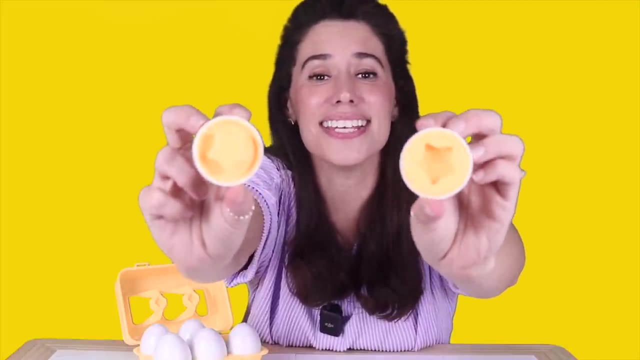 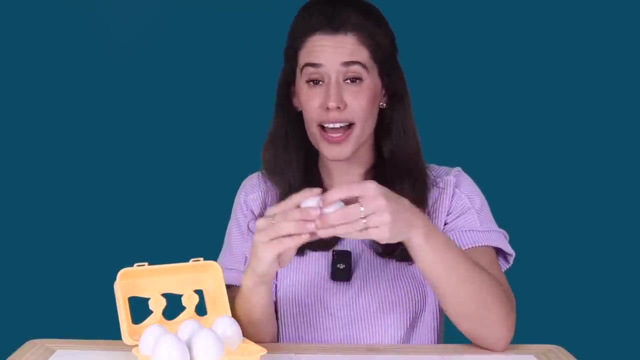 yellow egg. This is probably the color of the eggs that you see when you open an egg egg at home: Yellow. This egg is yellow. All right, we have one more. What color do you think could be in our last egg Say? 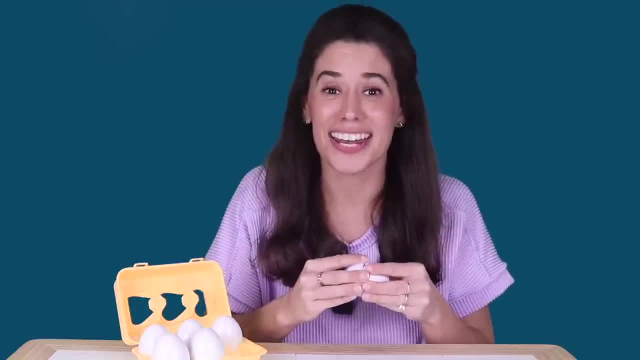 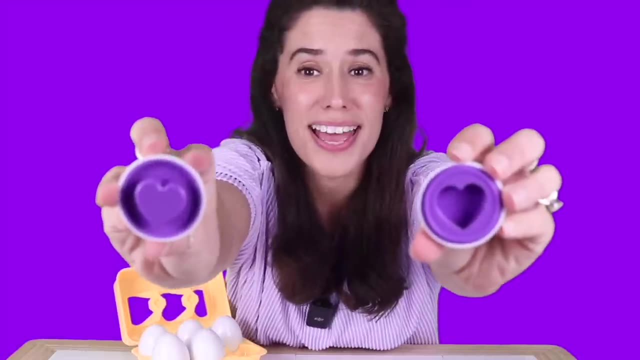 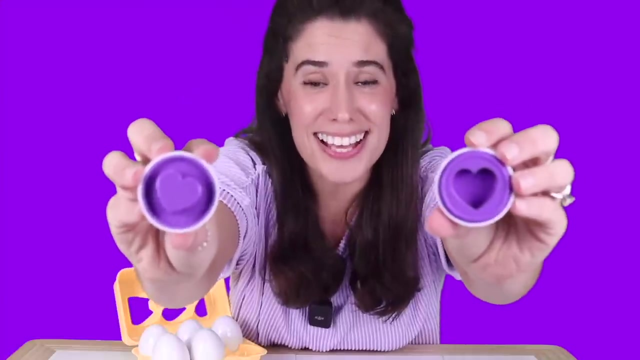 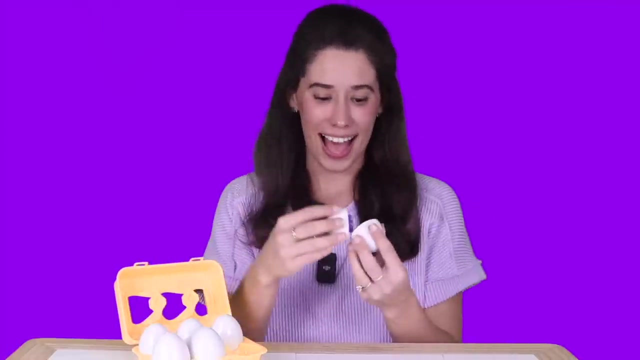 open with me and we'll open it together. All right, Open, open, open. Wow, it's purple And it's a purple heart, A heart that shows that Jesus loves us. Purple, A purple heart. I love purple. Thank you for opening these eggs with me. I had so. 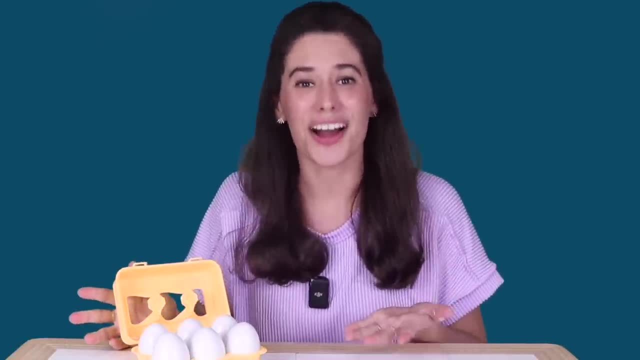 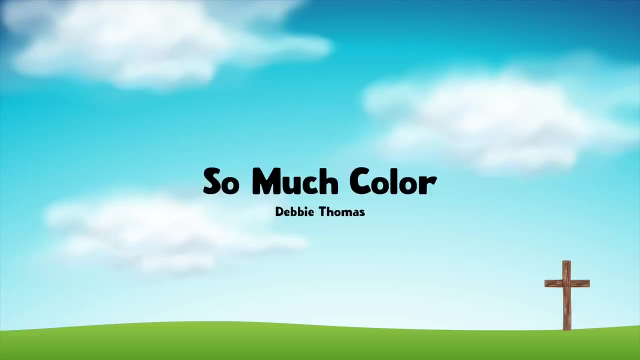 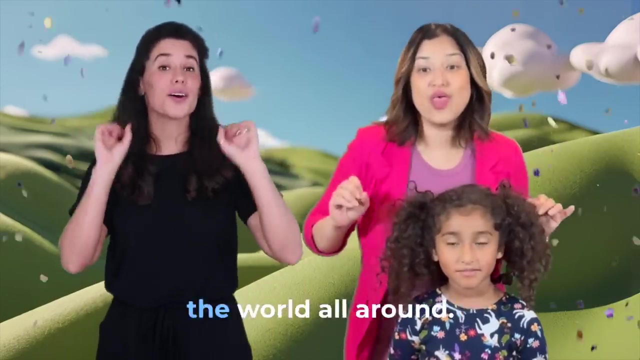 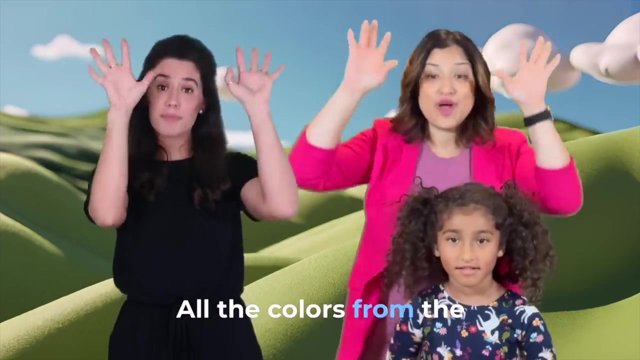 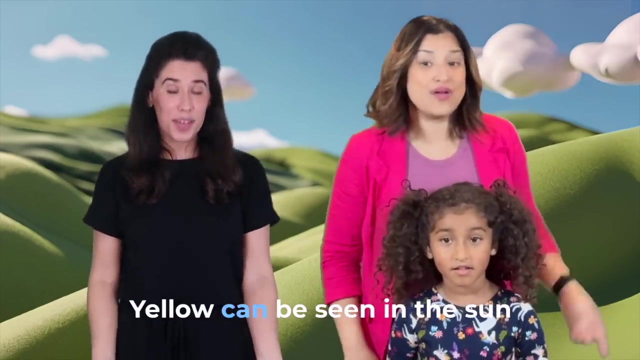 much fun learning all the colors that were inside our egg. There's so much color in the world all around And when you see it you've got to know it. All the colors from the sky to the ground. Blue is in the sky. Green is in the grass. Yellow- 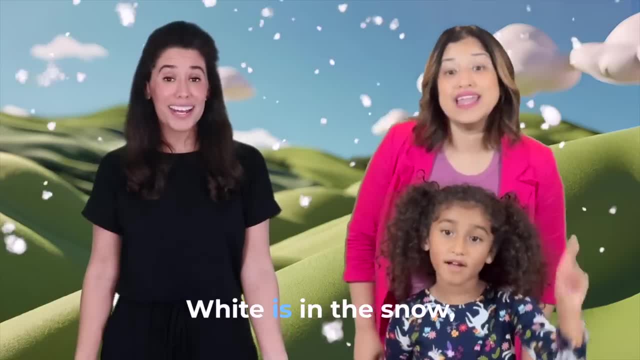 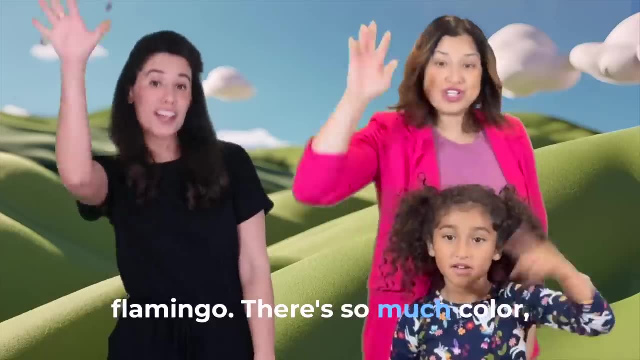 can be seen in the sun. White is in the snow, Red is in the rose, Pink in a tall flamingo. There's so much color What. There's so much color Where. There's so much color in the world, all around And when. 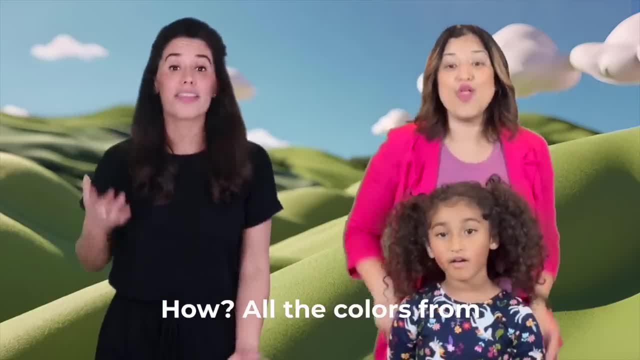 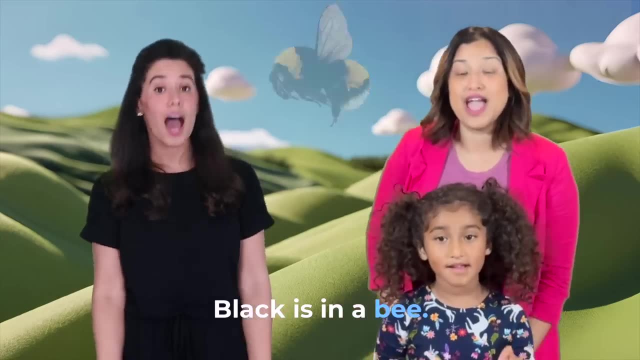 you see it? Yeah, You've got to know it How. All the colors from the sky to the ground. Brown is in a tree, Black is in a bee, Gray is in the color of Ross, Orange in a year, Blue is. 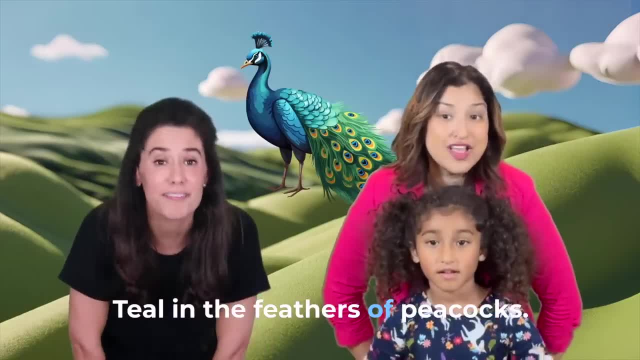 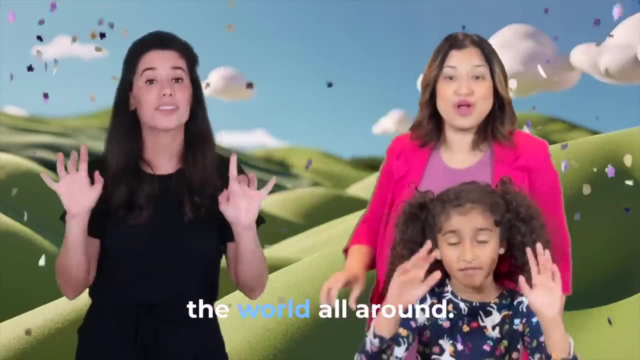 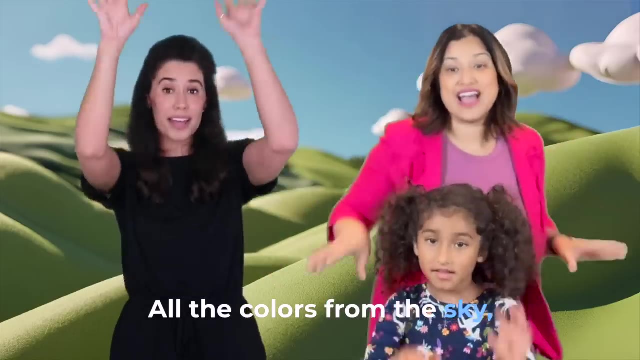 in a jam. Purple in a jam Dew, in the feathers of peacocks. There's so much color What? There's so much color Where. There's so much color in the world all around And when you see it. Yeah, You've got to know it. How All the colors from? 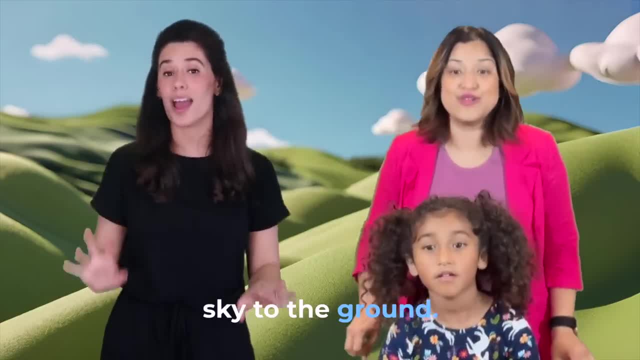 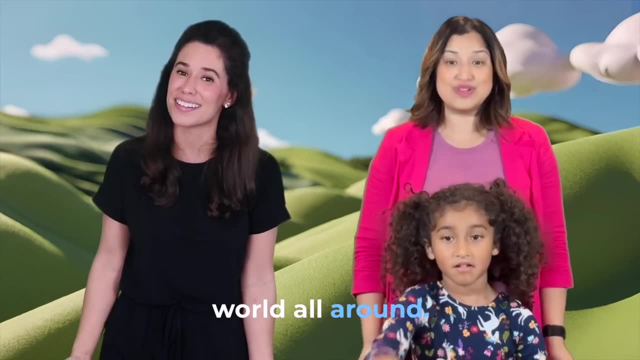 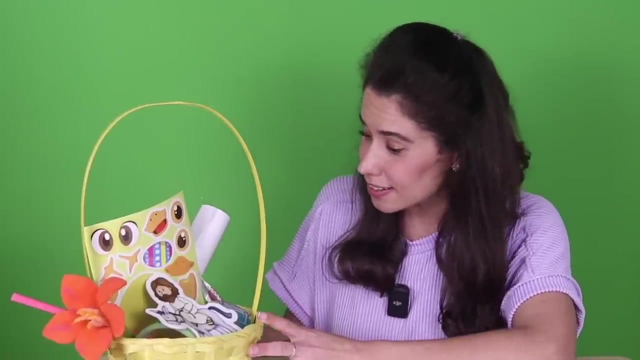 the sky to the ground. All the colors from the sky to the ground. So much color in the world all around. Yeah, Okay, let's take something else out of our basket. What's in the basket? What could it be? What's in the basket? 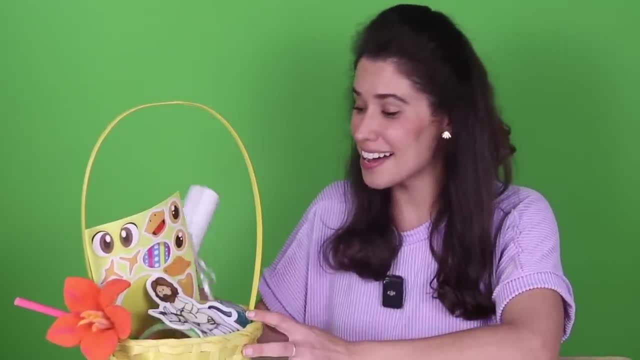 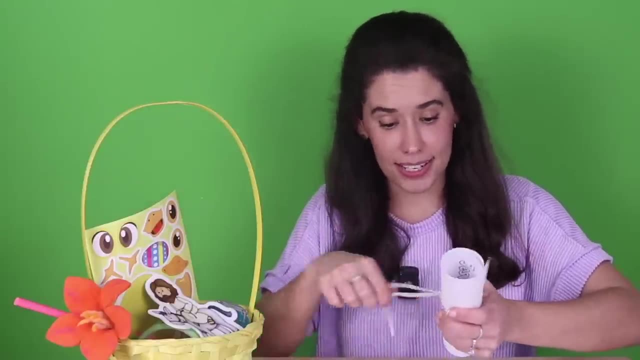 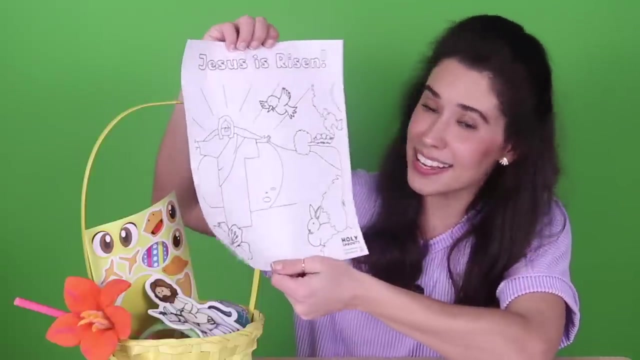 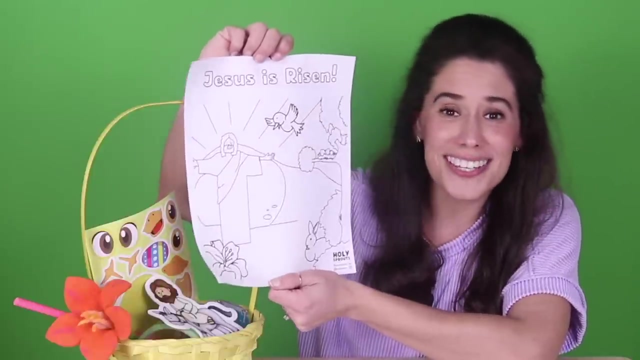 Let's look and see. Oh look, What is this? I think we need to open it. Let's open it. Oh wow, It looks like a coloring page. It's a coloring page with Jesus on it. Would you like to color with me? 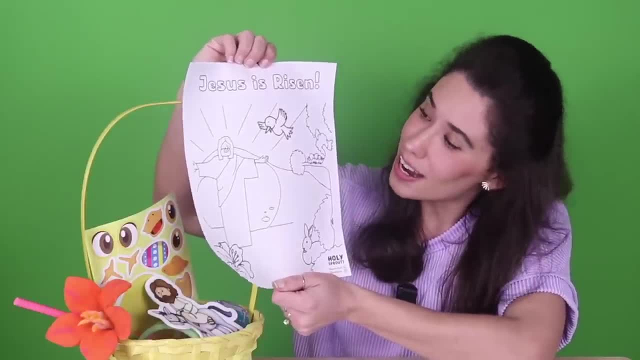 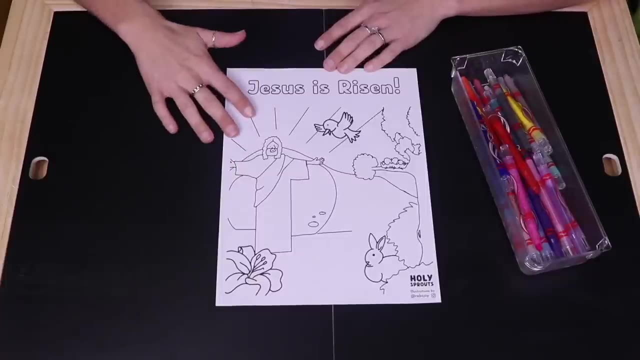 Yes, I would love to color with you. All right, let's go and color our page. I'm so excited that we get to color together today. If you have this coloring sheet, you can get it out so you can color with me. 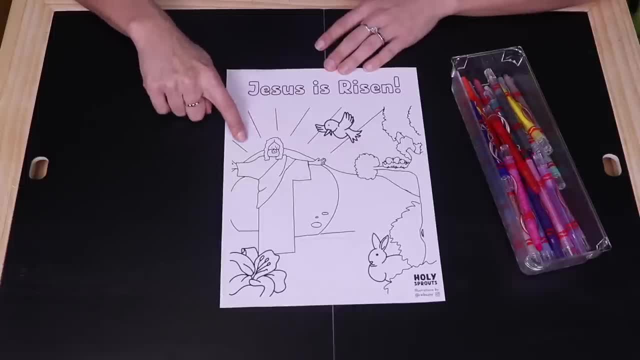 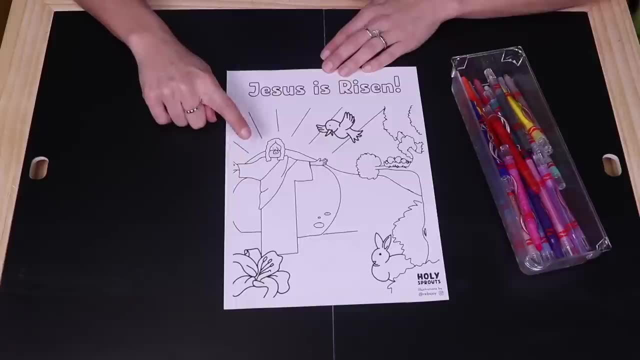 All right on our coloring sheet. look who we have right here. It's Jesus. It's Jesus after he was risen and came out of the tomb, And you know what That means? we get to be friends with him forever. That's so exciting. 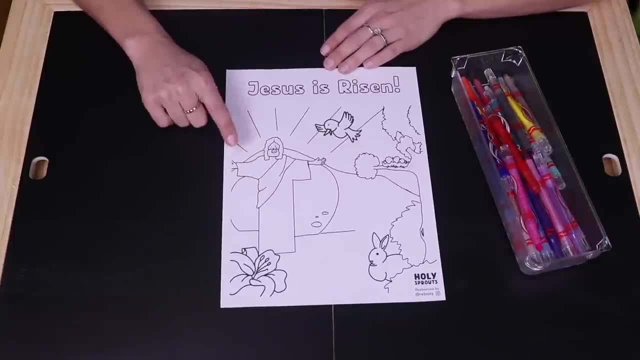 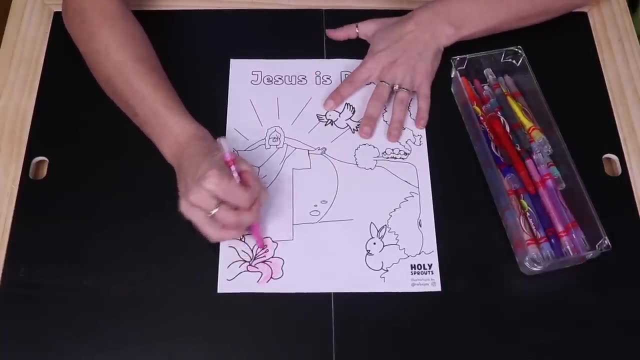 All right, let's color our coloring sheet. First, I am gonna color this beautiful flower right here in pink, a pretty pink right here for this flower. Look at that. Did you know that God made all the flowers and all the animals that we see on our earth? 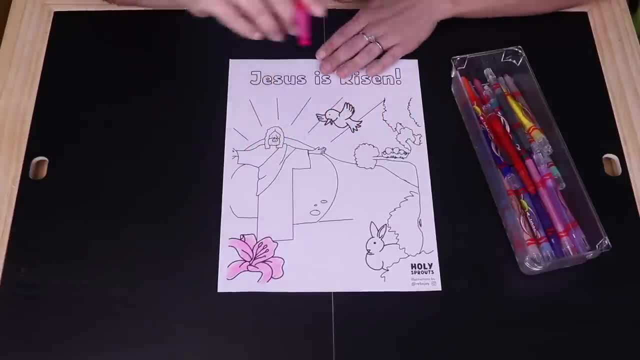 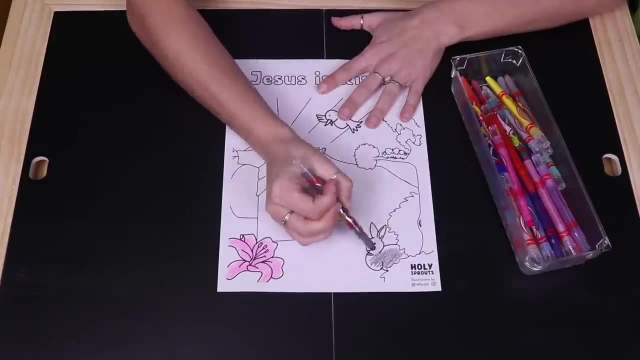 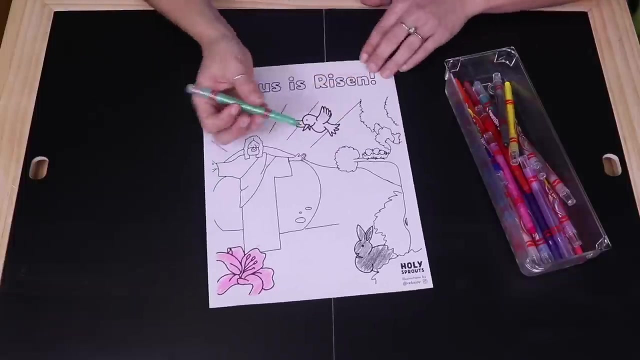 What a pretty flower. All right, I'm gonna do this little bunny hat. I'm gonna do this little bunny right here. He's gonna be black, A black little bunny. What a cute little bunny. All right, Now let's do these bushes green. 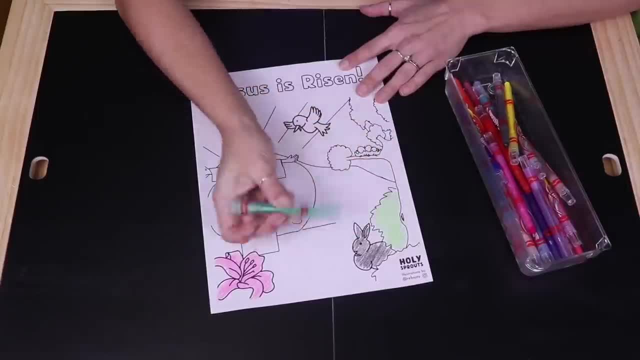 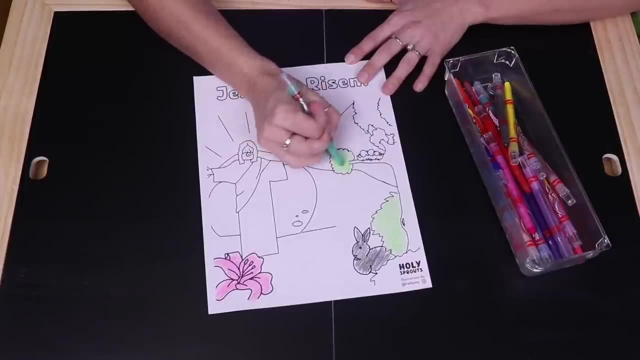 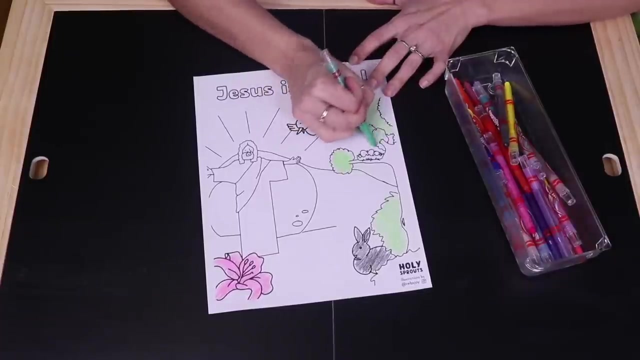 A pretty green, All right, All right, Look at that. For these bushes and leaves and for this tree right here, pretty green. It's springtime and all the animals are starting to come out and the leaves are coming out and the trees are growing, the flowers are growing. 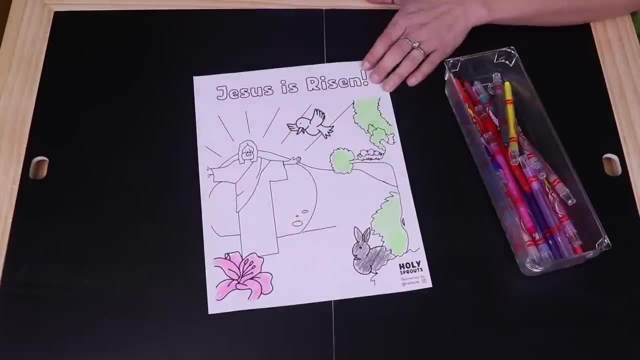 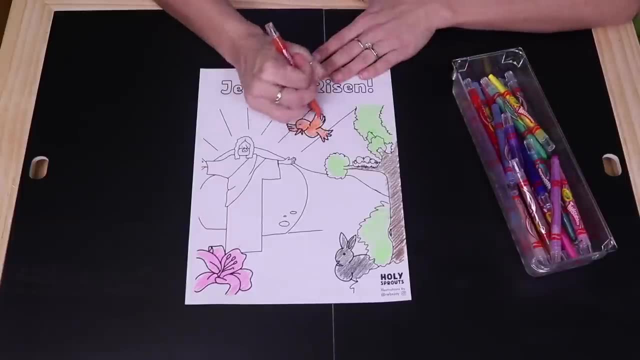 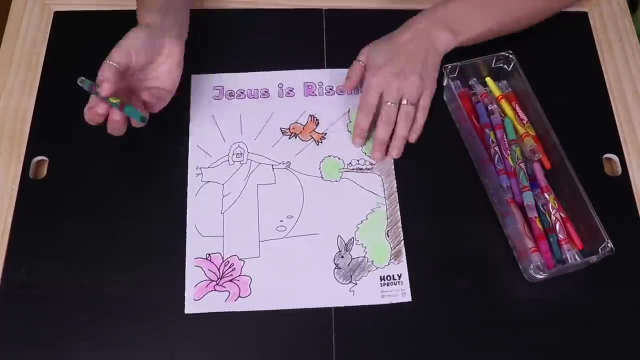 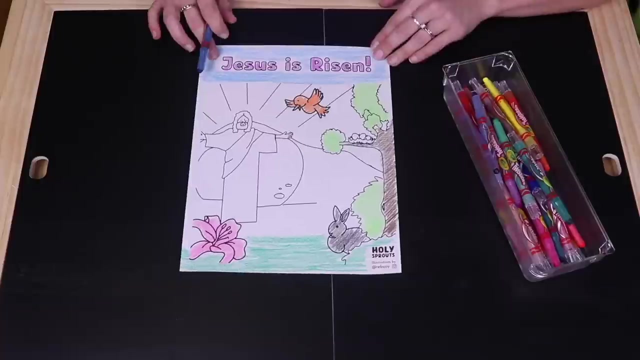 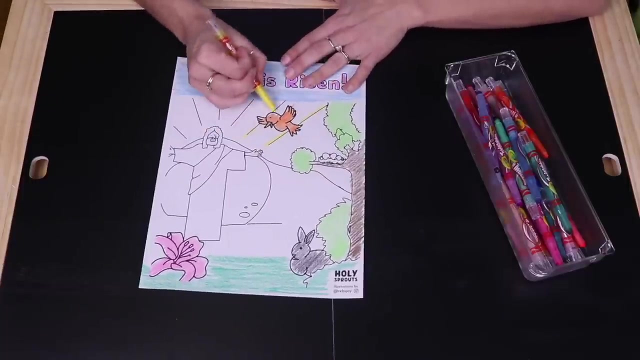 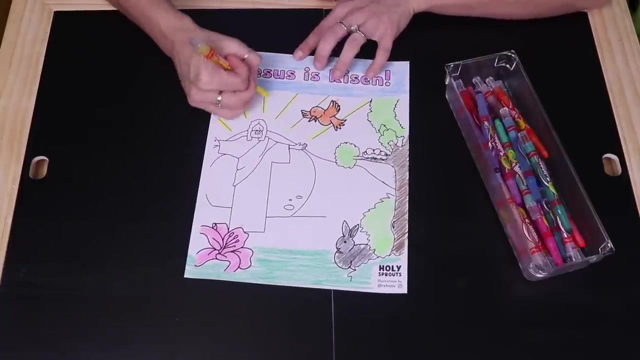 Everything's so beautiful. All right, there we go. See you next time, Bye-bye, okay. and you know what? jesus has some light coming off of him, so we are going to color these beautiful rays yellow. i'm gonna color these rays in yellow. there we go, let's see. 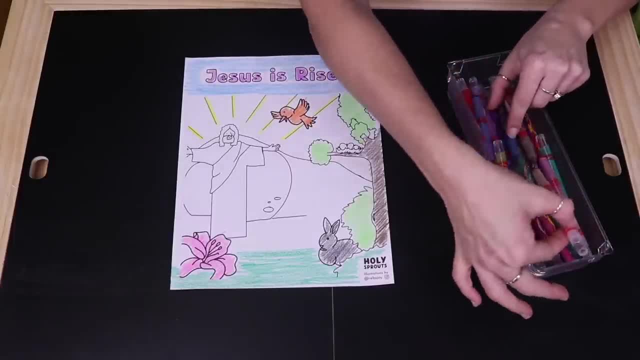 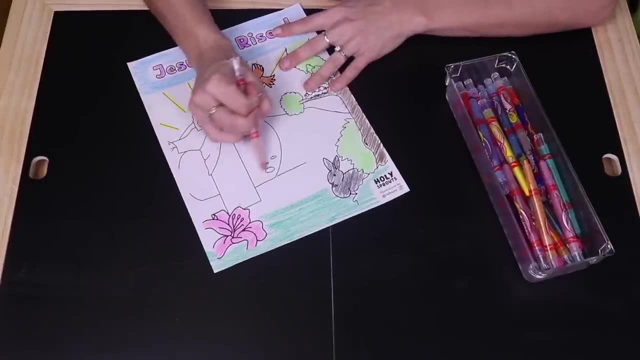 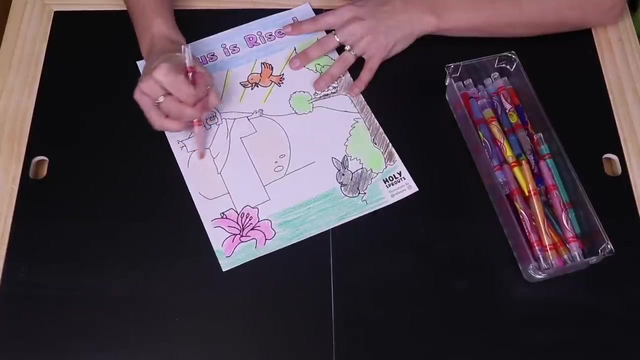 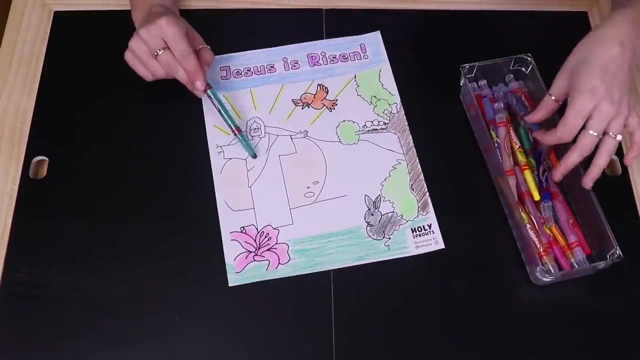 we could color. maybe there's a brown color. we can color the two in this kind of brown color right here. there we go, all right, and i think the last thing we have to color is jesus clothes. yes, let's color jesus's clothes. what color should we use? 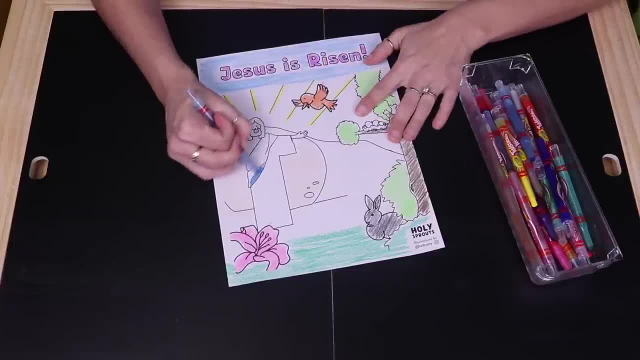 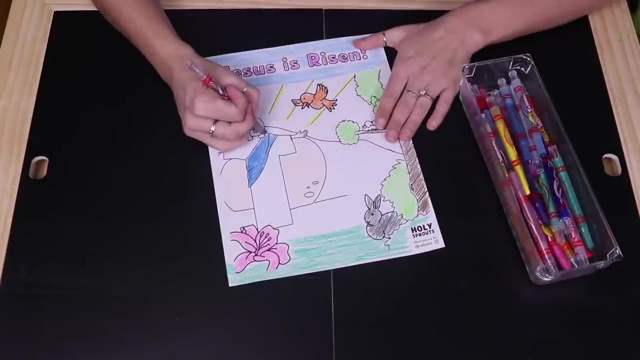 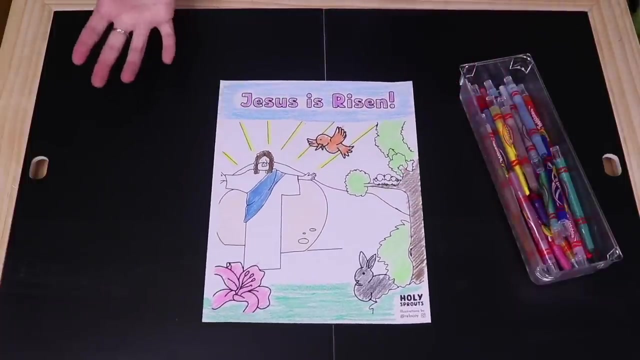 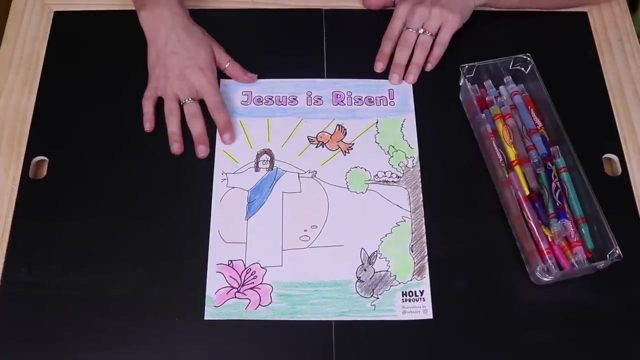 how about this blue? a little bit of a darker blue. there we go. that looks good. we could also color jesus's hair. actually, give him some brown hair and i think we're finished. wow, look at our coloring sheet. it looks beautiful. it looks so beautiful. i'm sure your coloring sheet looks so beautiful too. thank you so much for coloring jesus. 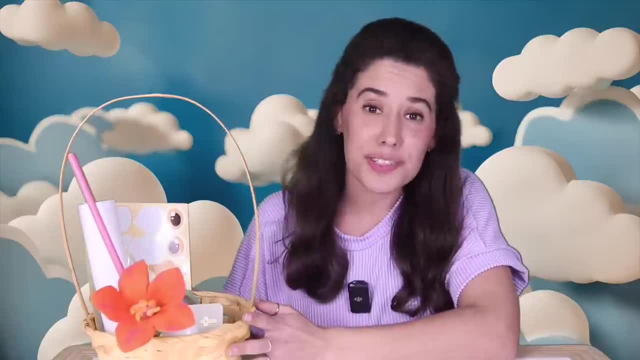 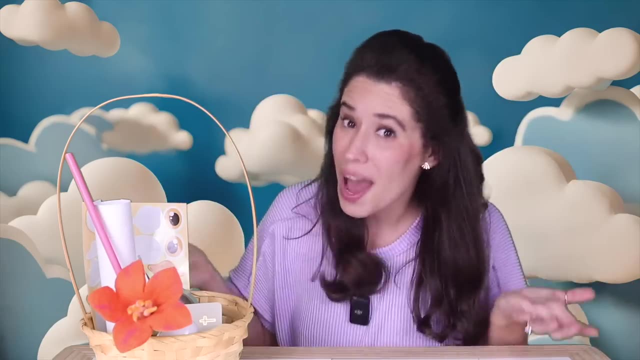 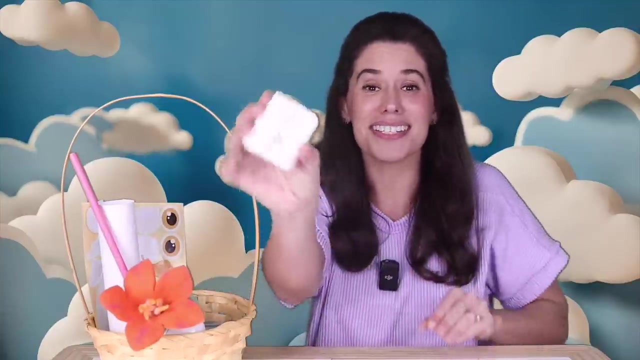 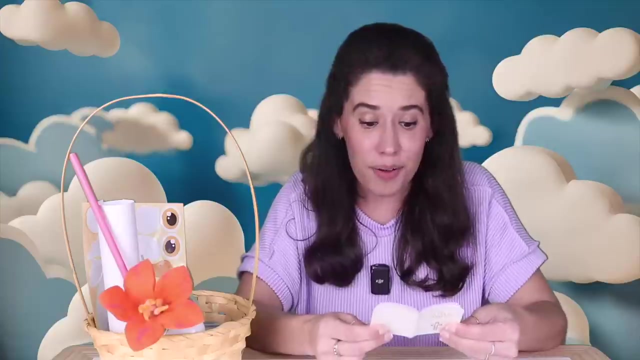 with me. let's see what else we have in our basket. what's in the basket? what could it be? what's in the basket? let's look and see. wow, it's our teeny tiny bible. our teeny tiny bible. and now we can read our bible verse for today. 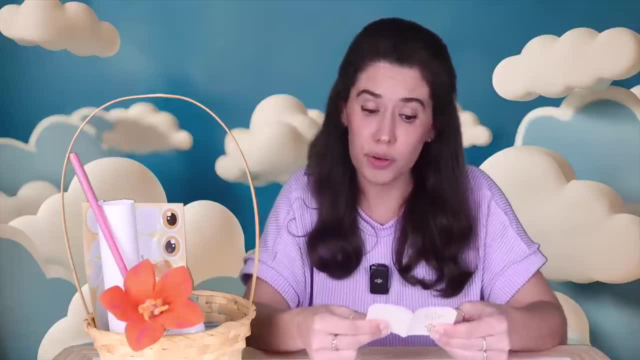 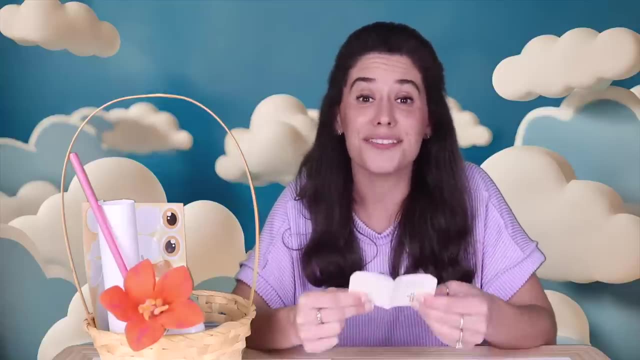 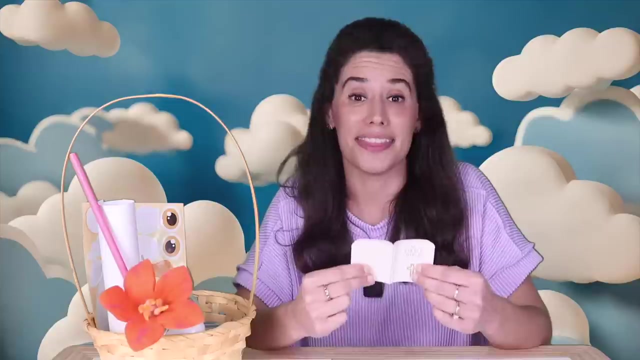 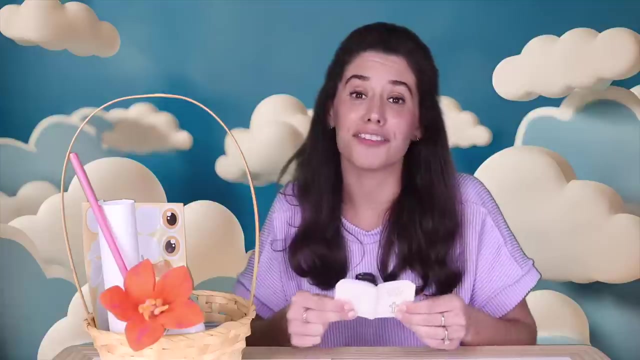 our bible verse for today is luke 24: 6, and it says: he is not here, he is risen from the dead. he is not here, he is risen from the dead. and that verse is talking about jesus: how jesus was risen from the dead and is alive for us today. wow, what a wonderful verse. 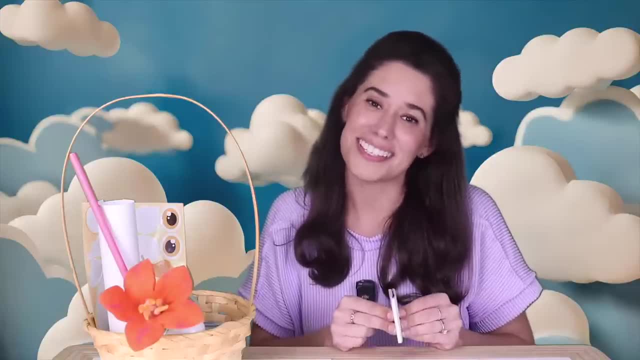 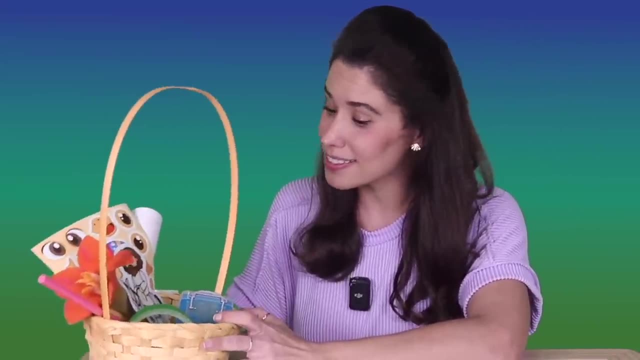 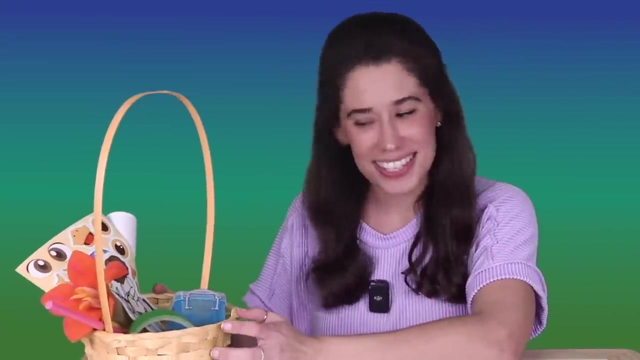 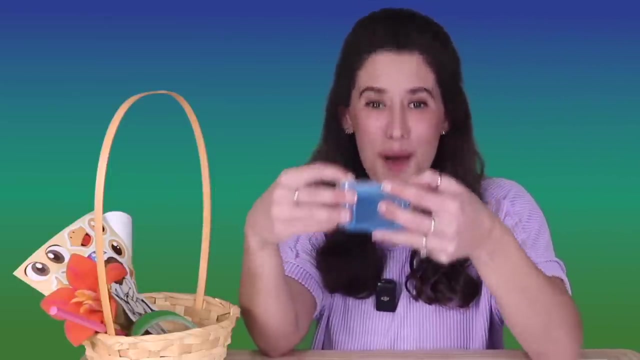 that is so exciting to know that Jesus is alive. all right, let's get something else out of our activity basket. what's in the basket? what could it be? what's in the basket? let's look and see. I see a blue box. a blue box. yes, let's open it. 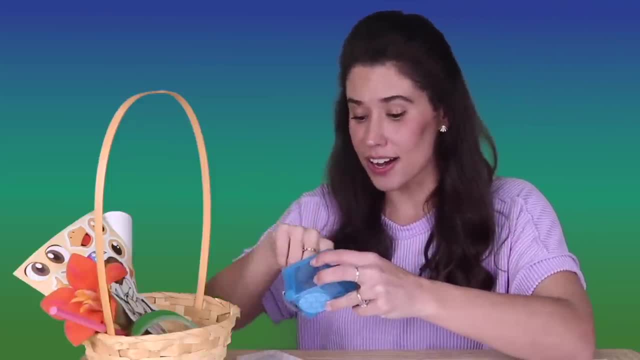 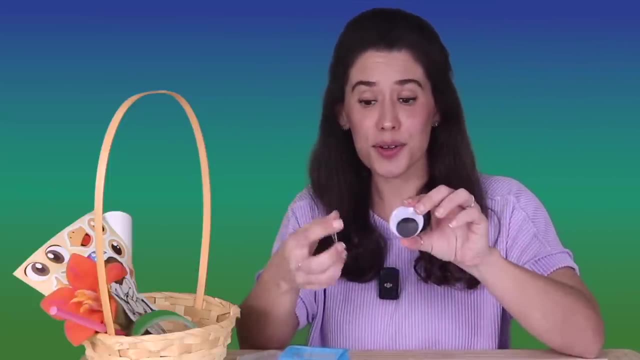 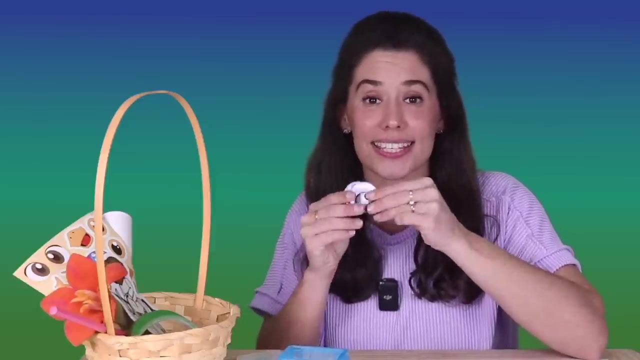 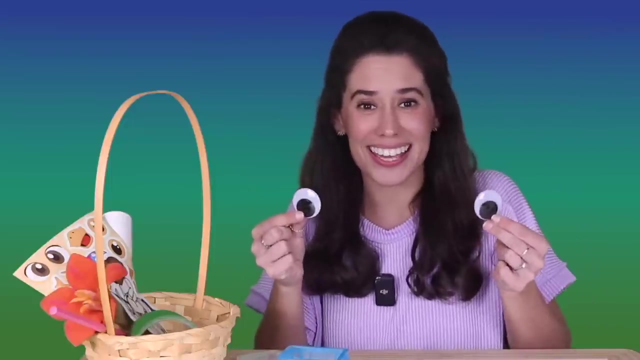 and see what's inside. all right, let's take it out. let's take it out. I see two eyes, two funny eyes. you know what I think these eyes are for? I think these eyes are to play the game I spy. yes, would you like to play the game with me? 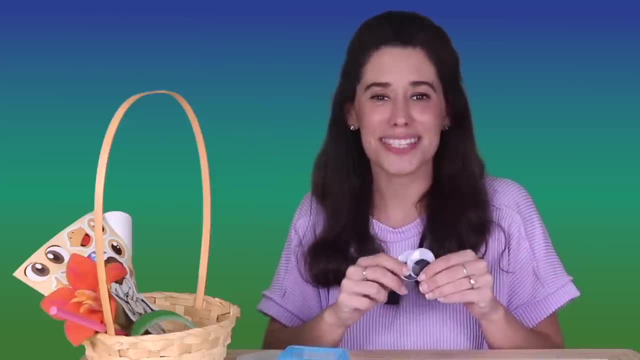 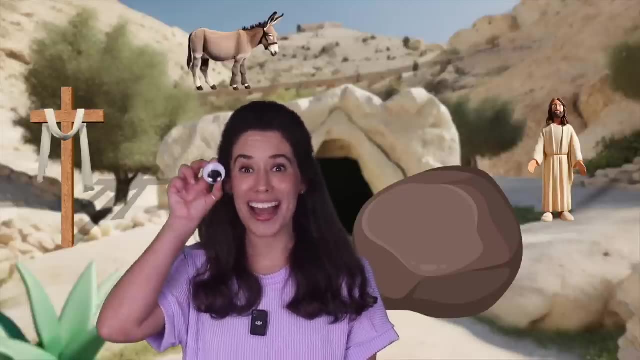 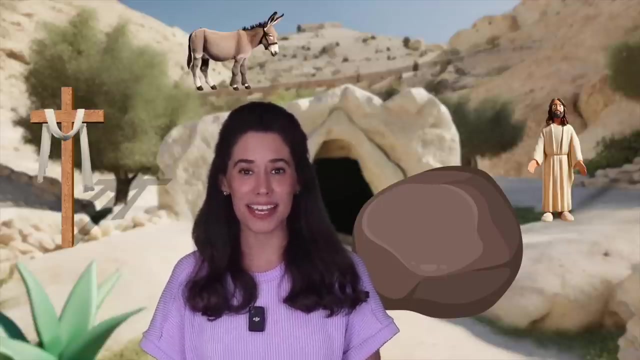 yes, you would. all right, let's go play the game. I spy, all right, I spy with my little eye something beginning with the letter D. that's right, something beginning with the letter D. do you know what it is? yes, it's a donkey. a donkey. do you see a? 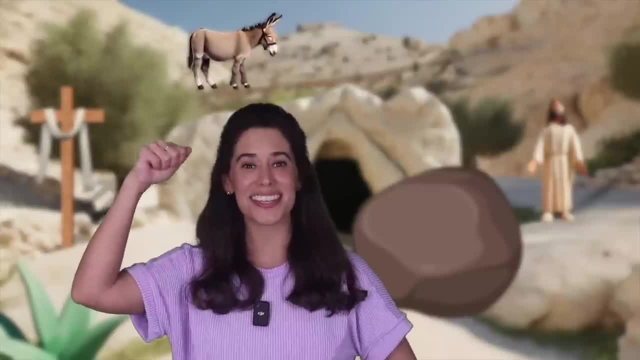 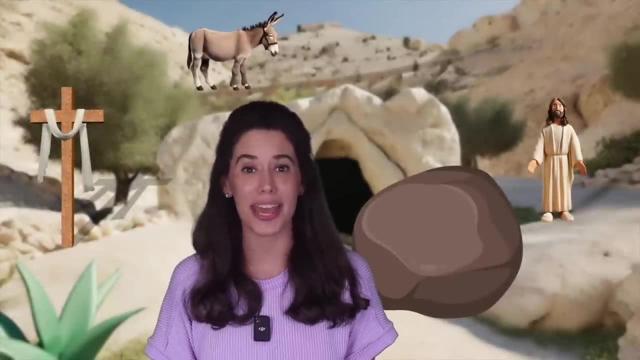 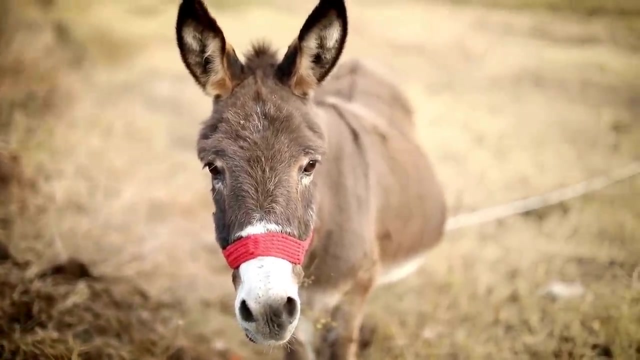 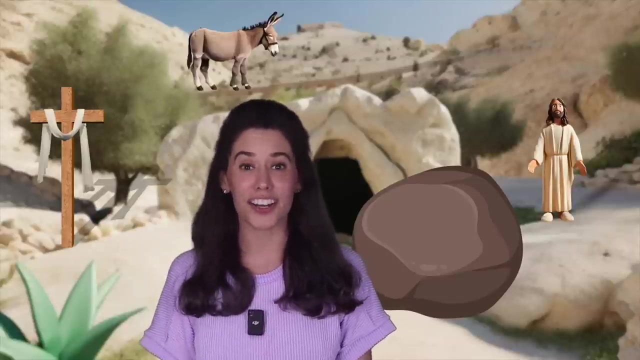 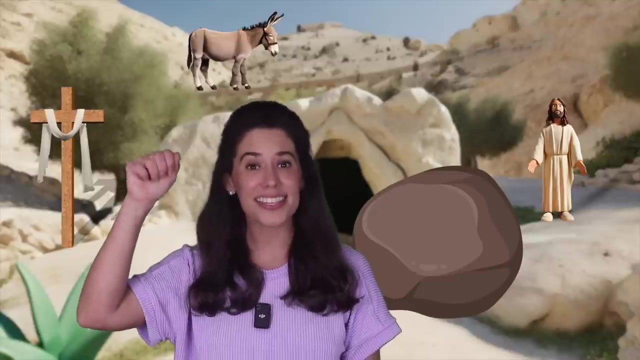 donkey anywhere. yes, there it is the donkey. good job, it's just like the donkey that Jesus rode on when he came into Jerusalem. I spy, who is my little eye? something beginning with the letter s s. do you know what it is? yes, that's right, it's stone. 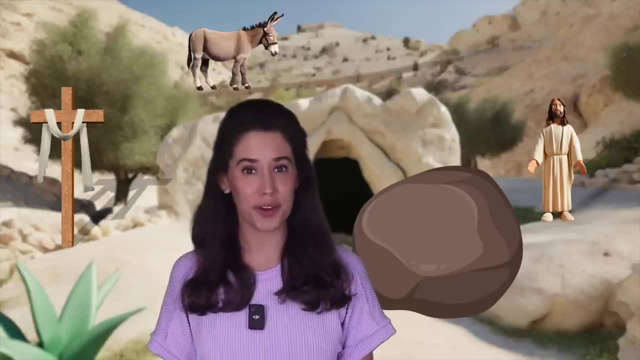 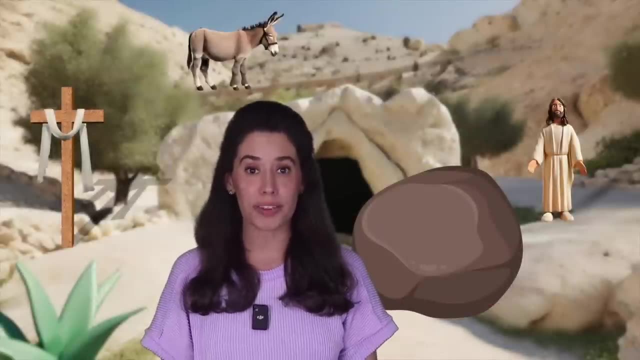 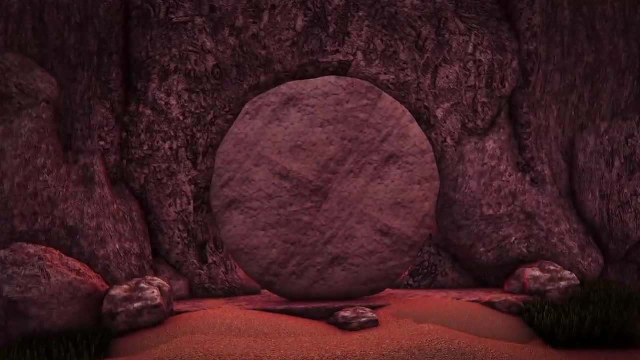 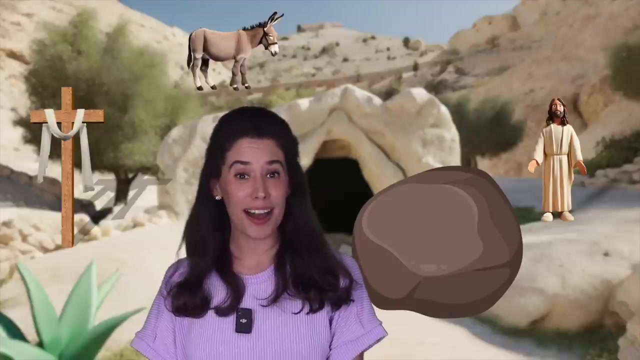 I see a stone. do you see a stone? yes, there, it is good job. it's like the stone that was rolled away from the tomb in the Easter story. all right, I spy with my little eye. something beginning with the letter C. all right, I spy with my little eye. something beginning with the letter C. 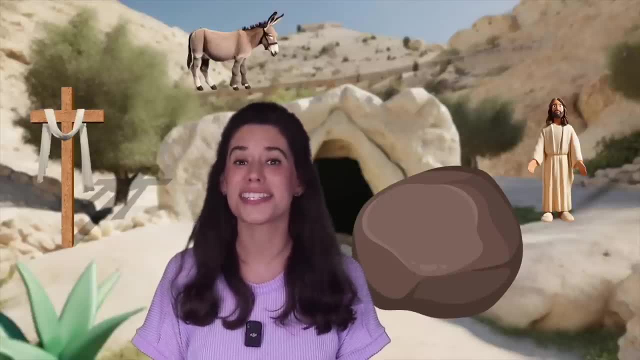 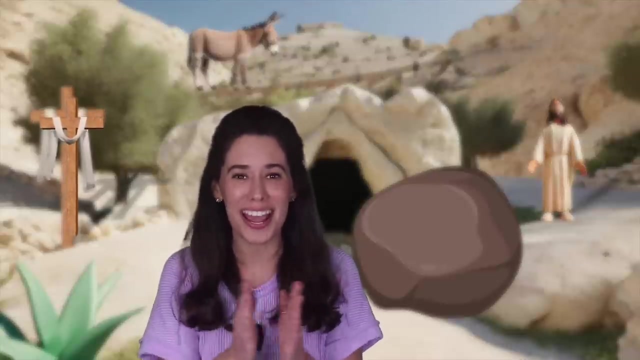 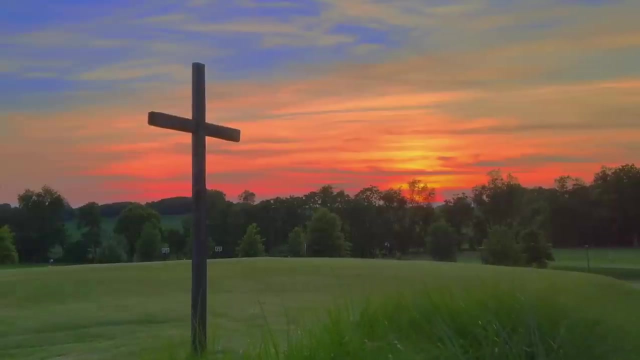 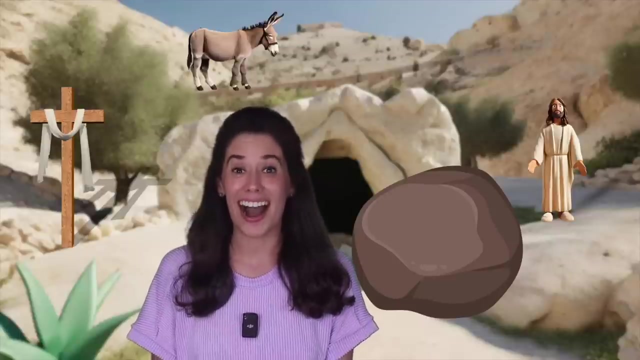 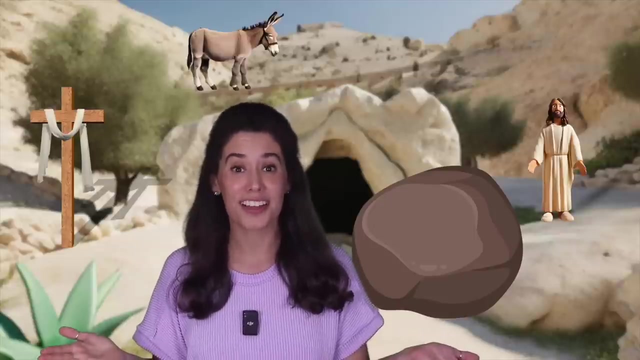 see something beginning with the letter C. do you know what it could be? yes, you're right, it's a cross. a cross, yes, and there it is great job. that is like the cross that Jesus died on for us. you, you was- I spy with my little eye. something beginning with the letter J. yes, the. 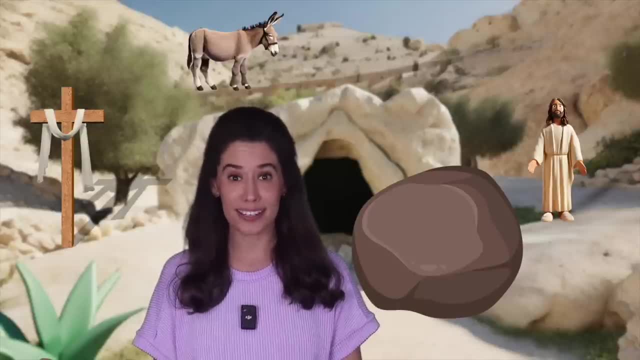 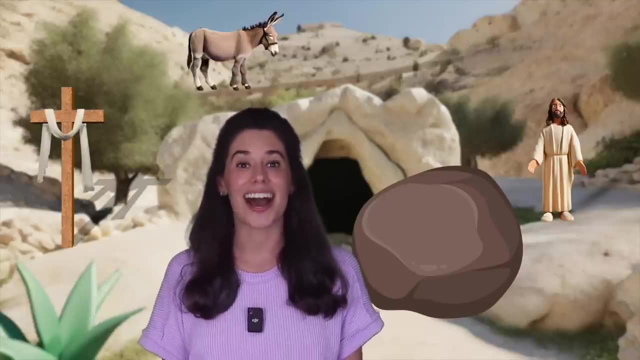 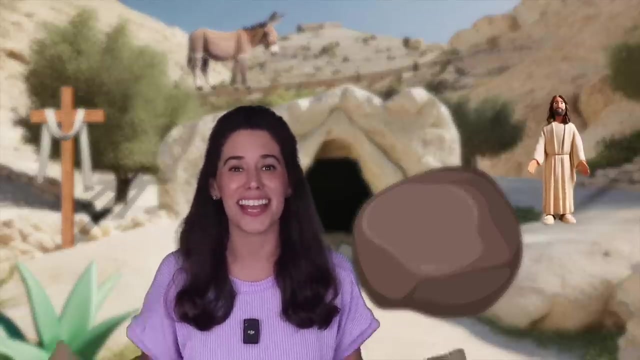 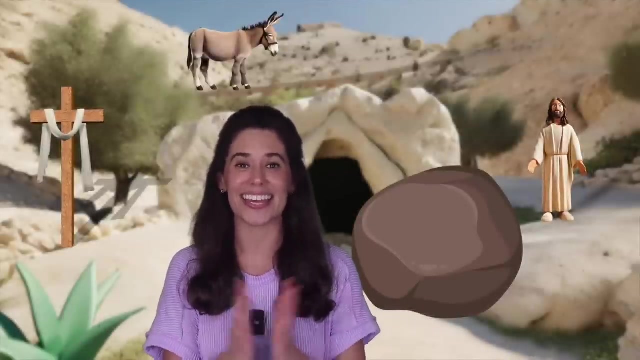 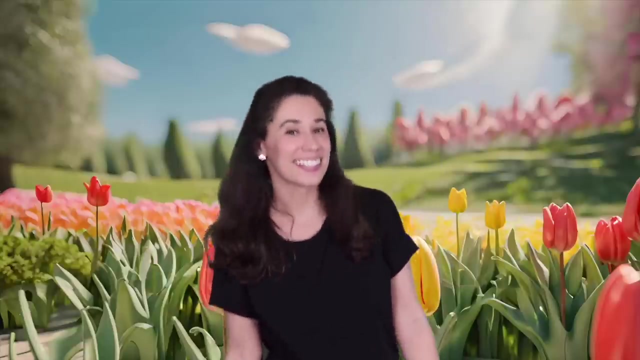 letter. j do you know what it could be? do you know? yes, Jesus, yes, I see Jesus. can you find him? do you see Jesus? yes, and there he is. There's Jesus, and he is alive. Yay, Can you jump, jump, jump, Jesus is alive. 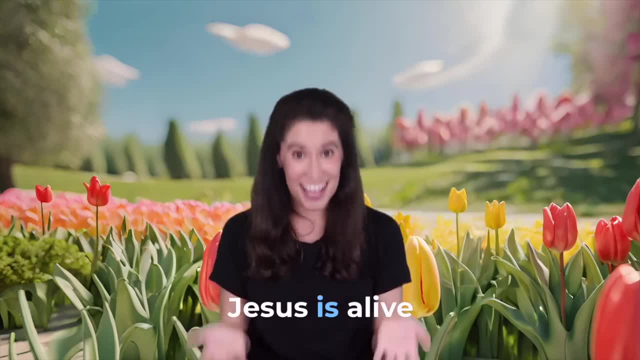 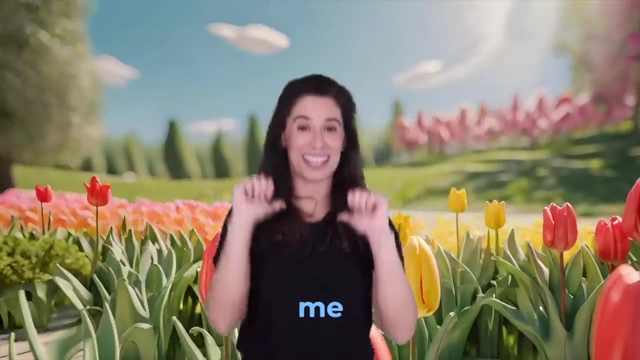 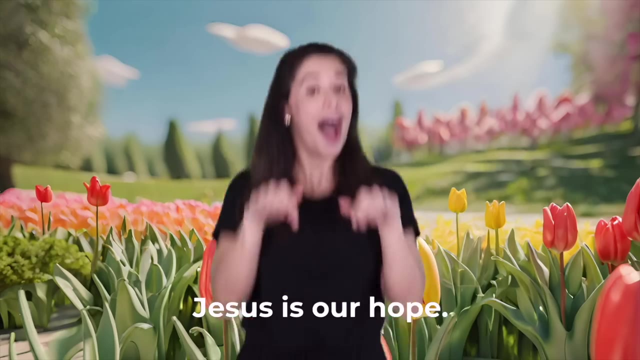 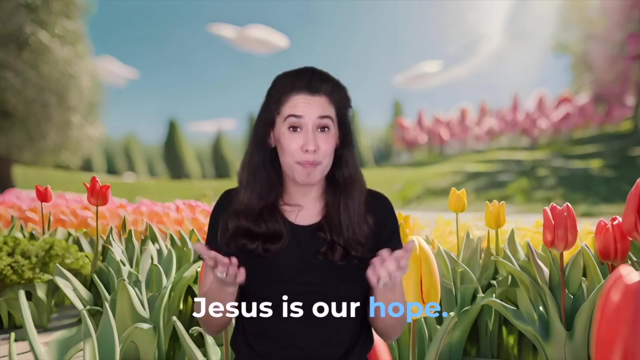 Jump, jump, jump. Jesus is alive. Jump, jump, jump, Jesus is alive. Jump around with me, Can you hop, hop, hop, Jesus is our hope. Hop, hop, hop, Jesus is our hope. Hop, hop, hop, Jesus is our hope. 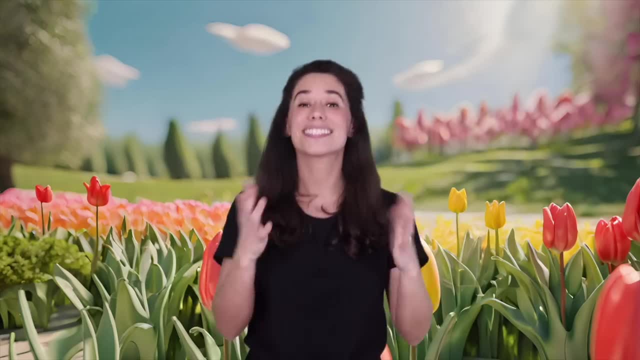 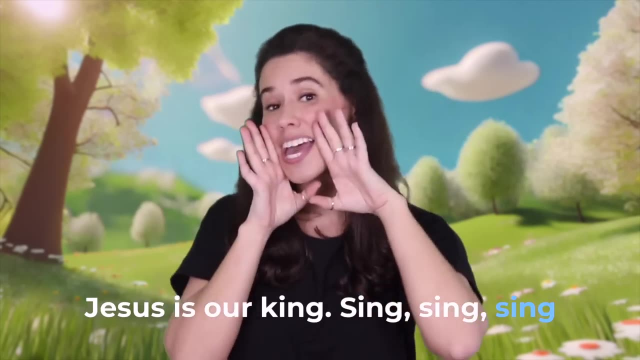 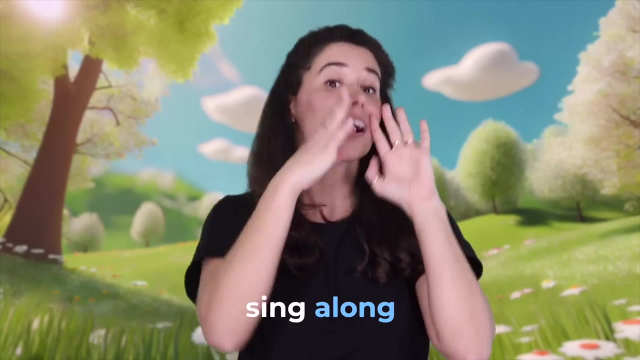 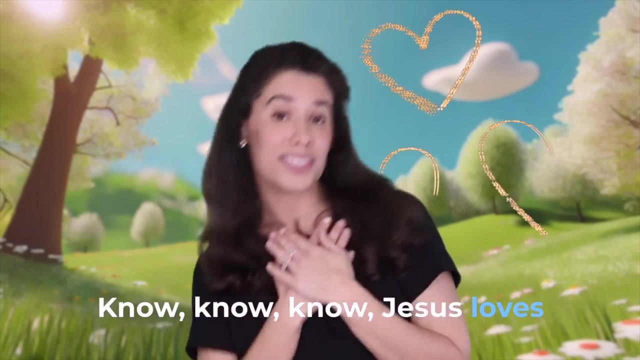 Hop along with me. Can you sing, sing, sing? Jesus is our King. Sing, sing, sing. Jesus is our King. Sing, sing, sing. Jesus is our King. Sing along with me, Sing along with me. Did you know, know, know, Jesus loves you so. 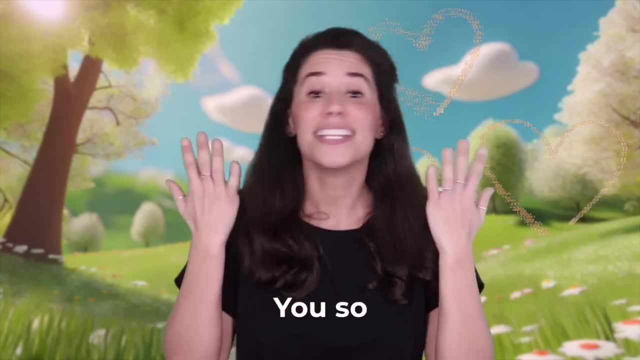 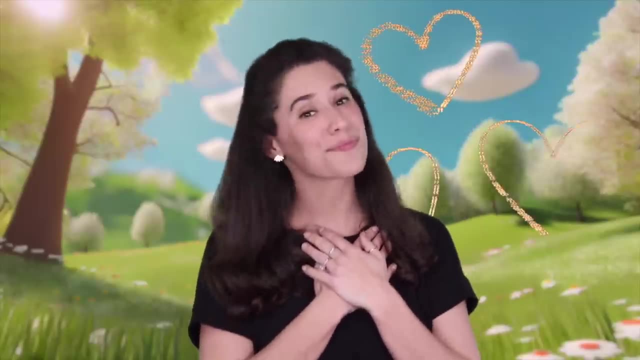 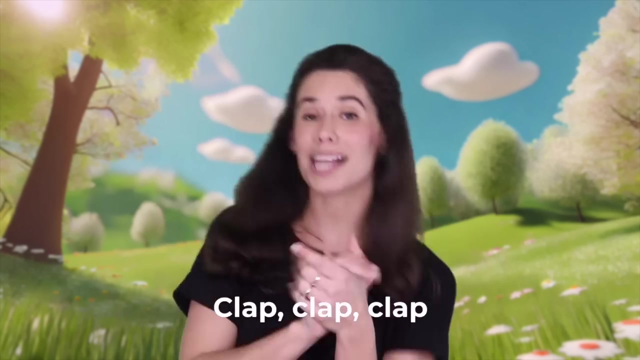 Did you know Jesus loves you? so Did you know Jesus loves you? so Jesus loves you. so Can you clap, clap, clap, he is coming back. Clap, clap, clap, he is coming back. Clap, clap, clap, he is coming back. 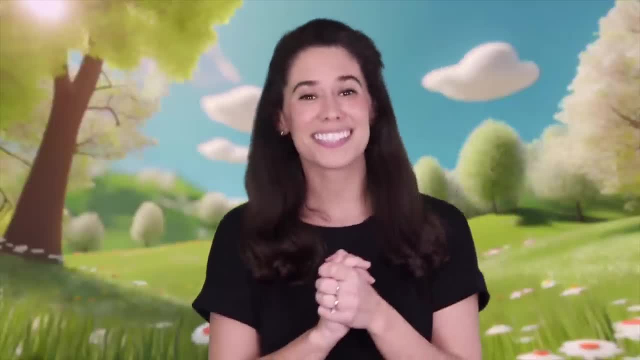 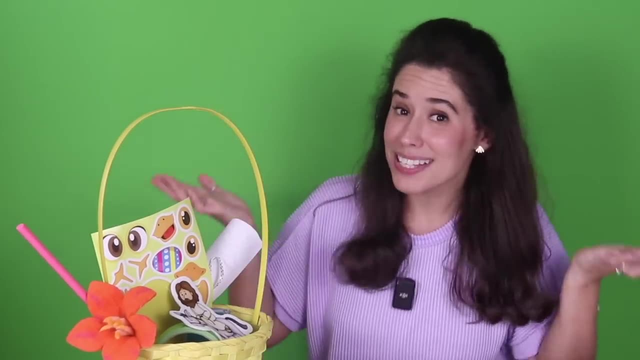 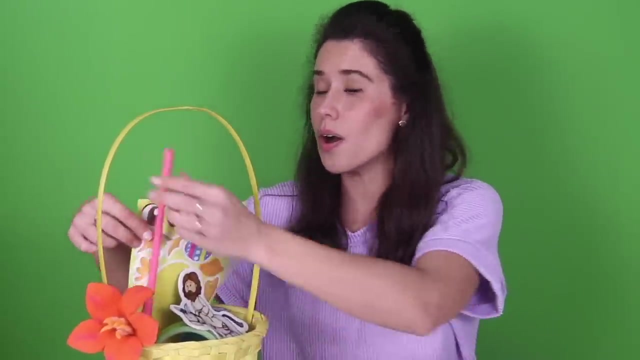 Clap your hands with me. Let's see what else we can pick out of our activity basket. What's in the basket? what could it be? What's in the basket? let's look and see. Hmm, oh, I see a pink spoon. 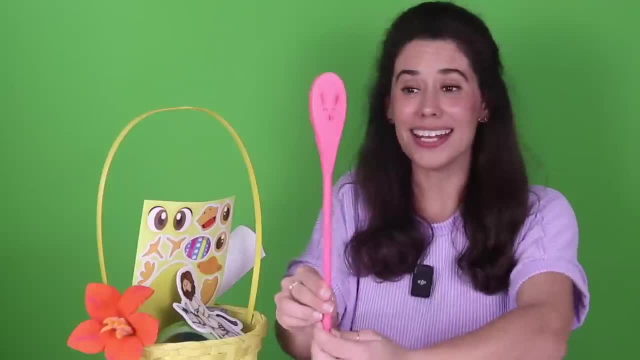 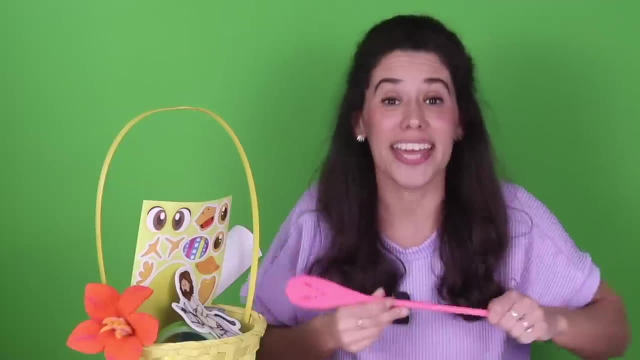 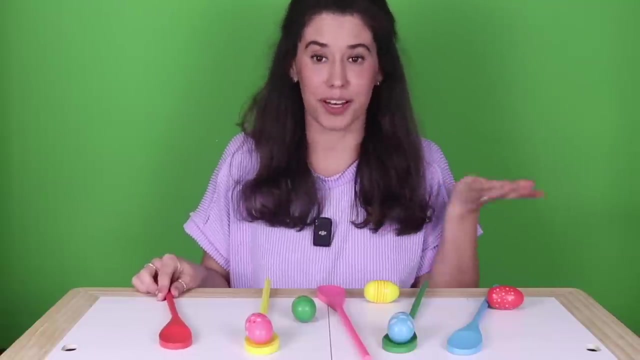 Yes, I see a spoon And it has a little bunny on the side. Look at that, what a cute little bunny face. Alright, I can't wait to see what activity we're going to do with our spoon. Come on, Wow, I have some colorful spoons right here. 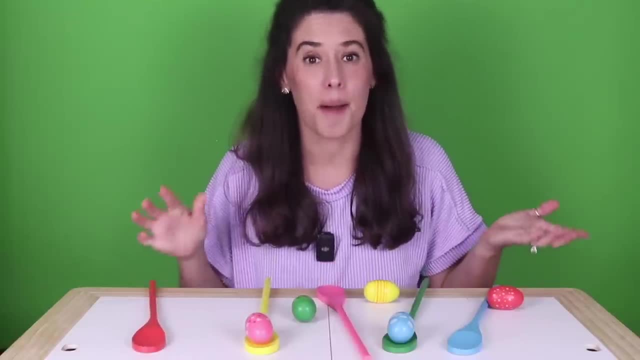 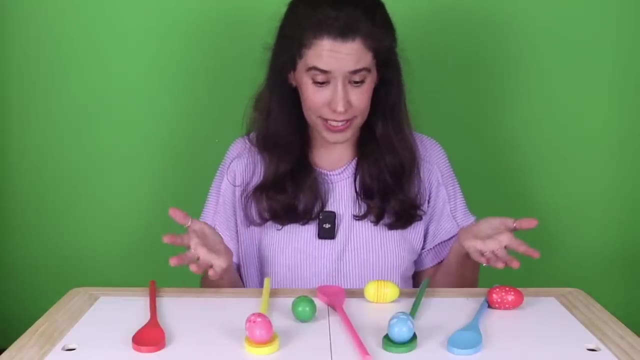 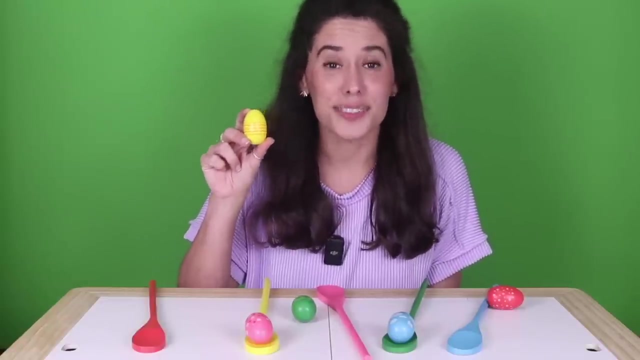 And some colorful eggs. But you know what? The eggs and the spoons are in the wrong place. We need to try and match the colored eggs with the right colored spoon. Alright, Would you like to help me? Can you help me? 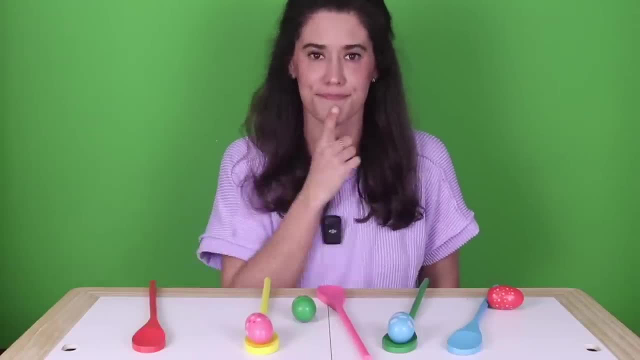 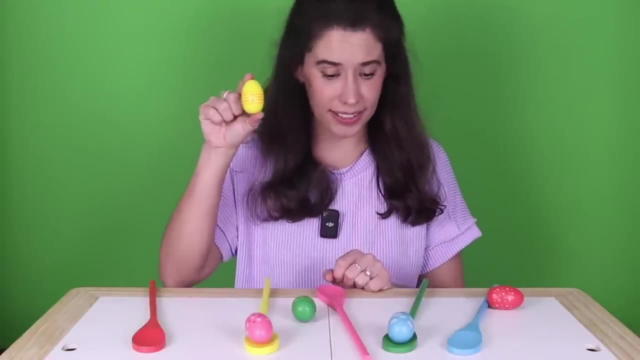 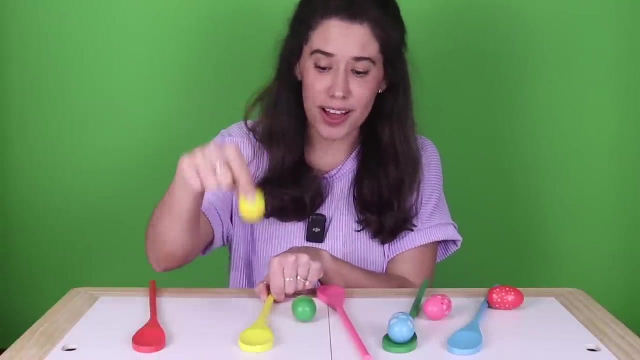 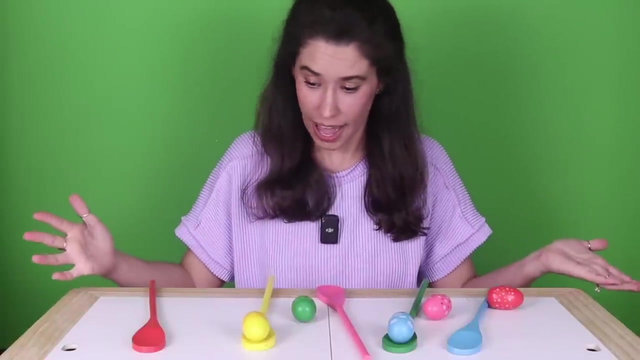 Yes, Alright, let's get started. Hmm, let's see, We have a yellow egg. The yellow egg needs to go on the The yellow spoon. that's right, The yellow egg goes on the yellow spoon. Good job, Alright. what else do we have? 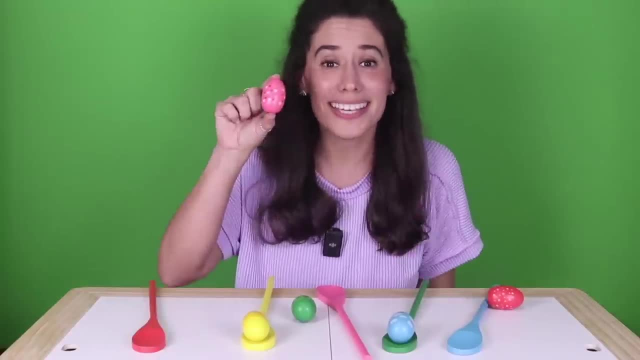 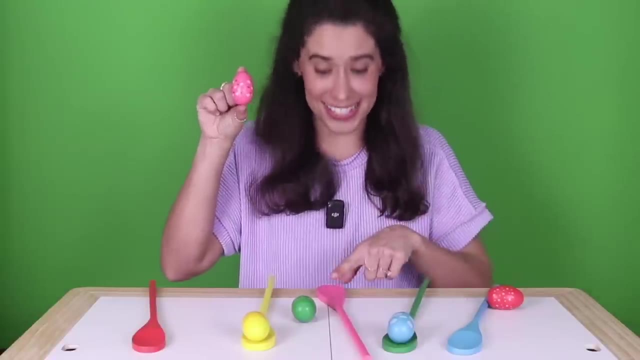 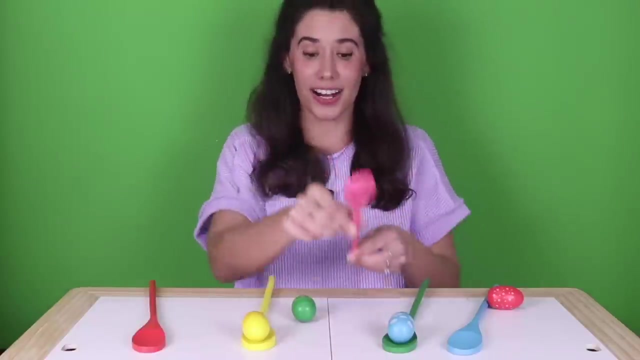 Hmm, let's see, We've got a pink egg. Do you see a pink spoon, Do you? Yes, it's right here. This pink spoon has a bunny on it, The cute little bunny. Alright, let's put our pink egg. 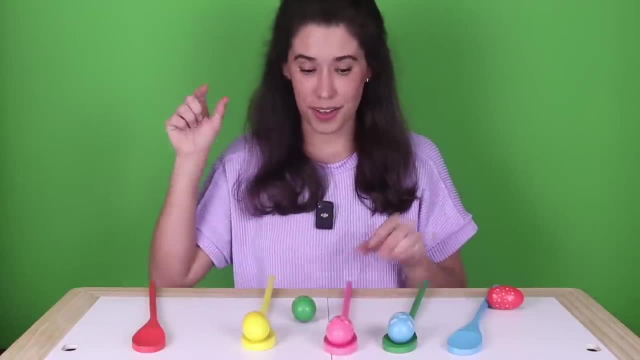 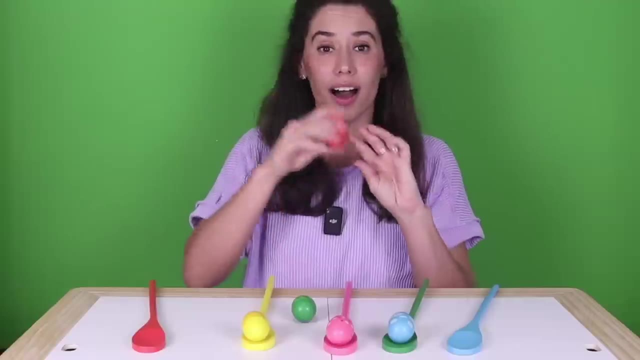 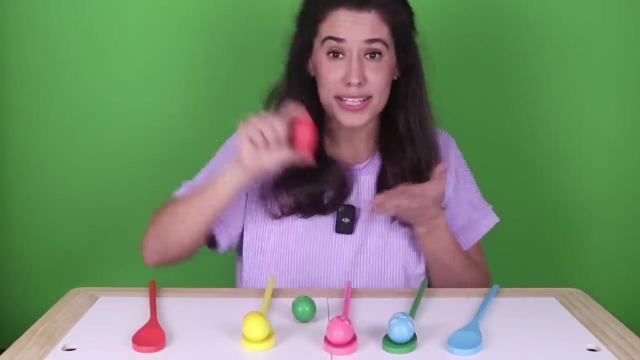 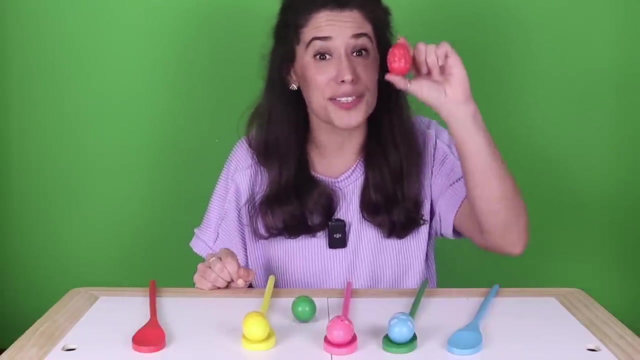 on our pink spoon. Alright, Thank you. Let's see what else. I have a red egg. This egg is red, Red. And what spoon do you see here that goes with the red egg? Do you see a spoon that matches the red egg? 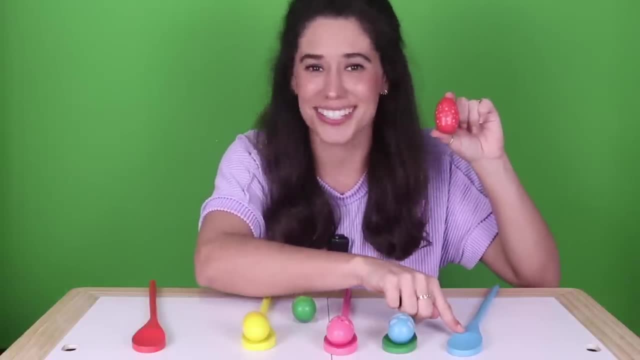 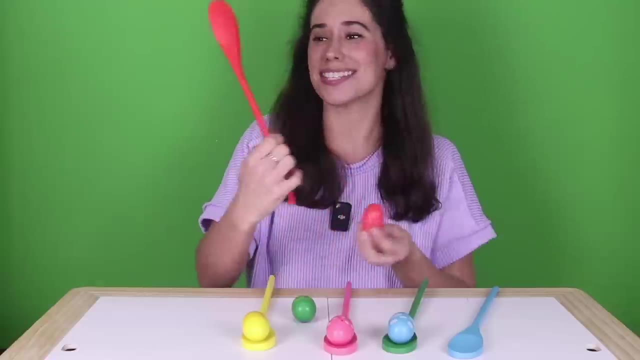 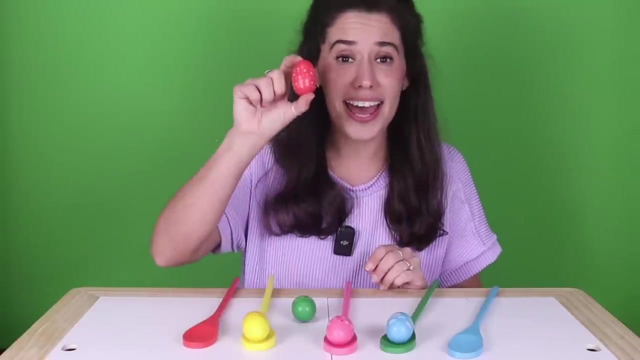 Is it this one? No, it's not that one, It's, Yes, This one. right here, This little spoon has a duck face, A cute little duck face, And our red egg goes on the red spoon. Yay, Thank you. 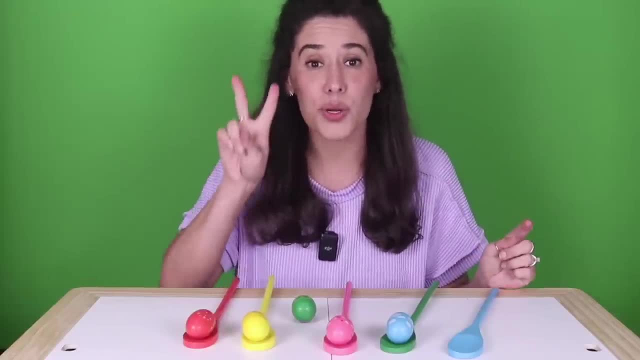 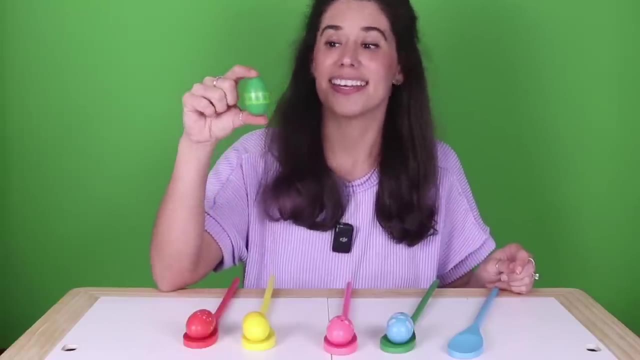 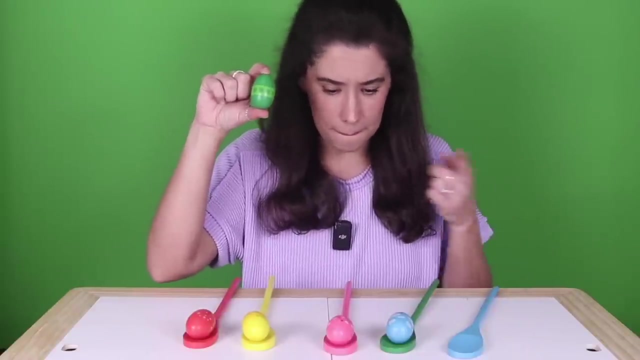 for helping. Alright, we have two left. I see here a green egg, Yes, a green egg. Do you see the spoon where the green egg could go? Hmm, I see it, but it has a blue egg on it, Silly blue egg. 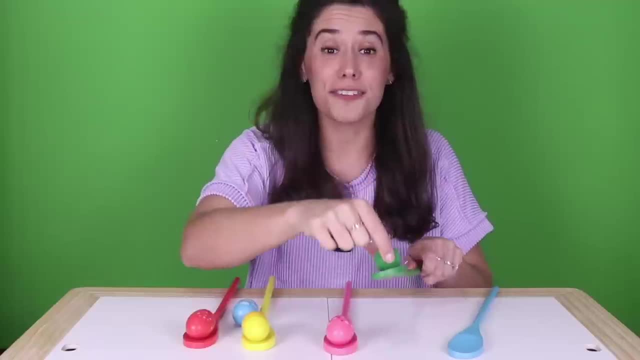 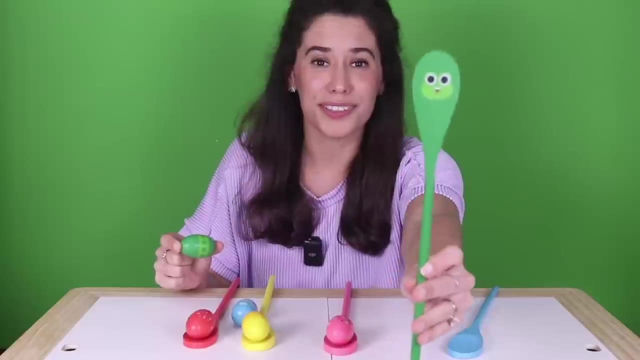 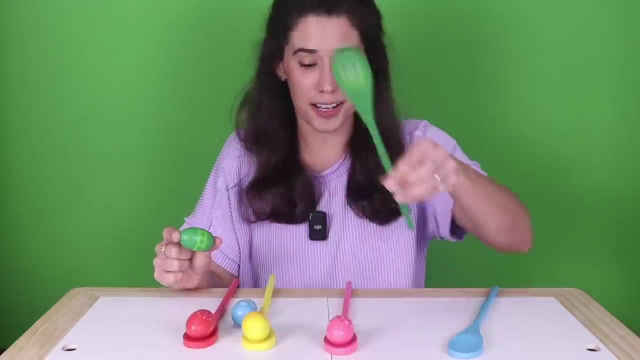 You can't be there. This is for our green egg. Yes, the green egg goes on the green spoon. And this little spoon looks like a green frog: Ribbit, Ribbit, Ribbit, Cute little green frog. Our green egg goes on. 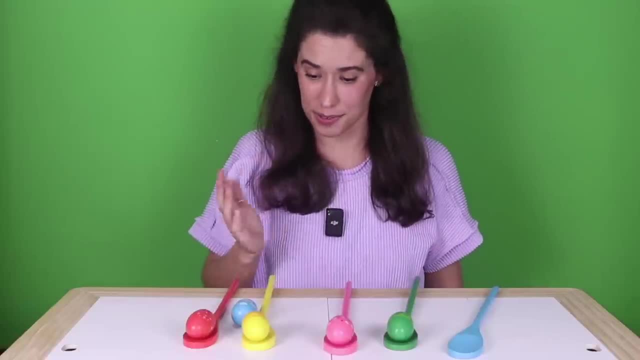 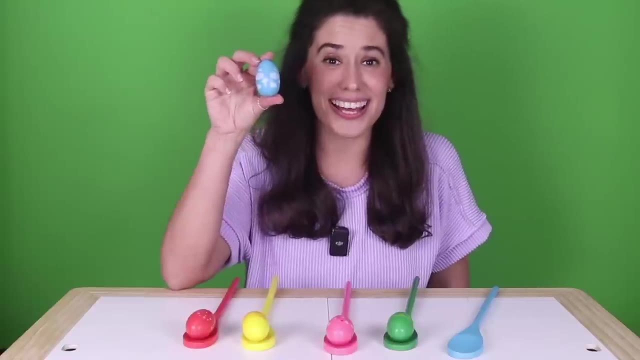 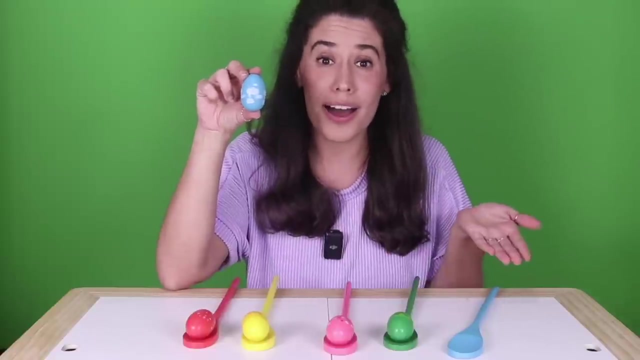 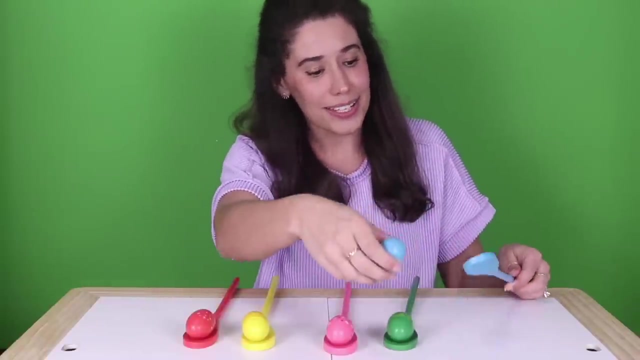 the green spoon. Thank you, Alright, the last one we have is the blue egg. That's right, the blue egg. And the blue egg goes on. the which one? Yes, The blue spoon. Good job, Let's see, the blue spoon has. 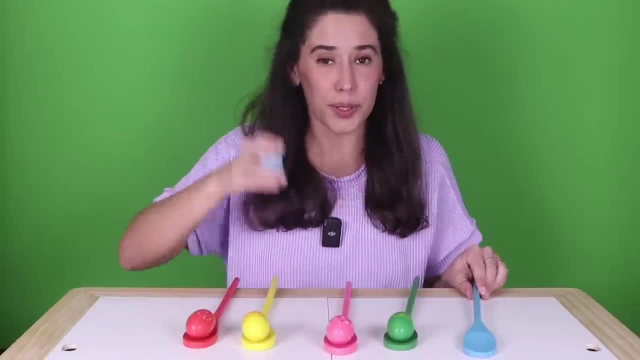 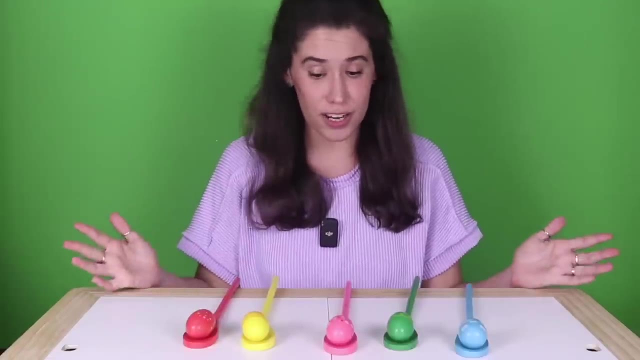 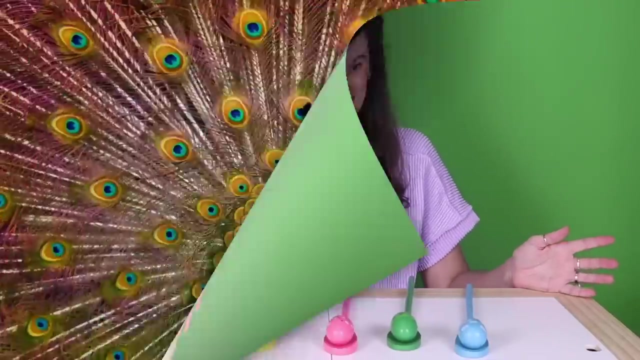 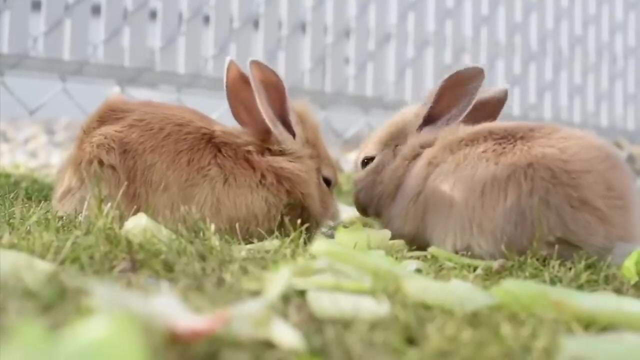 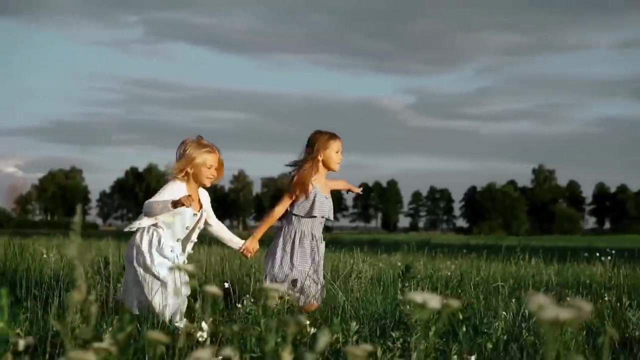 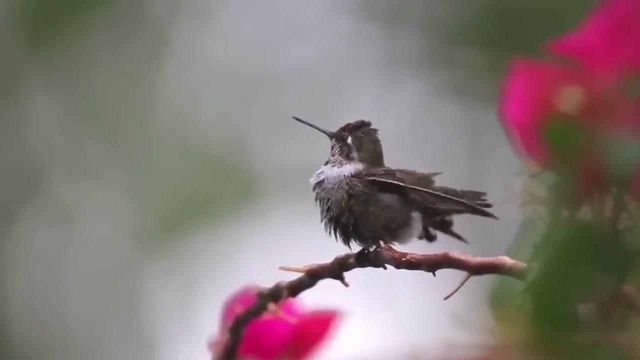 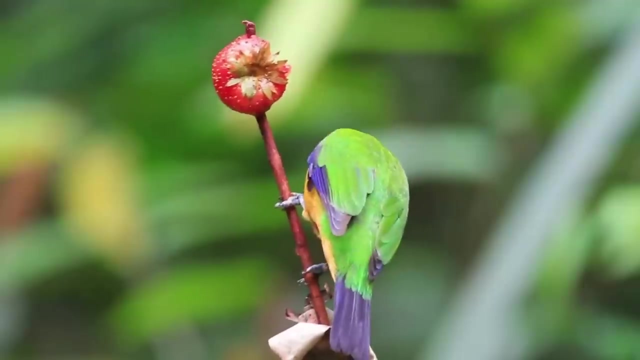 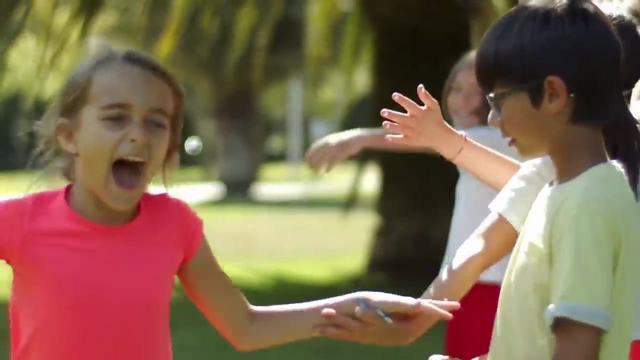 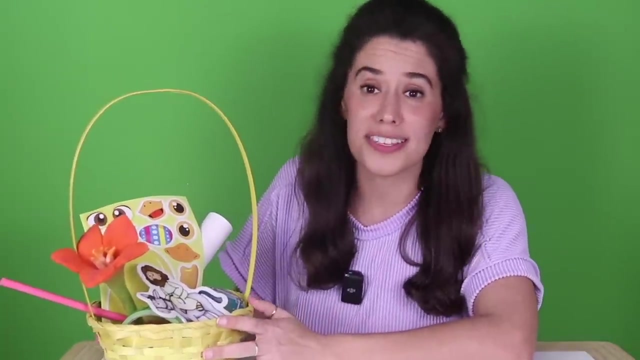 a little cloud on it, The blue egg goes on the blue spoon. Good job. Thank you so much for helping me match the eggs with the right spoon. That was lots of fun. I think we have a few more things that we haven't looked. 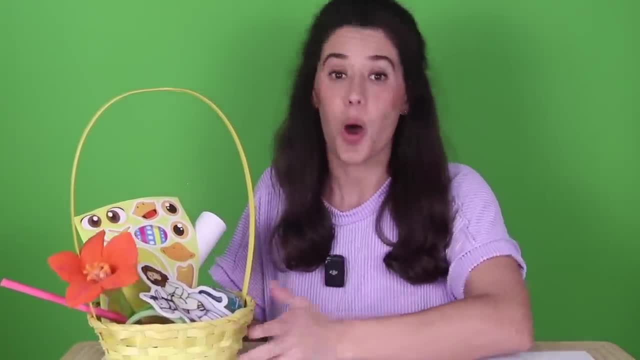 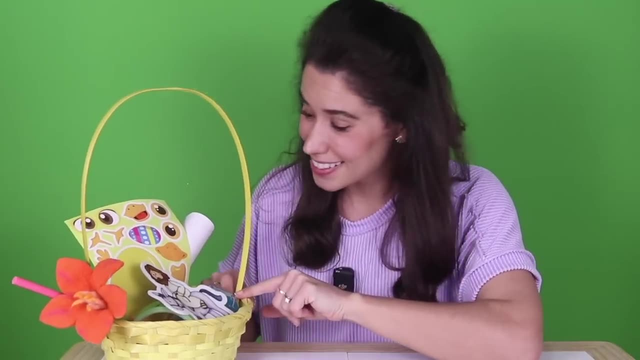 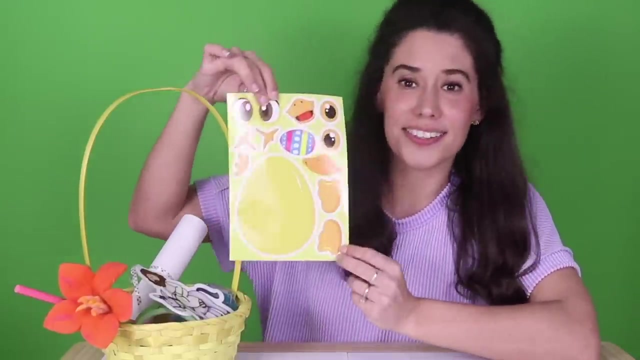 at in our basket. What's in the basket? What could it be? What's in the basket? Let's look and see. Wow, I see a sticker page. Yes, I think it kind of looks like a duck. Yes, a sticker page. 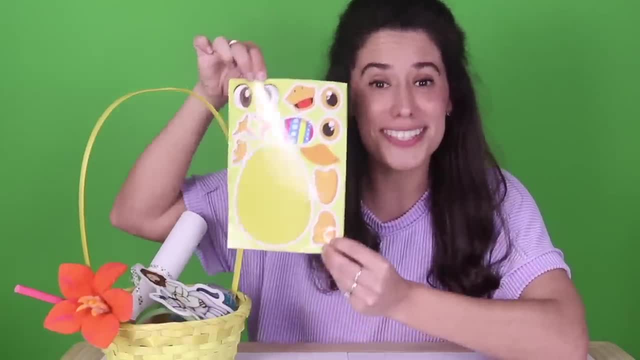 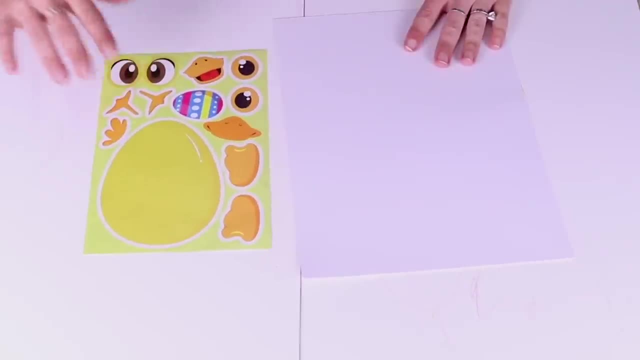 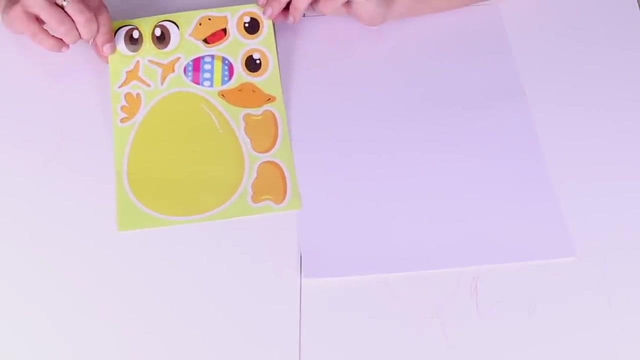 Why don't we go and see what we're going to do with our fun sticker page? Alright, come on, I have a blank sheet of paper and the duck sticker so we can work on our duck together And our duck. did you know that they come out of? 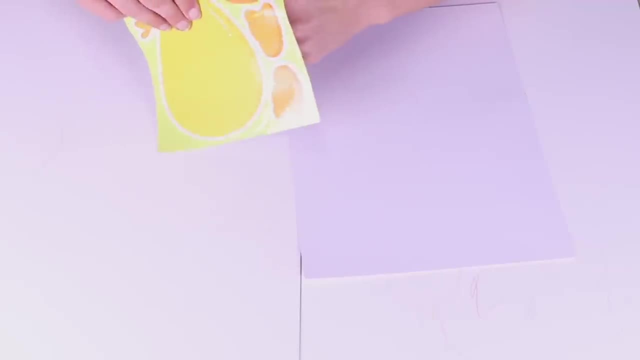 eggs. That's right. Ducks come out of eggs. They hatch In the springtime. they come to life, Just like Jesus came back to life at Easter time. Alright, here is our egg. Let's see which I should we use for our duck. 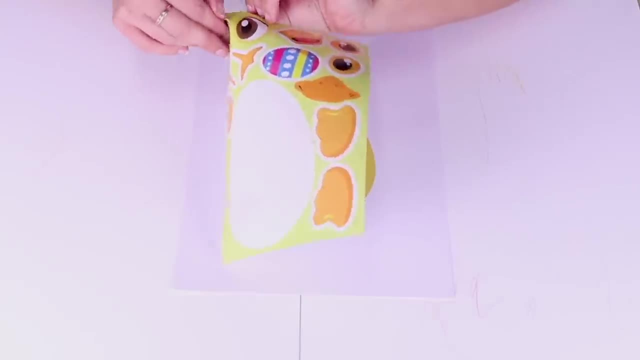 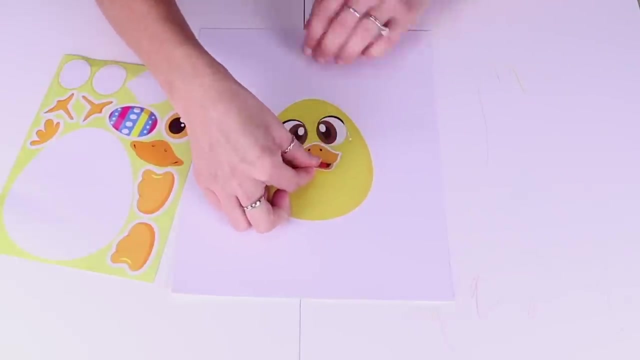 I think I'm going to use these eyes, And our duck has two eyes: One eye and another eye. There we go. Alright, let's see, I think our duck needs a mouth Or a beak. There we go. Oh, he's looking so cute. 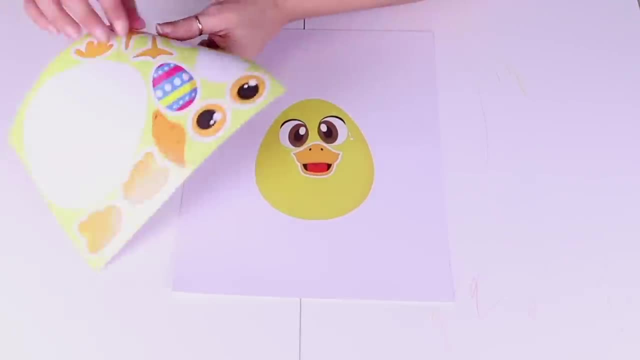 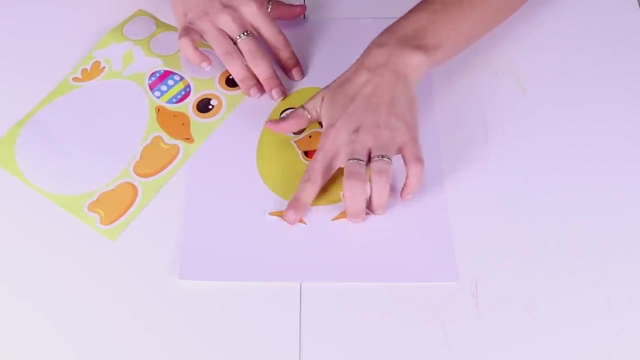 Already. What else does our little duck need? Hmm, I think he needs some feet. Yes, let's put some feet on him So he can waddle around and see his friends. Alright, there we go. Now he's got some feet. 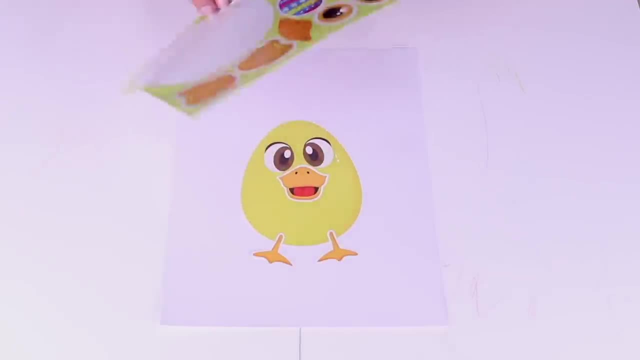 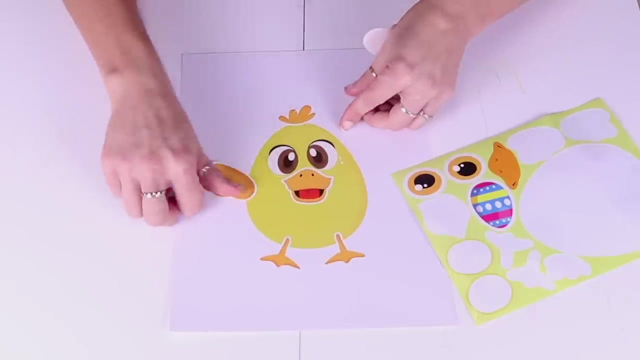 What else? Hmm, let's put some little hair on top of our little duck's head right here. There we go. Okay, um, and I think the last thing is some wings, So our duck can fly. There we go. Look at that. 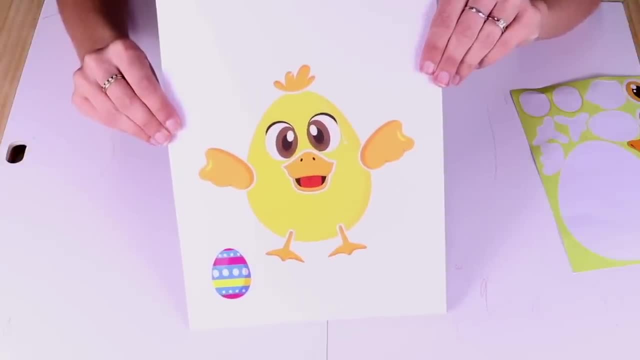 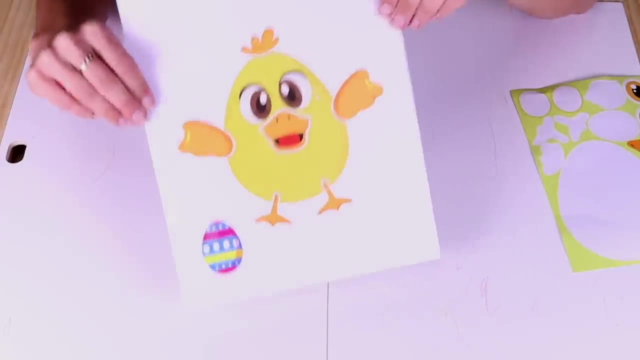 Look at our cute duck. Do you know what a duck says? A duck says quack, quack, quack, quack, quack, quack. What a cute little duck. Quack, quack, quack, quack, quack quack. 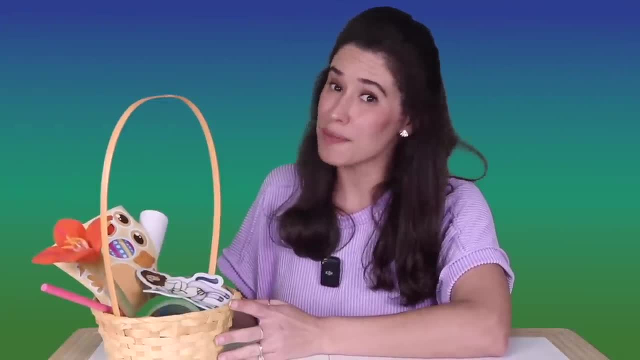 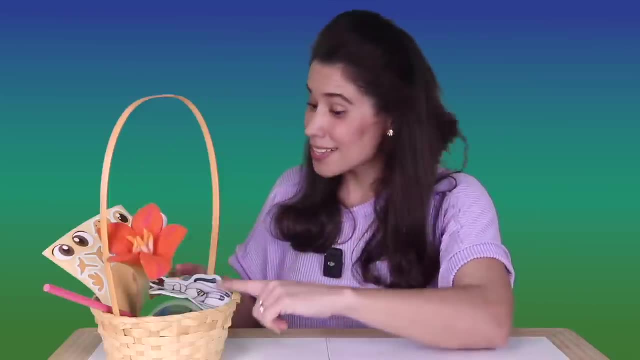 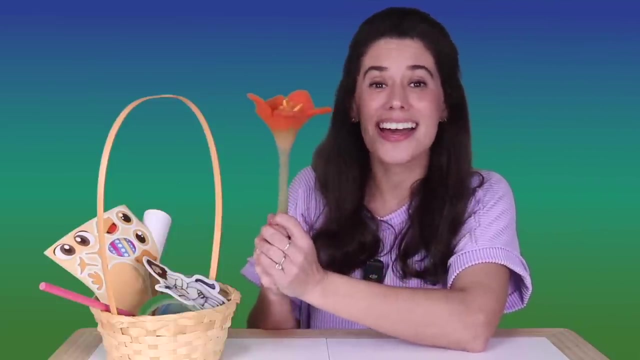 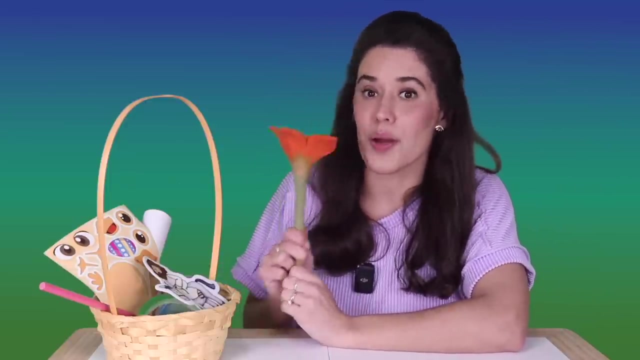 What else do we have in our basket? What's in the basket? What could it be? What's in the basket? Let's look and see. I see a flower, Yes, a beautiful flower. Oh, it smells good too. I wonder what we're going to talk. 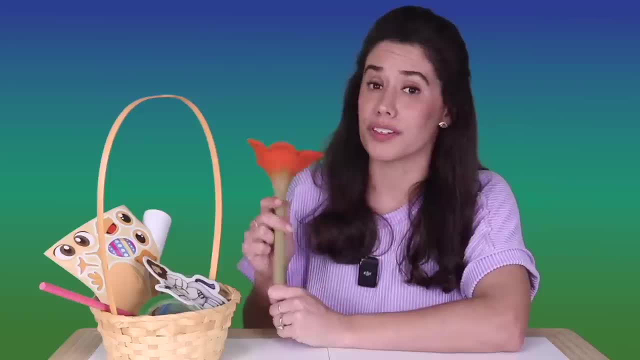 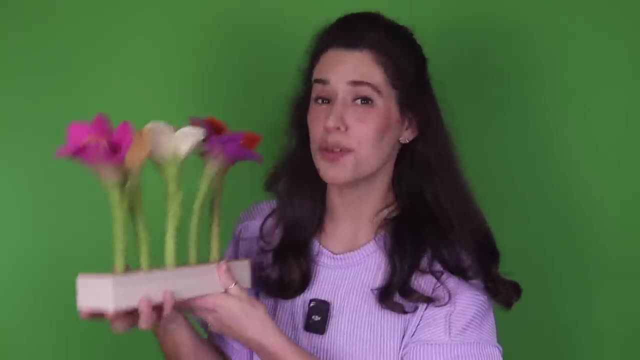 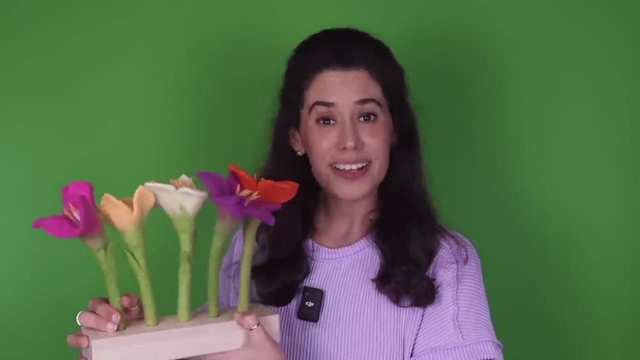 about with our flower. Hmm, maybe we're going to talk about the beautiful flowers that God made. Wow, Look at all these beautiful flowers that God made for us to enjoy, Aren't they beautiful? Flowers bloom in the springtime. Yes, flowers bloom in the. 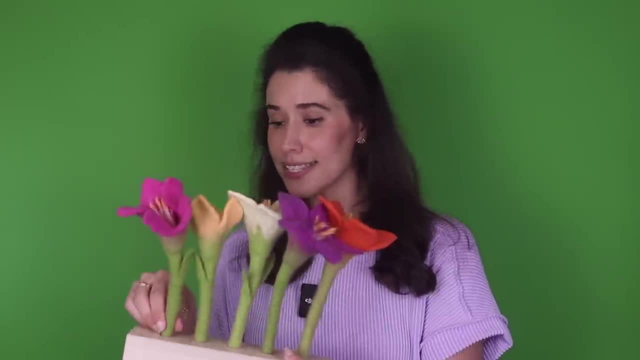 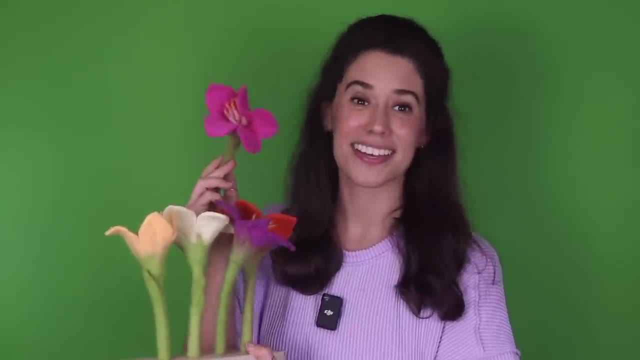 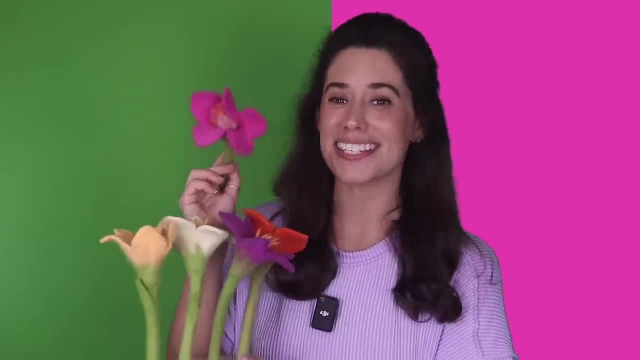 springtime, And what pretty flowers. Let's see What color is this flower. Do you know what color this flower is? Yes, This flower is pink, P-p-pink. This is a pink flower. Pink, Alright. let's see what else. 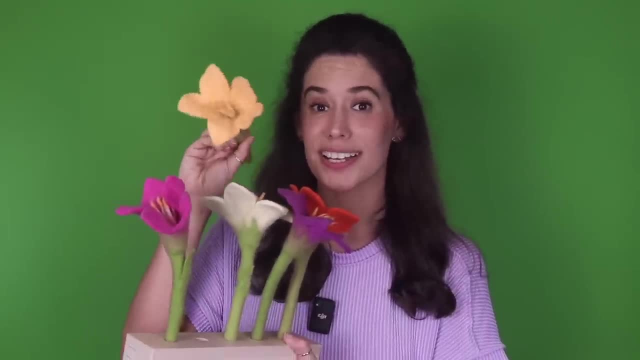 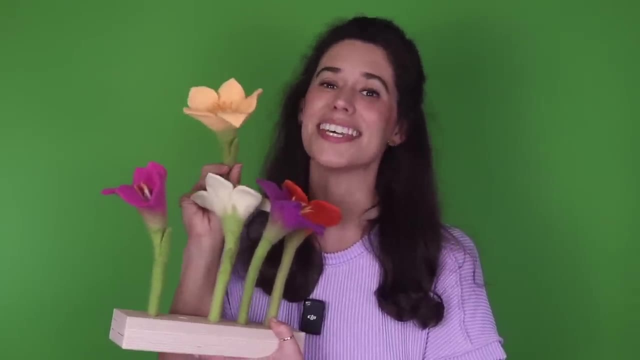 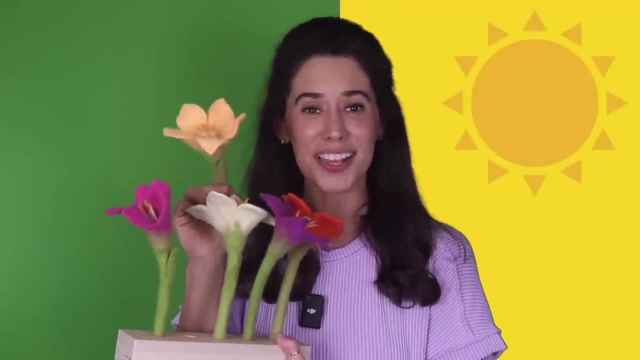 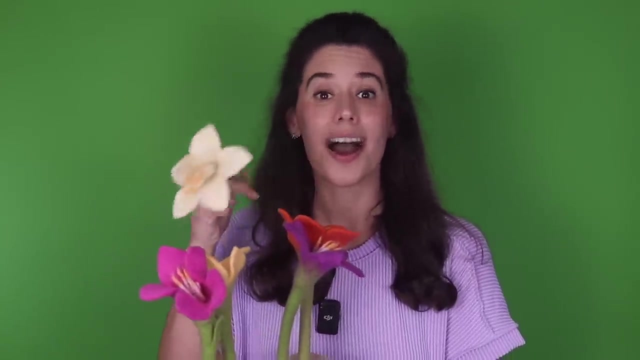 do we have? This is a beautiful flower. It's the same color as the sun. What color is this flower? It's yellow. Yes, a beautiful yellow flower, Y-y-yellow, Yellow. Next we have a white flower. That's right. 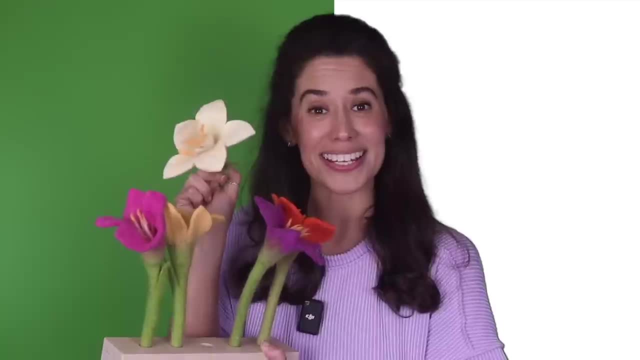 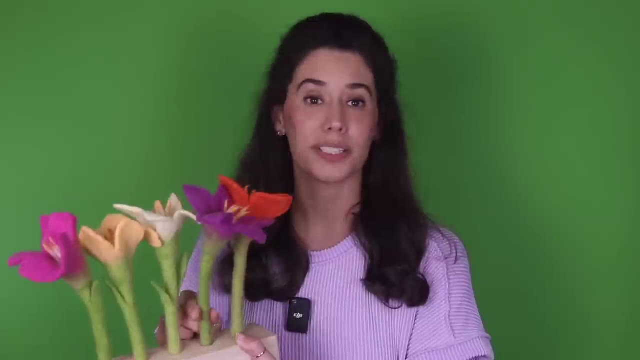 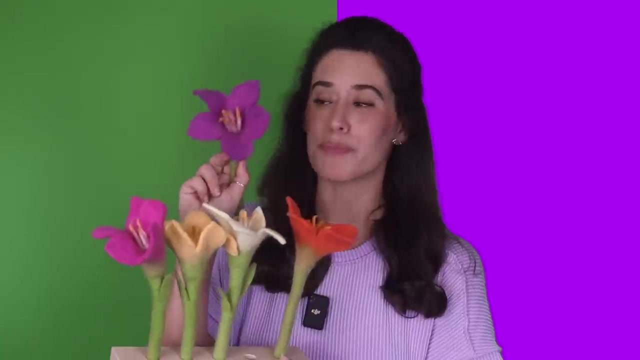 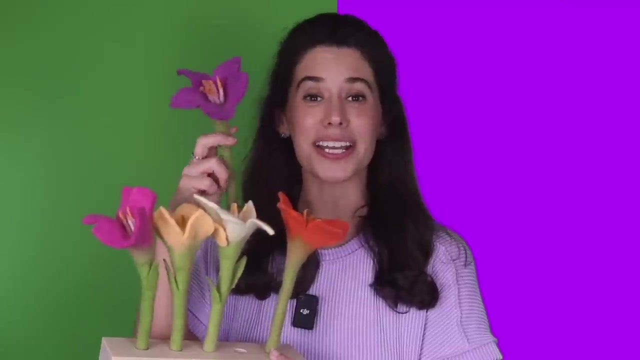 White flower W-w-white. Yes, this flower is white, Alright, what else? We only have two more flowers. This flower is purple, Purple, P-p-purple, What a pretty flower. This flower is purple, Alright, and our last flower. 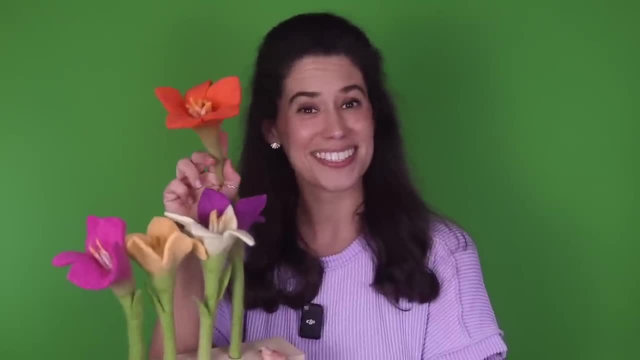 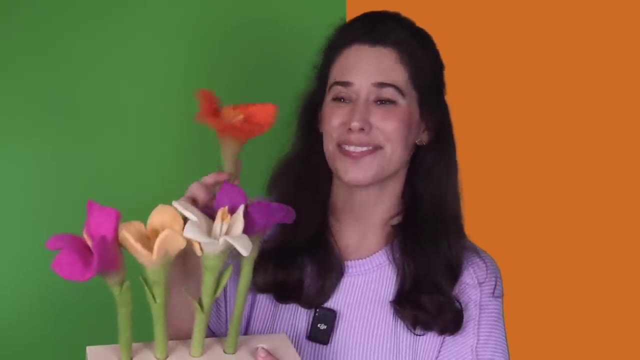 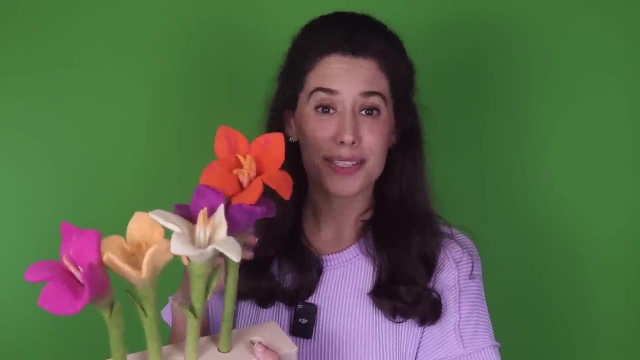 isdo, you know what color this is? Yes, Yes, you're right, It's an orange flower. Yes, this flower is orange. What a beautiful orange flower. Oh, it smells pretty too. Wow, I love flowers. and these are all such pretty flowers. 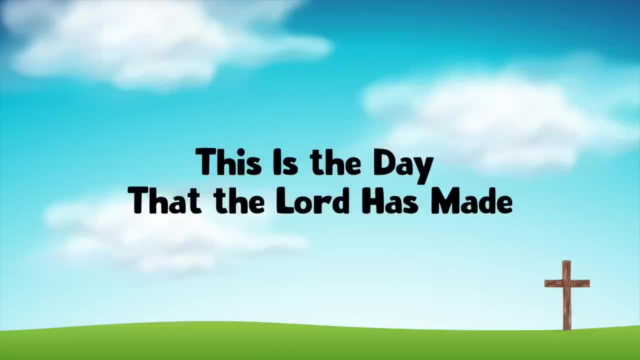 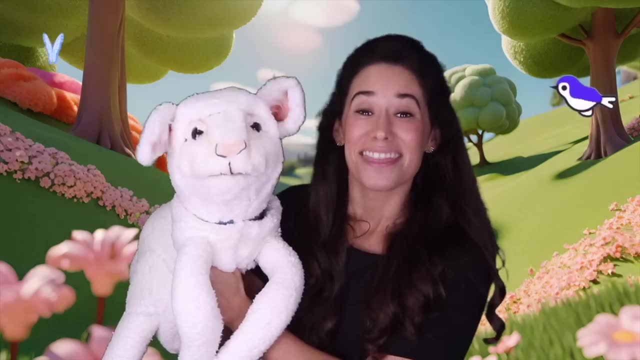 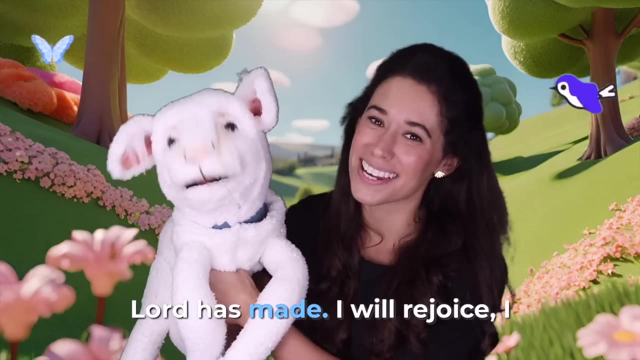 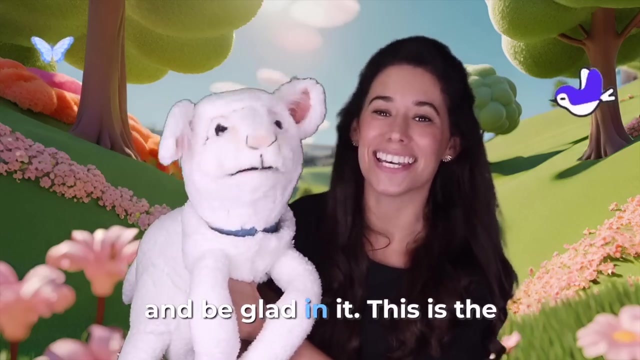 that God made for us to enjoy. So what about our next flower? This is the day. this is the day that the Lord has made, that the Lord has made. I will rejoice, I will rejoice and be glad in it, and be glad in it. This is the day. 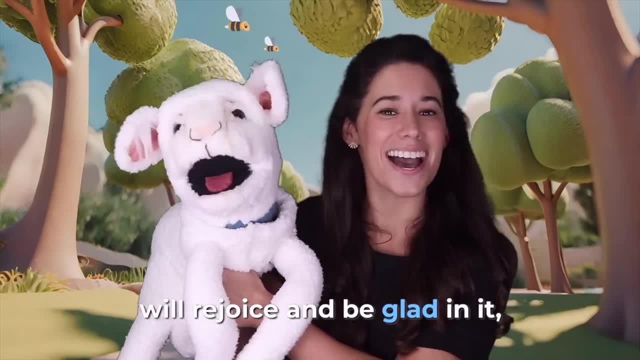 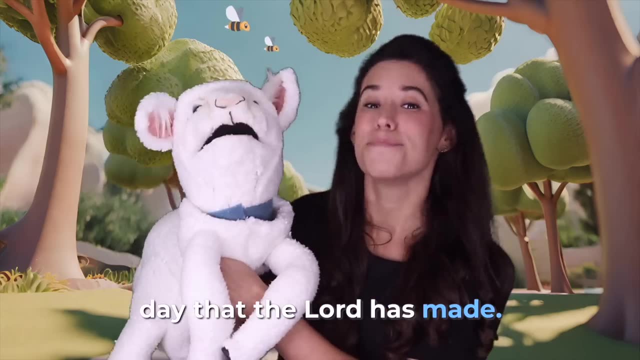 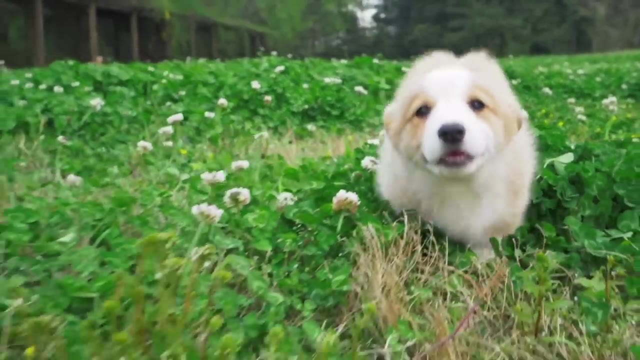 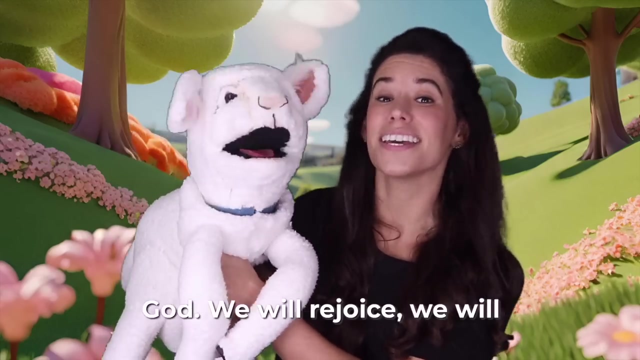 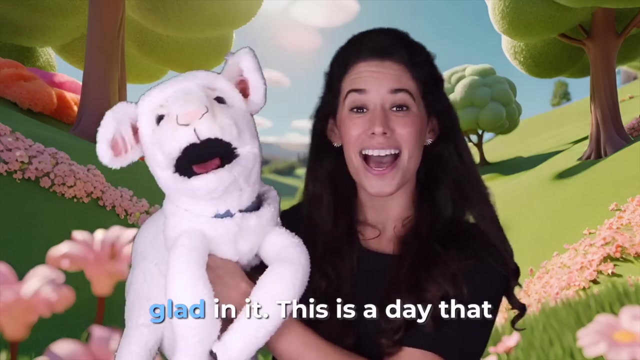 that the Lord has made. I will rejoice and be glad in it. This is the day That the Lord has made. We are the kids. We are the kids Of the living God, Of the living God. We will rejoice. We will rejoice And be glad in it, And be glad in it.